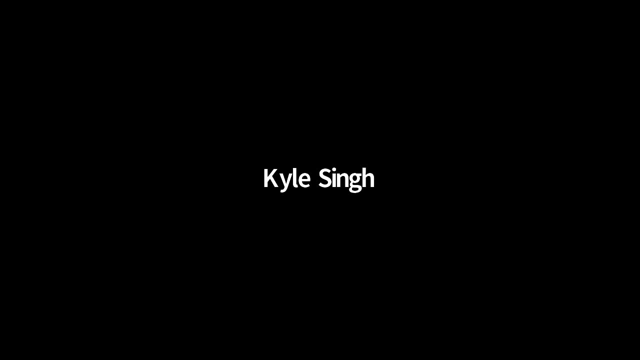 probing quark and gluon dynamics. you guys may have seen in some of our exploration, a lot of that probing happens through the weak interactions. Okay, so this is a good chance for us to sort of peer into this, see how it all works Today. I'm going to sort of just 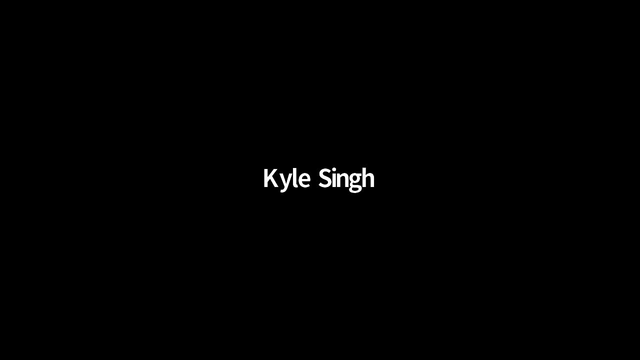 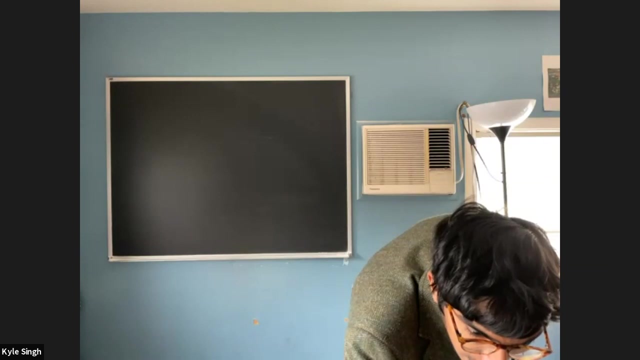 show you the basics of the weak interaction. I'm going to show you the Feynman rules and that kind of thing. I won't derive the Okay yeah, thank you for that. I will pin my No. it says it's pinned. Oh my bad. Oh, spotlight. Oh yeah, Because when I click on the speaker, view: Yes. 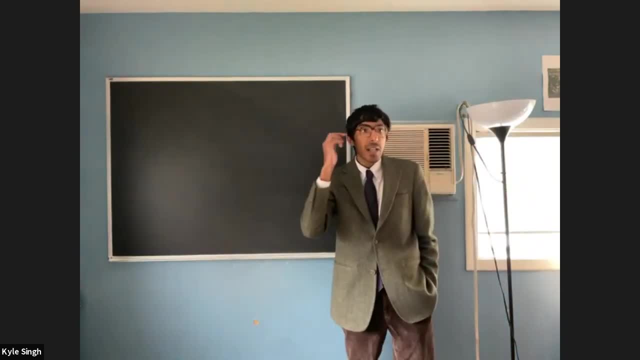 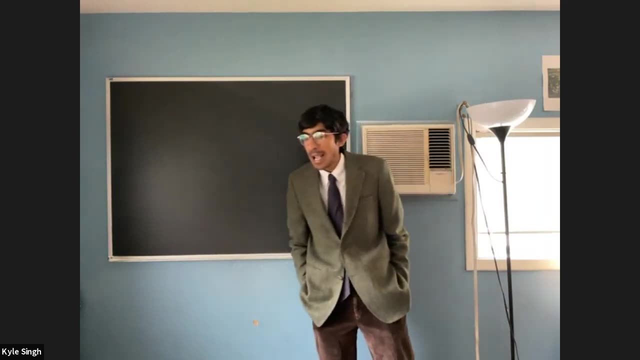 yes, there we go. Now it's good, Yes, good, Okay, so today I'll sort of show you the basics of the weak interaction, the Feynman rules and all of that kind of thing, And next week we will do. 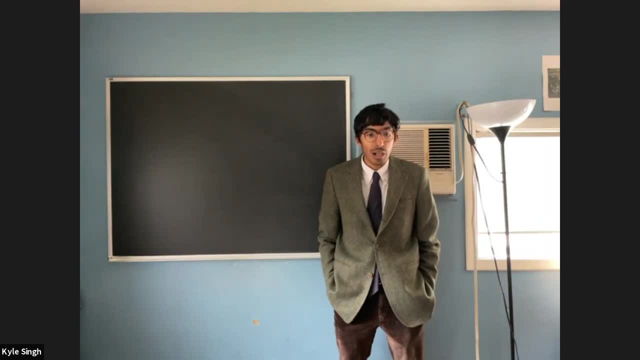 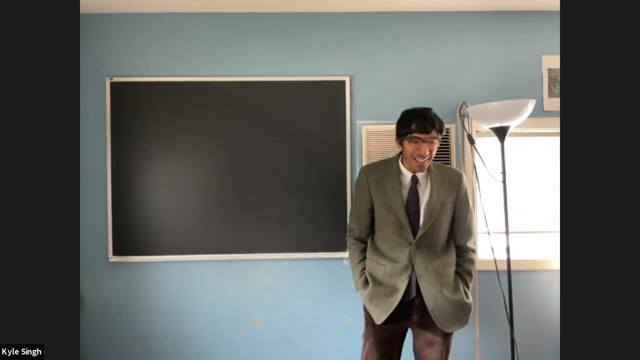 electroweak unification. So that will take us the whole lecture, Electroweak unification being the major achievement of Glashow, Weinberg and Salon- mainly Glashow, But that is a sort of a nice. It's a difficult topic but it's a good topic to look at. But we'll try. I'll try to. 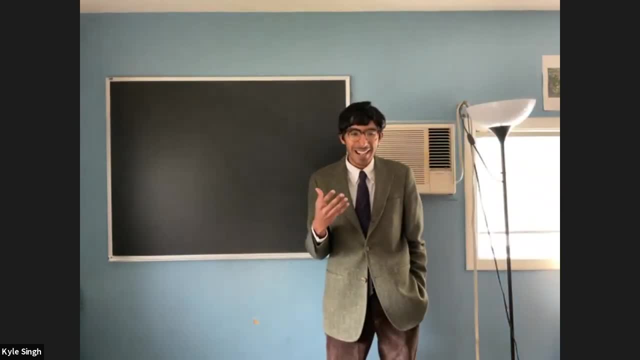 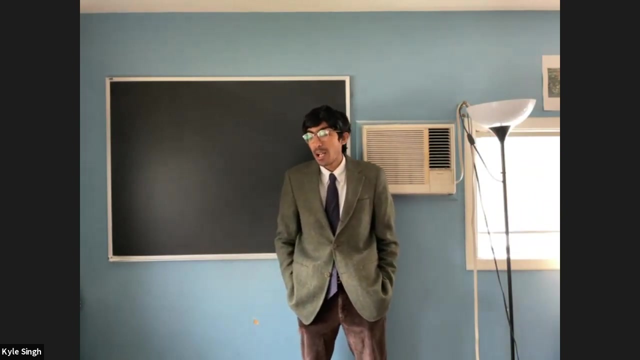 simplify it as much as possible, But it's a challenging topic But we'll look at it, since it's such a big achievement of 20th century physics. And if you want to look that up, that's called the GSW model. People usually write it Or G. I don't know something like that. If 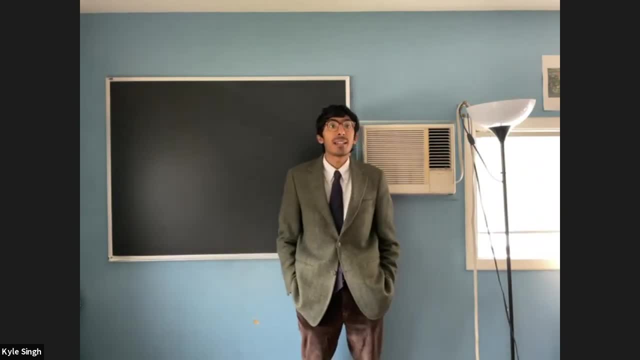 you just look up electroweak unification, which showed that the electromagnetic forces really are derived from weak interactions, that there's a unified underlined structure to that, which was quite a big achievement. Okay, let's get, Let's get started on that. then The homework. So there's a couple, There's quite a little bit of 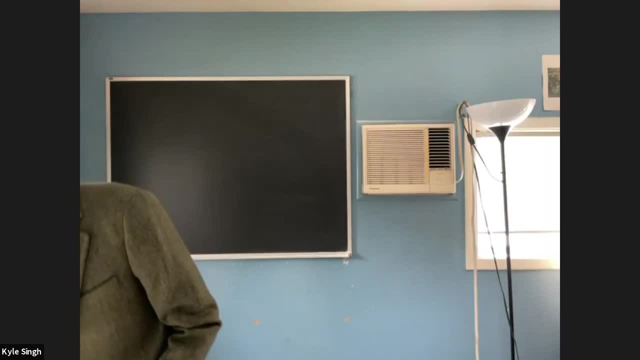 papers I want you to look at. So the first thing is LB, chapter 47.. Okay, And this is in addition, because there was two weeks of reading in the document, right, So you know, get that done too. And then there's two papers. I want you to look at The first paper. 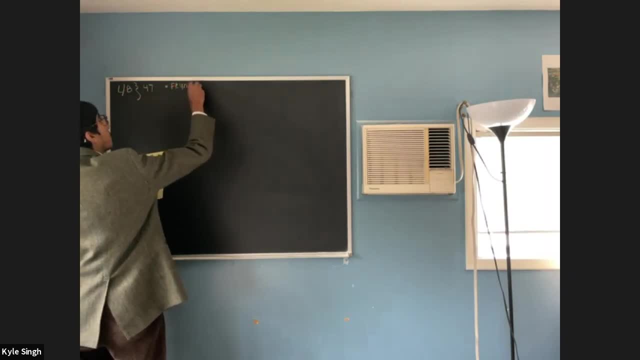 is by Feynman and Gelman. So these are sort of two. If you can't get these, let me know. I'll send you PDFs. Okay, Because I know what the access sometimes right, It's Okay, And this: 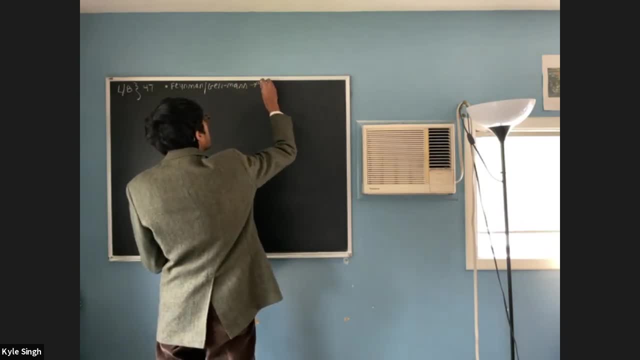 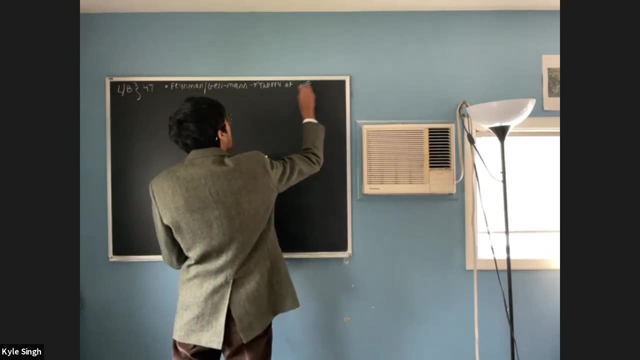 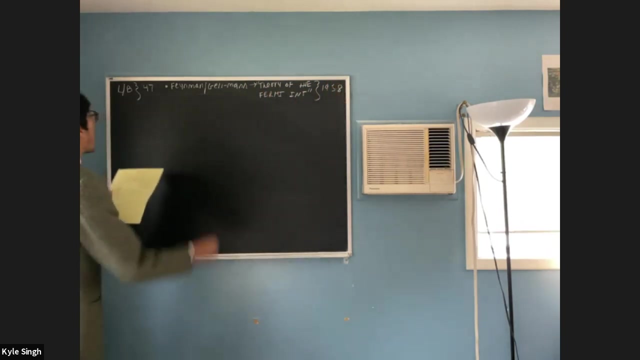 is called Theory of the Fermi Interaction And you'll see why it's called this. This was written in 1958.. And the second paper, And actually these two guys won the Nobel Prize for this. So TD Lee and CN Yang, who you know, Yang from Yang-Mills Theory, 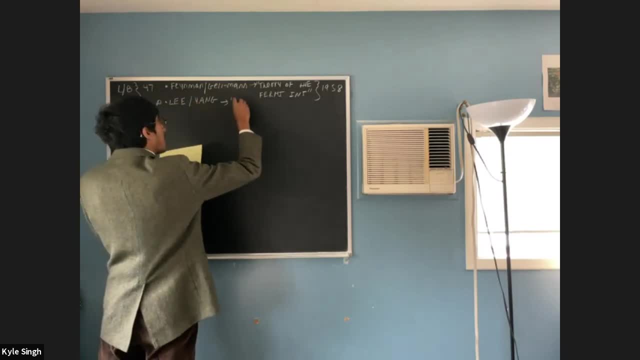 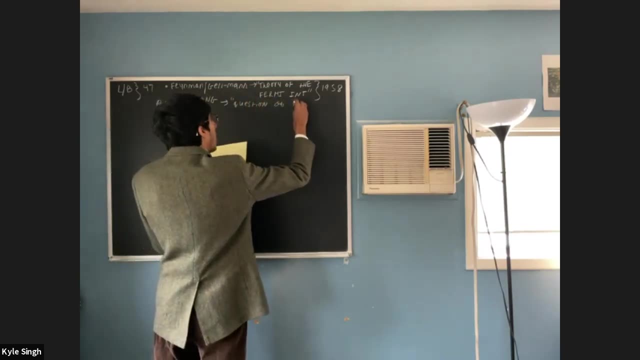 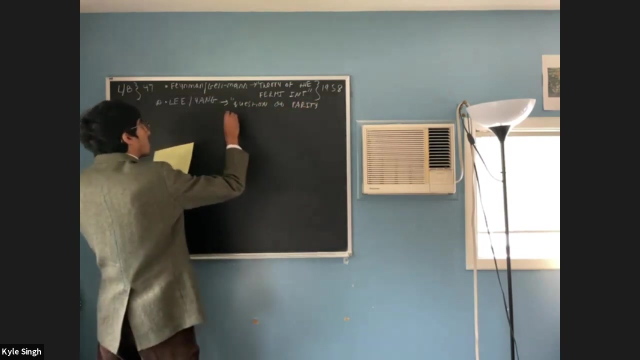 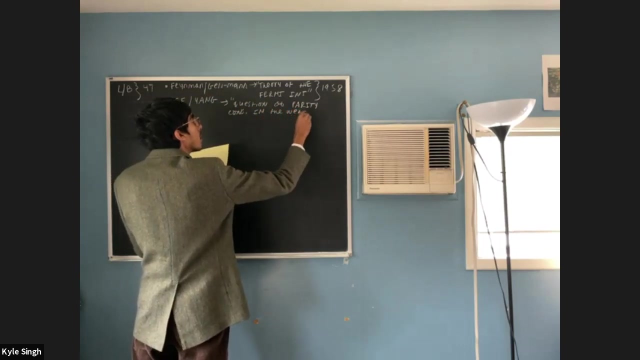 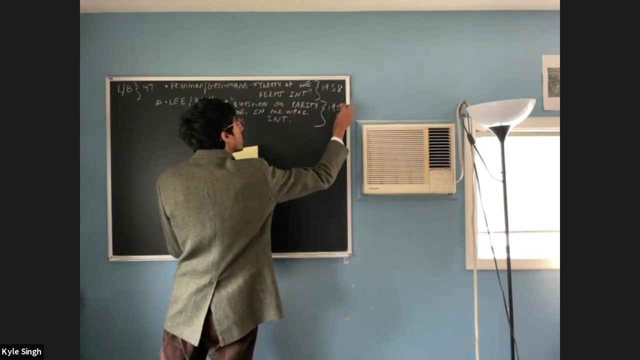 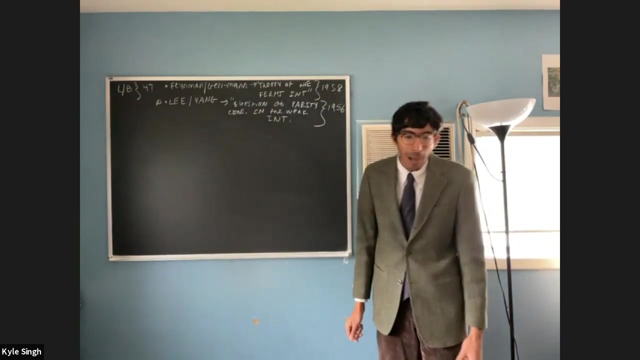 And they won the Nobel Prize And it's called Question and Answer. And it's called Question and Answer of parity conservation in the weak interaction. so parity conservation. this was written in 1956. these are two very iconic papers. there's like those classic Gelman and Lowe's papers. 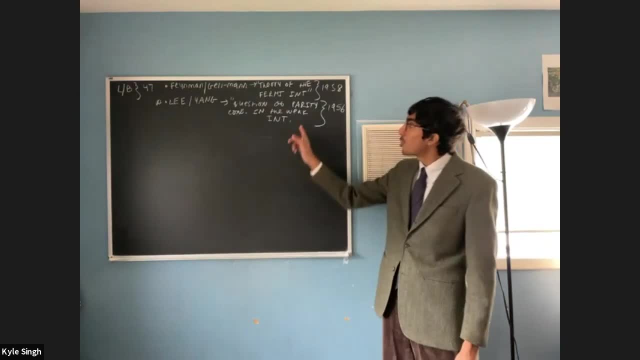 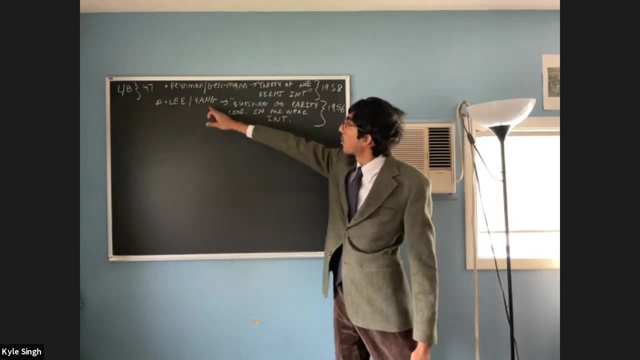 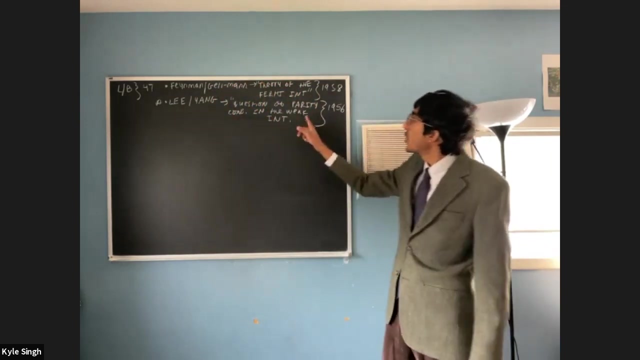 there's many classic papers in QFT. these two are very classic papers and they have thousands of citations and obviously Feynman and Gelman- all Nobel Prize winners. Gelman worked a lot on QCD. we know Feynman and Lieny. this paper is extremely famous. 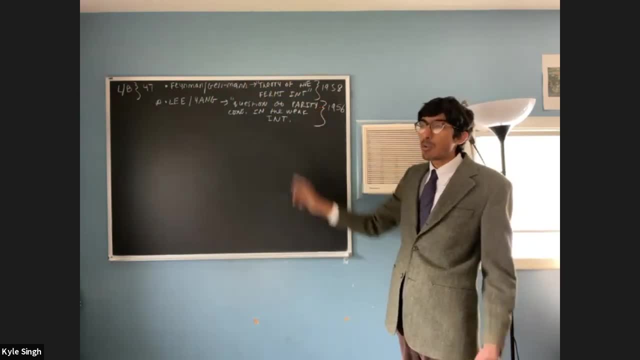 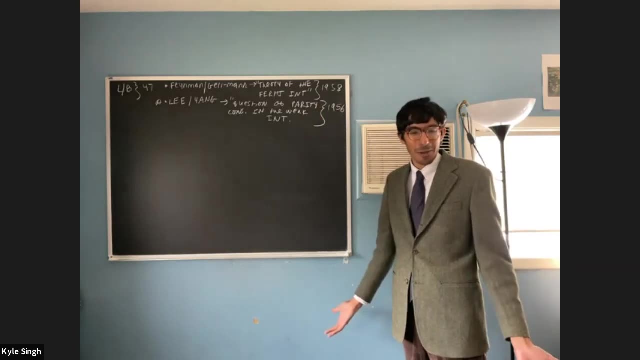 because this proved, not proved, but it sort of. there was an experimenter who proved that parity was violated by the weak interaction and she was a woman, and she did not win the Nobel Prize with Lieny, which is ridiculous. everyone thinks she should have won it. 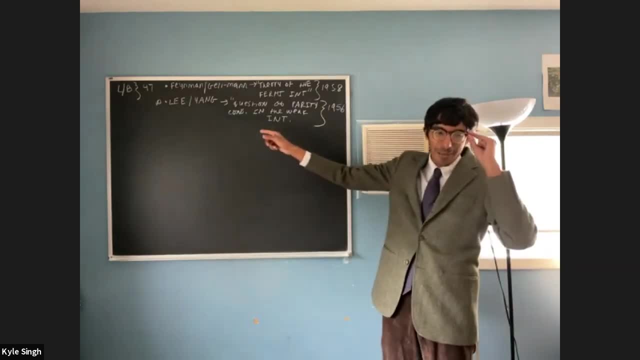 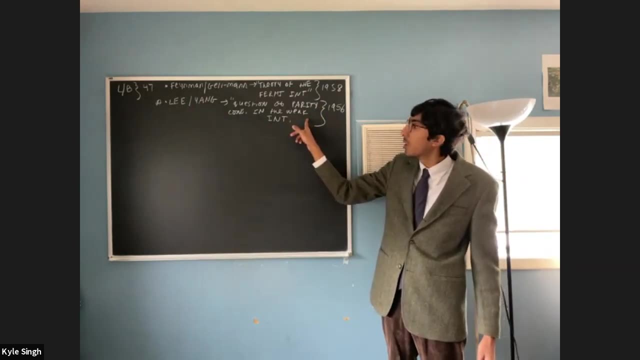 they only gave it to Lieny, which is crazy, but anyways. so this paper was the first theoretical paper that sort of postulated the idea of parity violation, which we know is violated by the weak interaction and this paper. you'll see where this paper comes from. 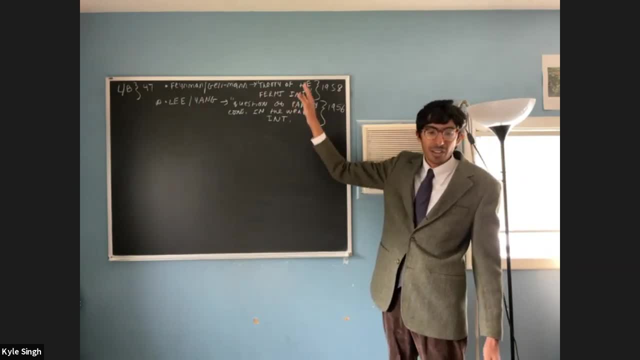 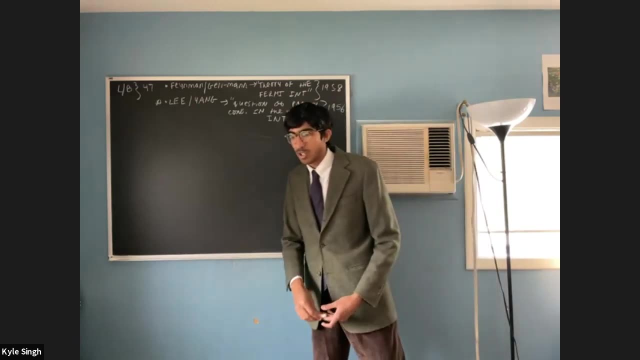 the basic idea of today, but please read these because they're very, they're very. it's very good to see the historical papers. I like assigning them. okay, let's get started. so do you got, do you know, the mediating particles of the weak interaction? what are the mediating? 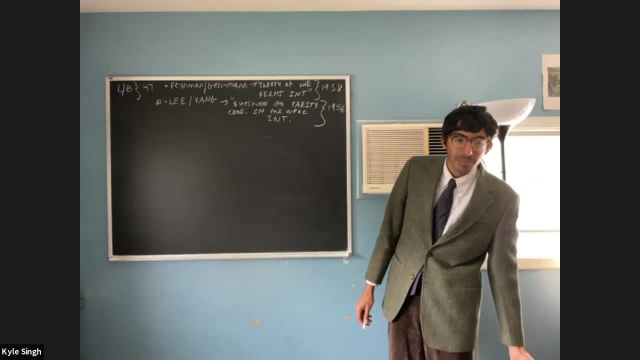 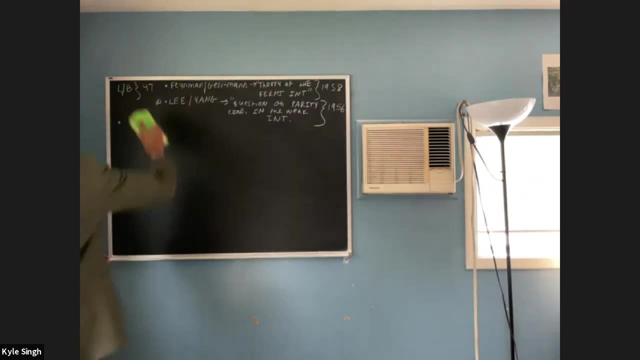 what are the force mediating particles? the W and Z bosons, exactly so, the mediating particles. so I'll erase this actually of the weak interaction, so that that will be our place to start, and it's actually the major difference. you'll see why it's called the weak interaction. 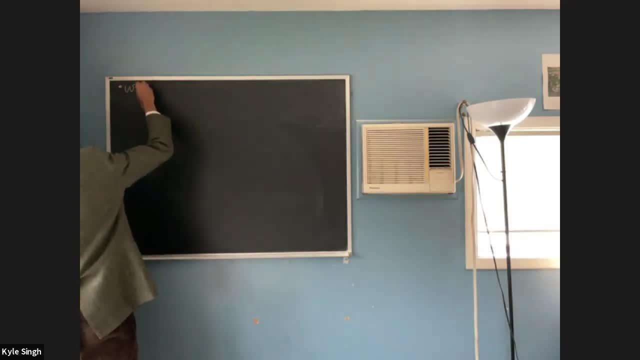 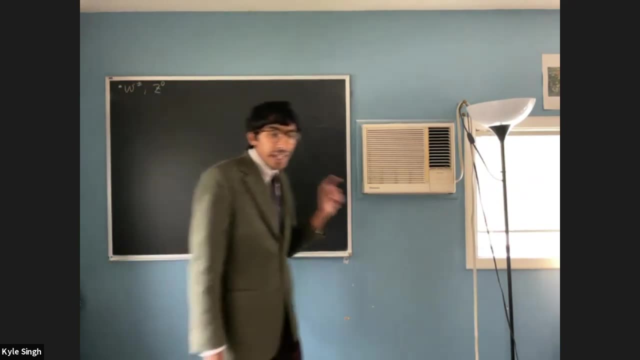 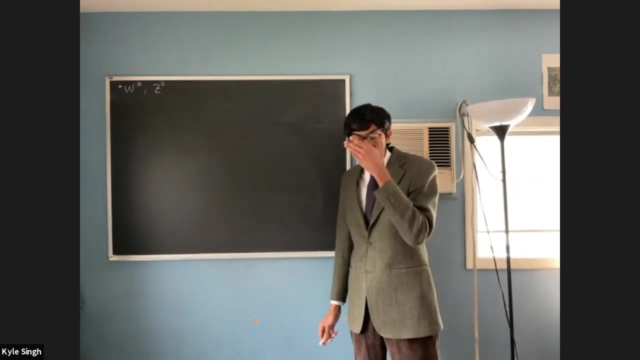 but the major difference is the W and Z bosons. so W plus or minus, and then the Z boson is a neutral boson. the key to the weak interaction is that these guys are massive. right, we know that the mediating particles in in the strong force. 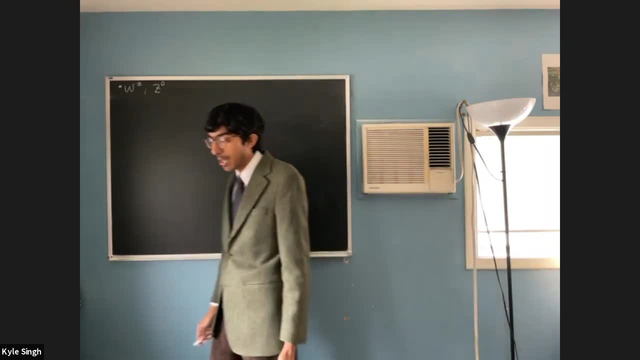 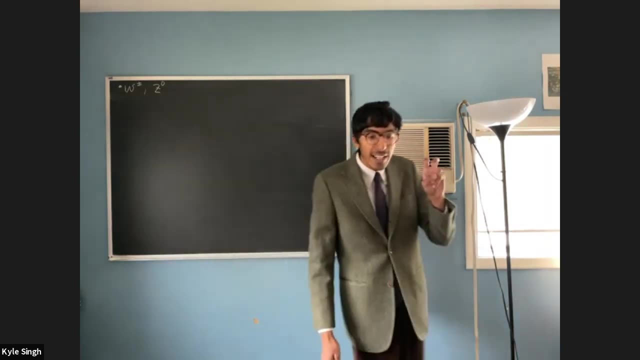 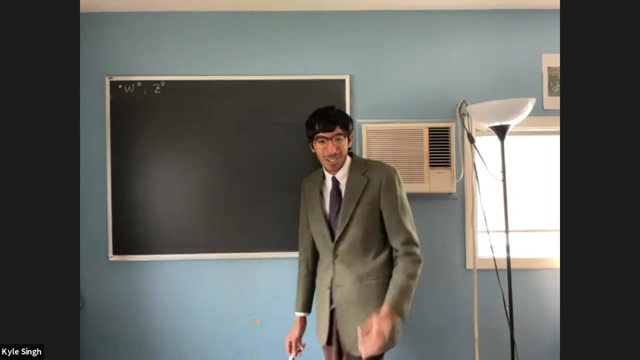 the gluons, the meeting particles in QED, the photon photons, are massless, right, and so that is the major. that's why this is called the weak interaction, quote unquote, because actually the meeting particles are massive, and actually pretty massive by the kinds of scales that we are talking about. 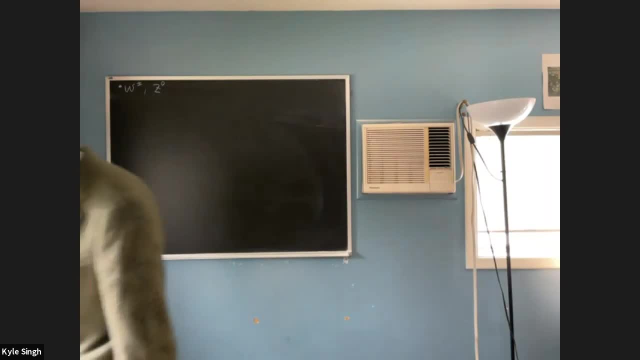 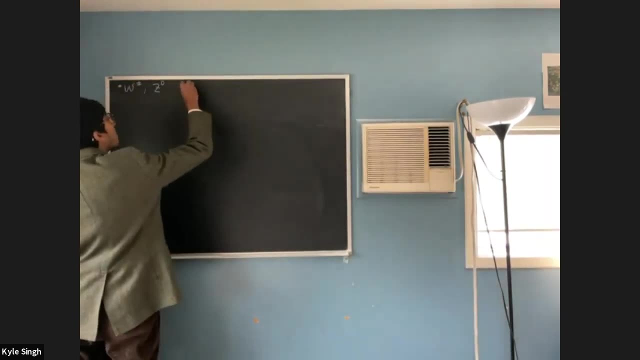 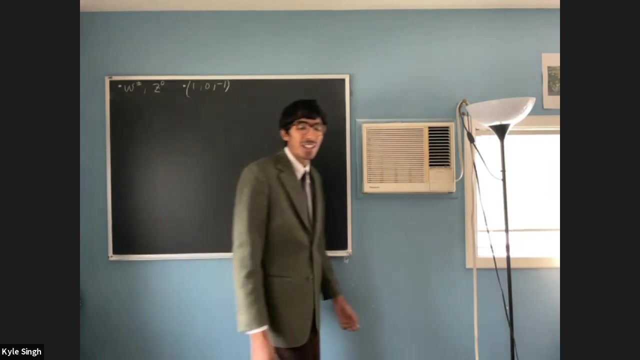 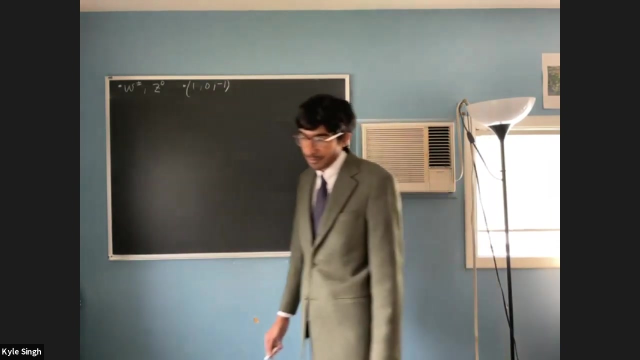 okay, so there are massive spin one particle right, and they have three allowed polarizations. so any massive spin one particle has three allowed polarizations, one zero and minus one. how many allowed polarizations does a photon have? a massless spin one particle, two right, exactly, exactly. 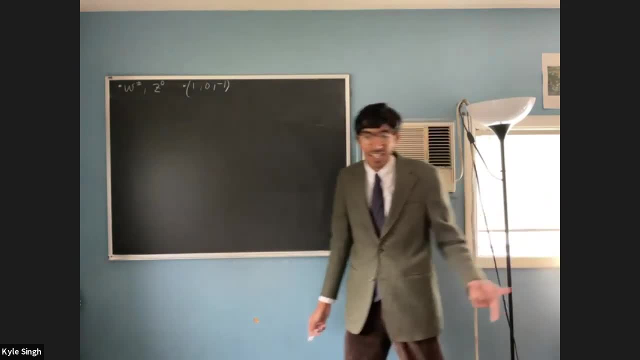 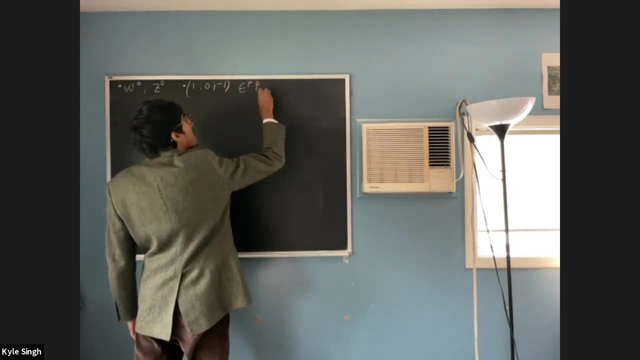 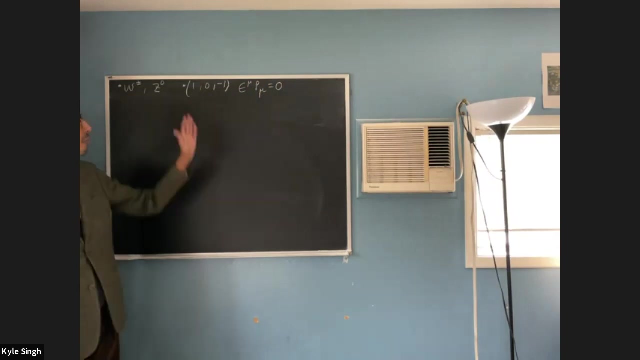 so there's one extra degree of freedom we have to just take into account. so let's work that out. so remember, the first condition we put on the photons for the polarization was that epsilon, mu, p, mu equals zero. all right was the very first condition, and that reduced the number of degrees of freedom from four to three. 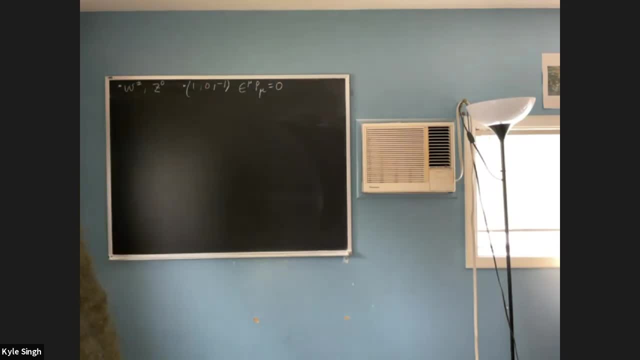 just by imposing this condition. okay, then, in the case of photons, we also impose coulomb gauge. so coulomb gauge was: epsilon zero equals zero. that's just the condition for coulomb gauge and the fact that epsilon dot p equals zero, and this reduced the number of degrees of freedom, for 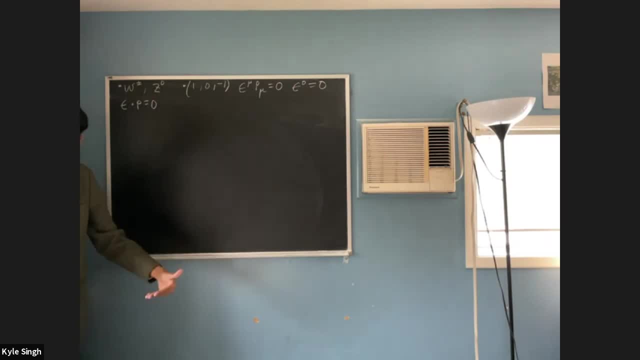 epsilon mu from uh three to two or four to two. so we imposed coulomb gauge for the photon, but this condition is enough for the w and z bosons because they have three possible helicities. okay, so that's the basic pure. you want to call it a gauge condition or whatever, so okay, let's write down the propagator. so 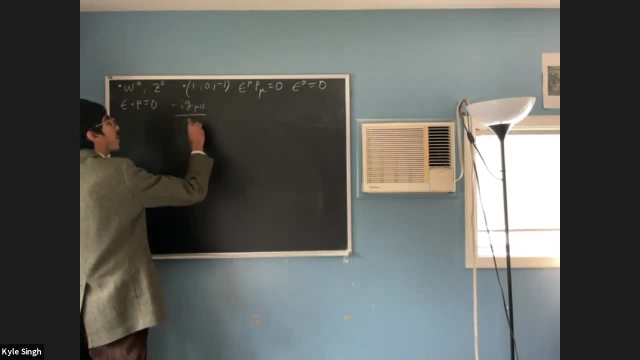 remember in qed the propagator went minus. i g mu nu over q, squared right where q is just the internal momenta, all right, that was the base. where g mu nu is the minkowski metric- sorry, i use g and eta kind of hand in hand. and if you wanted to work out the s matrix you would find. 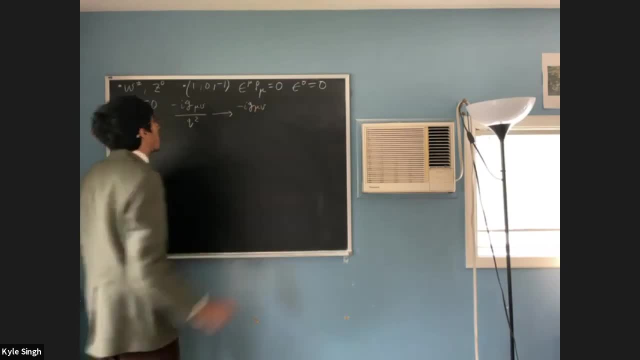 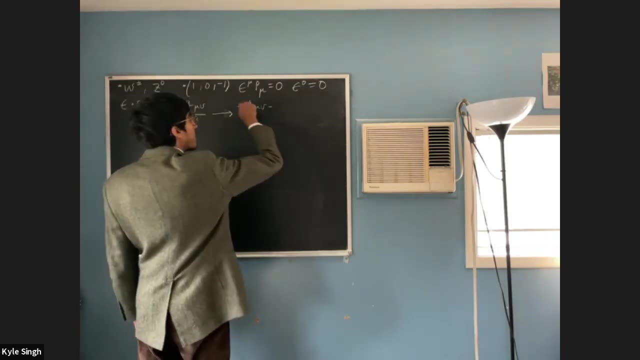 that in, uh, the weak interaction, you get a propagator: minus i g mu, nu, minus i times g mu nu. minus g mu g nu over m squared. okay, so we get a little bit of a different numerator over the standard sort of pole q squared now, minus m squared right here i also have 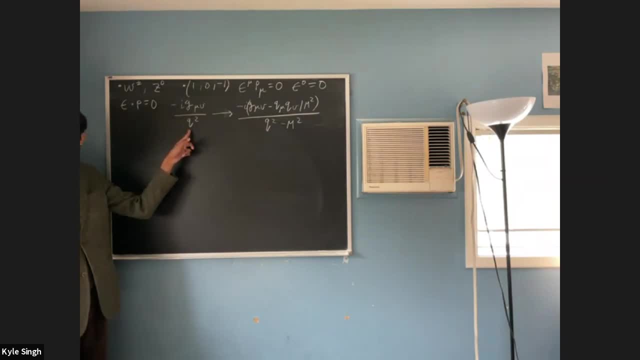 q squared minus m squared. but since the photon is massless, the m doesn't, you know, make a difference. so this is the w and z propagator. uh, now, we often work in a very uh nice limit for the weak interaction, where q squared is much less than m squared, because the it, because these bosons are so massive. 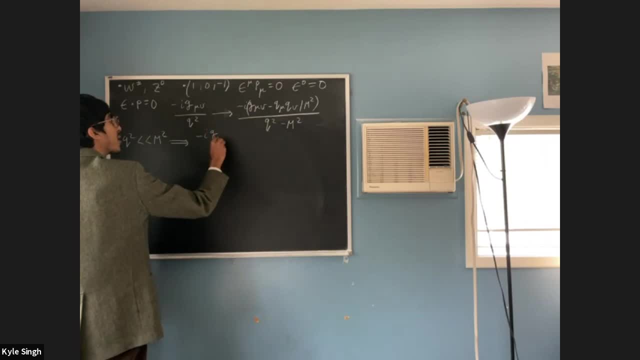 and so really we often just write the propagator as minus i g mu u uh. minus, uh. sorry, then we don't even need that term and we can just keep this bottom term. that's really what we usually write the propagator as minus i g mu nu. 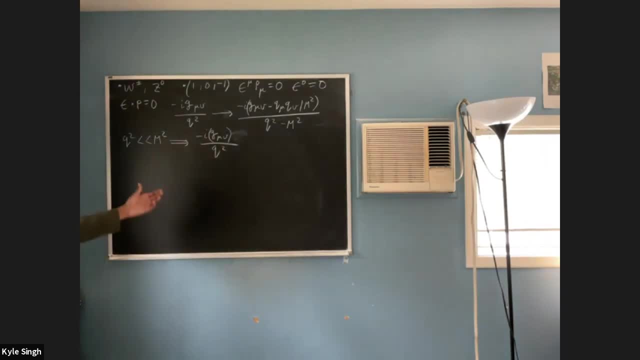 oh sorry, not q squared, m squared right, right, not q squared. so that's usually what i'll write the propagator as, just because we can usually just keep this limit, because the w and z bosons are massive. okay, so let's write down a vertex factor, right? that's sort of the next step that we usually do this kind of thing. so we have some. 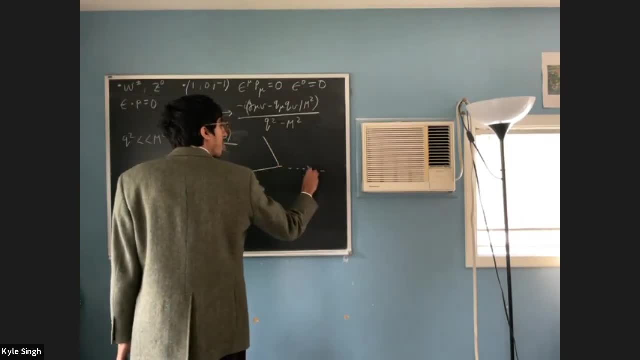 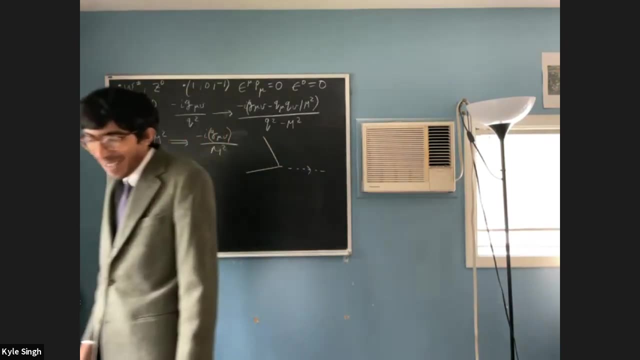 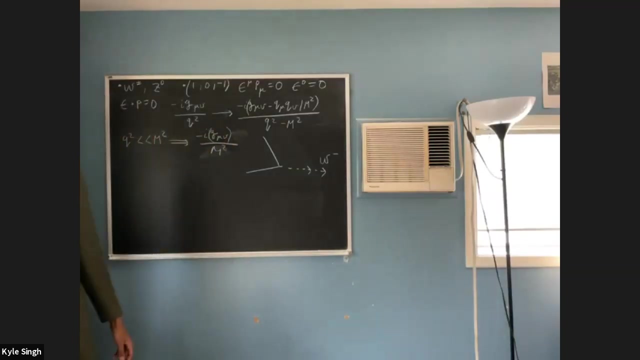 we'll use dashed lines for the w and z bosons, right. we have like curly lines for the gluon and then like a wavy line for the photon. so the last line left is a dead and we'll call this a w minus. let's look at interactions with the w minus first. 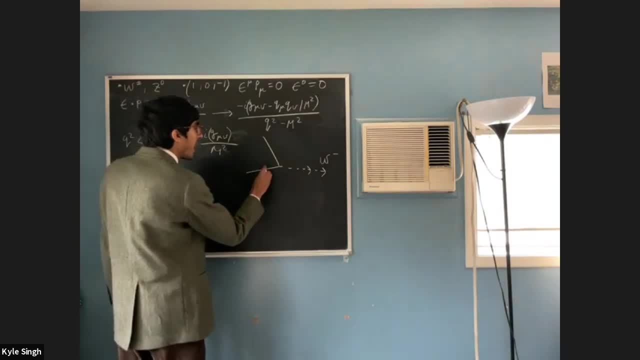 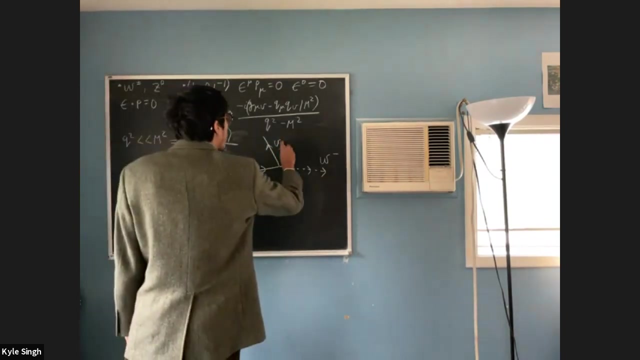 and let's say we have some lepton, call it l minus. could be any kind of a meson or an electron, and it's and it gives off some neutrino. so that's the thing. that's one of the most common weeks, so we'll call this. 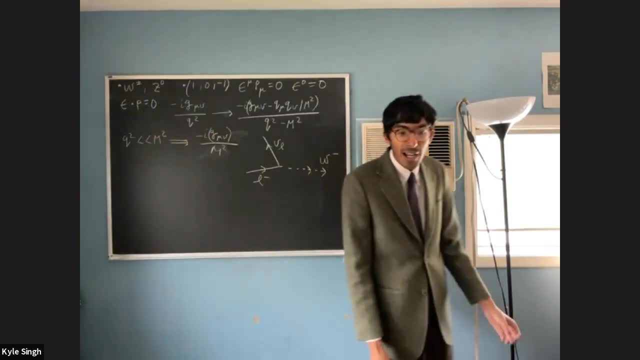 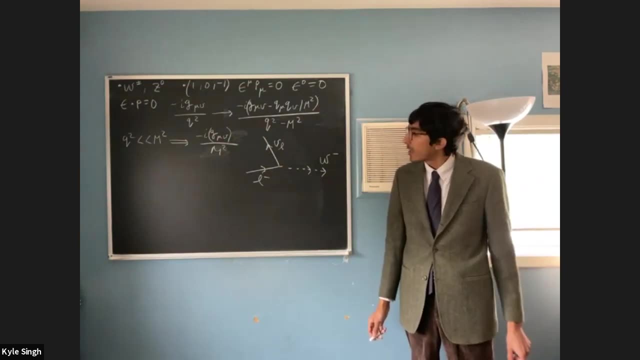 the neutrino. so remember the one of the most common interactions- that's a weak interaction- is a particle giving off a neutrino. okay, that is the most common weak interaction and to each lepton, each lepton gets assigned a neutrino. so the muon gets a muon nutrient you may have. 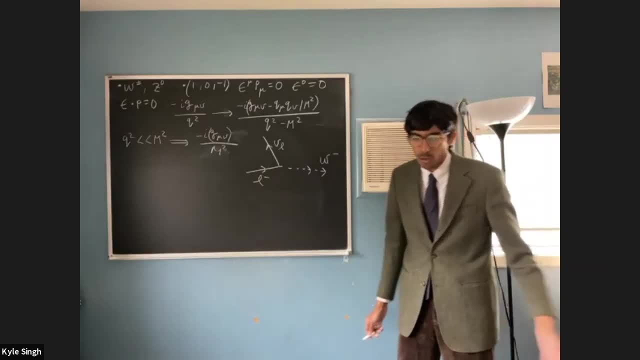 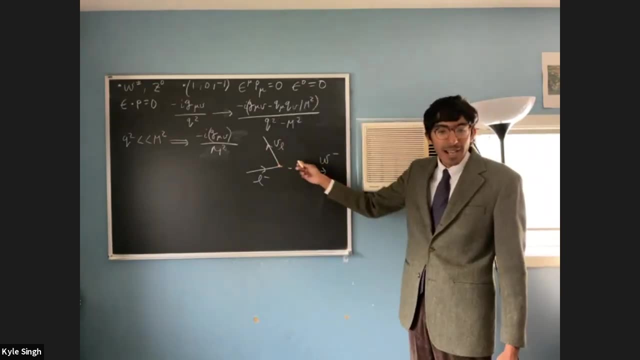 heard of this right when you see the standard model, the tau gets a tau neutrino. so this is the most common sort of interaction- quote unquote- we can have, and we'll have some vertex factor right for the mediating particle. so let's write down that vertex factor. 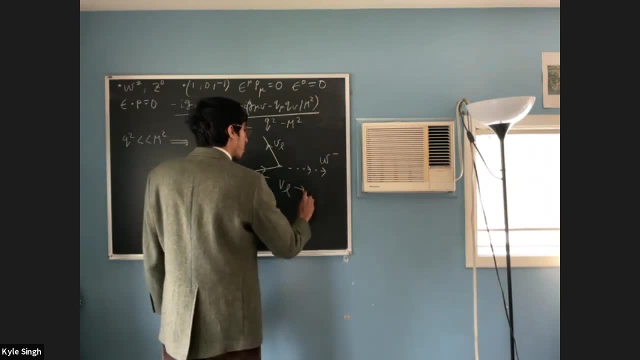 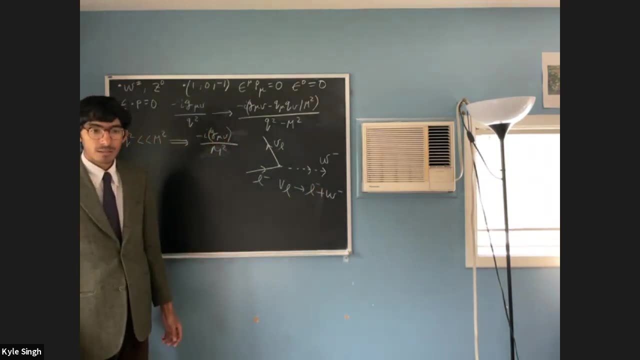 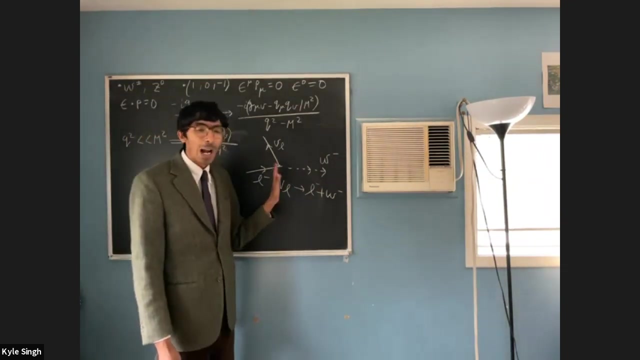 so this is just what this is just lepton neutrino to lepton plus w minus. that's what this is. and remember, we could also have a variety of different reactions. right, we could have an anti-lepton and the anti-neutrino. we could have all kinds of crossed reactions with crossing. 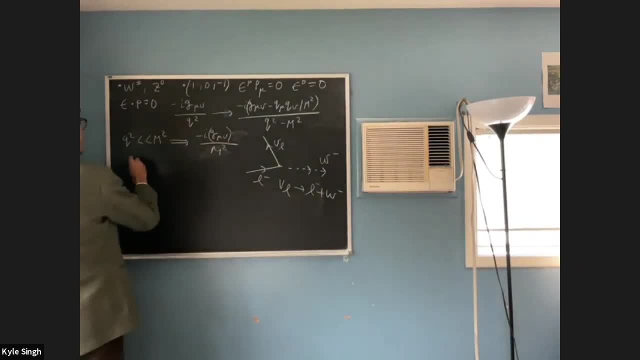 symmetry exchanging the sun. so here's the vertex factor. now the. the vertex factor for the weak interaction is what is so weird? so you have minus i, g w, where g w is what i'm going to call the weak coupling. okay, could i mean? that's just my 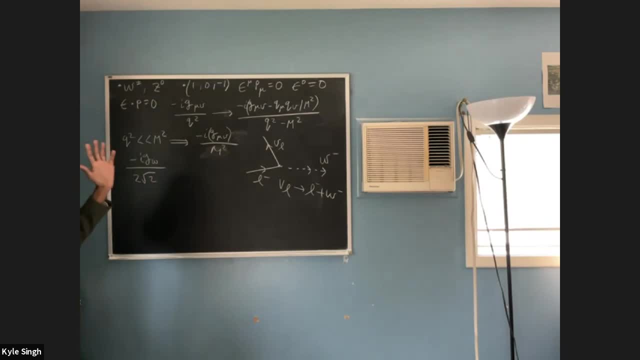 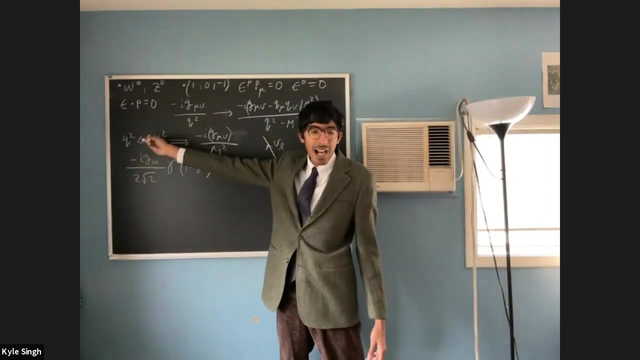 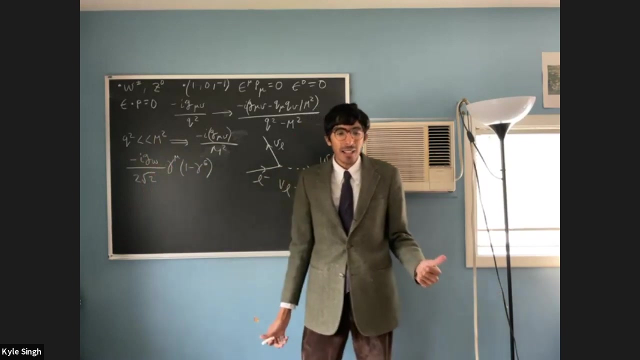 convention. these two root twos are convention times. gamma mu one minus gamma five. okay, so that is, that is the vertex factor, and so this stuff is fine. this, this, this guy, is just basically what we keep seeing popping up with vertex factors. right, gamma mu is fine. that tells me that the coupling's a 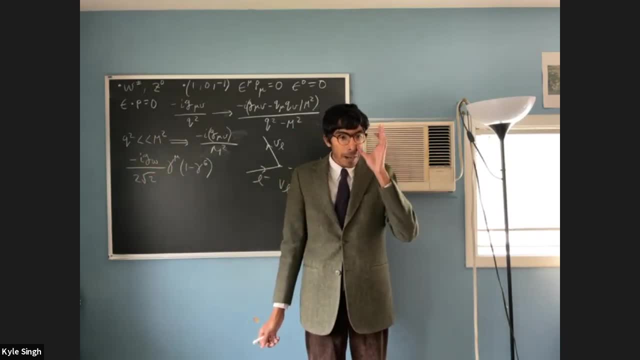 vector coupling, because in qed, remember, the coupling was gamma, it included a gamma mu, d mu. now, this guy's what's weird? this one minus gamma phi, and actually what you'll see is that this, first of all, this one minus gamma five, this combination of gamma matrices, gamma mu, gamma phi. 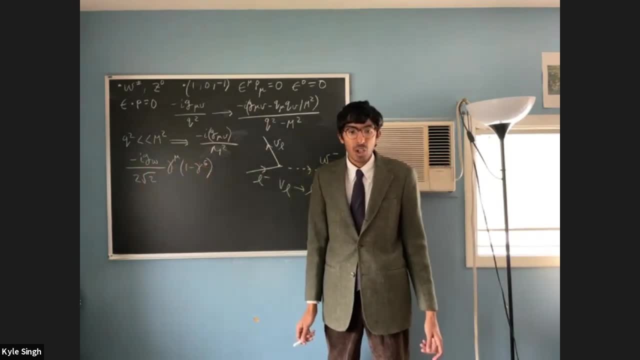 is what we call an axial vector coupling. okay, and the reason that historically, people didn't realize, didn't couldn't figure out whether it needed to be an axial vector coupling. they realized to be an axial vector coupling to account for parity violation, which will show And actually 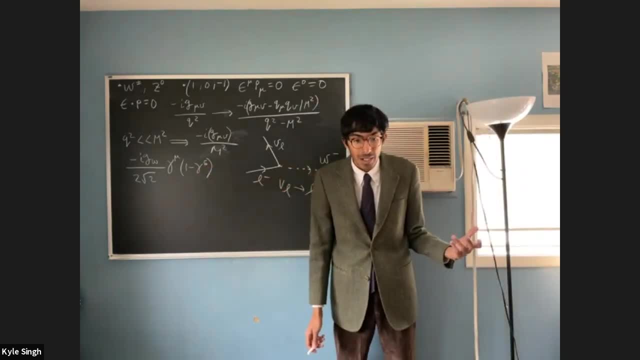 that's what that paper by Gelman and Feynman is about. So Feynman and Gelman were the first guys to say, look, we probably need an axial vector coupling to describe the weak interaction. So that's where this originates from. So if you look at that paper, they actually write this coupling. 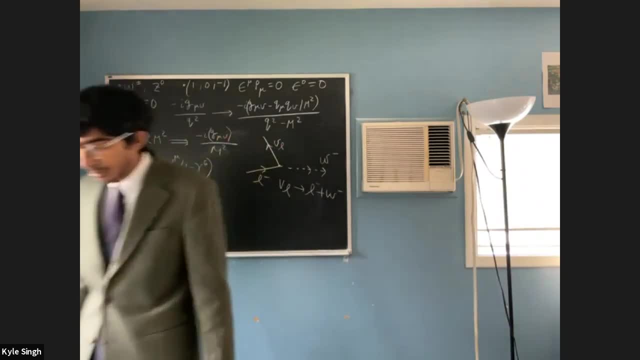 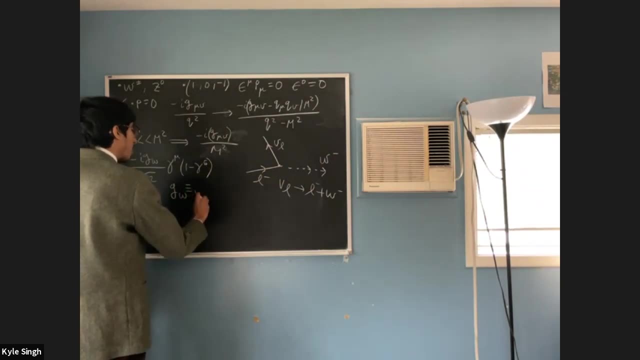 for the first time and play out the consequences. OK, it turns out that the coupling goes like 4 pi times alpha w, where alpha is just the fine structure constant, So I forget what it's like 1 over 137.. OK, cool Shall we compute an amplitude. 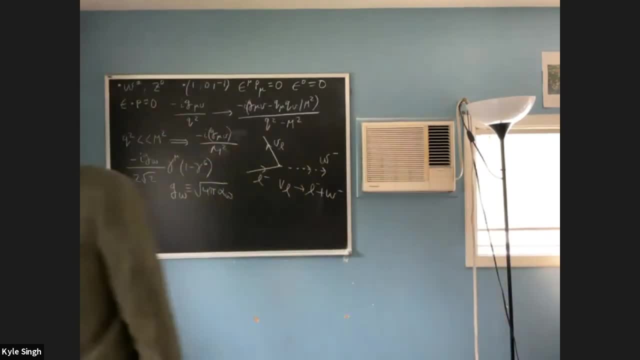 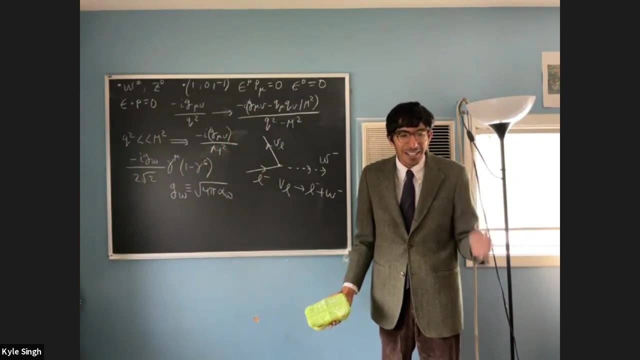 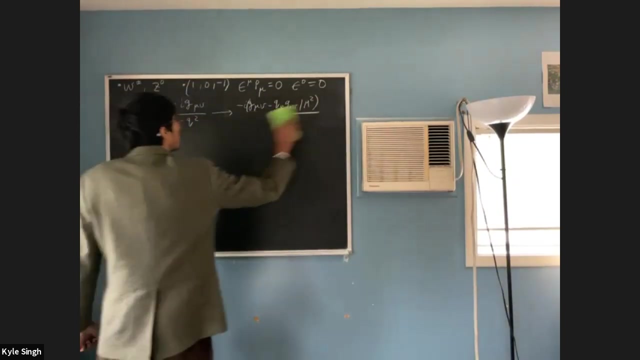 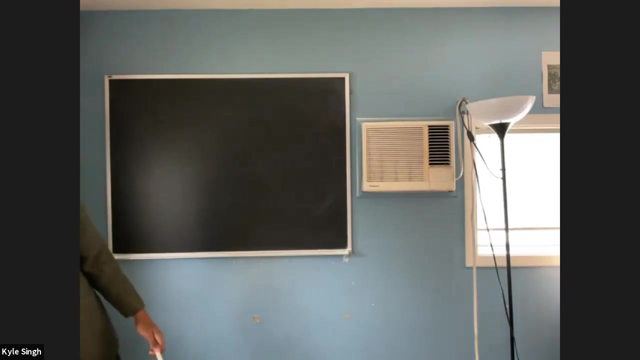 I think that's probably the next step. OK, let's do an amplitude. I'm only going to work out one amplitude in total today. The rest I'm just going to write down the cross-section, So I'll do one amplitude. I mean, it's really not that different, right? It's really not that different, It's all. 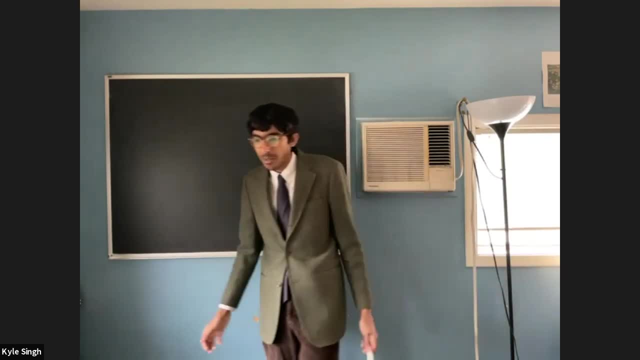 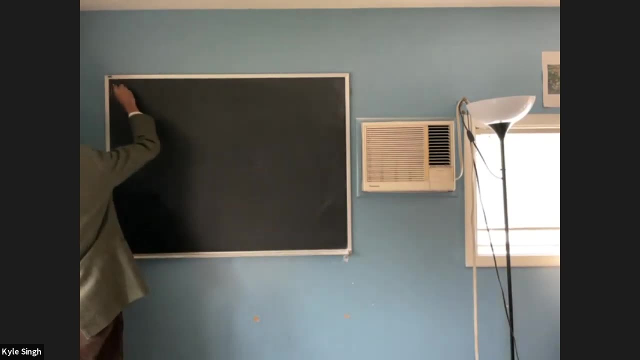 the same fine rules, and it's just the basic thing. But let's do one and then we're going to look at some of the different phenomena. So let's take a look at the process. Muon, neutrino plus electron goes to electron, neutrino plus muon. That would 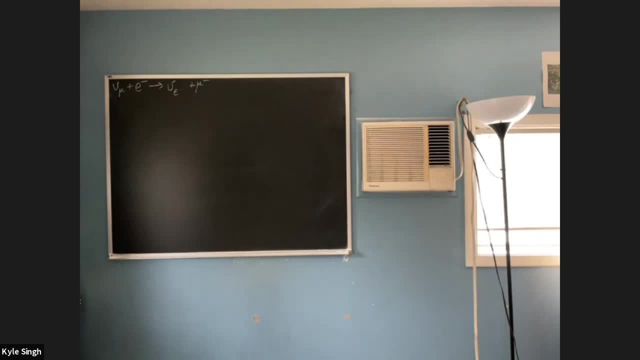 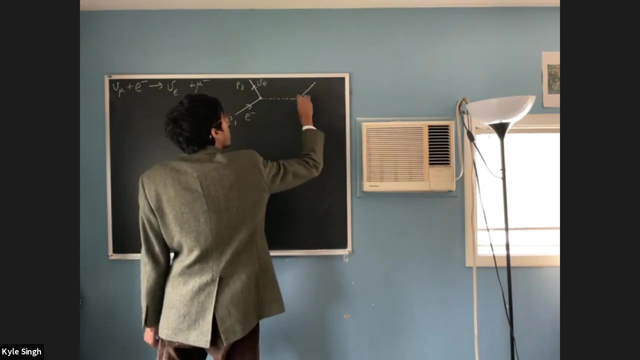 be the process. So let's draw the Feynman diagram. We'll call this P1.. We'll call this P3.. We'll call this the electron. Let me see if I want to do this. Yeah, we'll call this the electron neutrino. We have an internal line, another vertex. 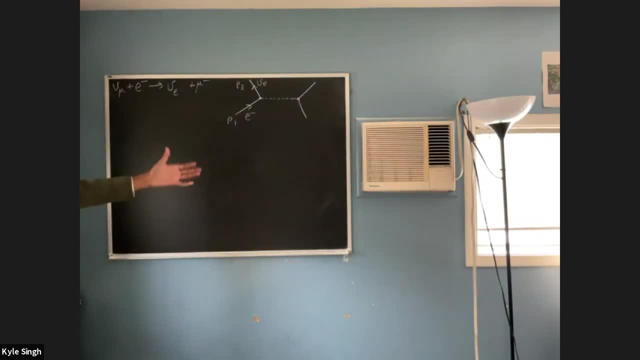 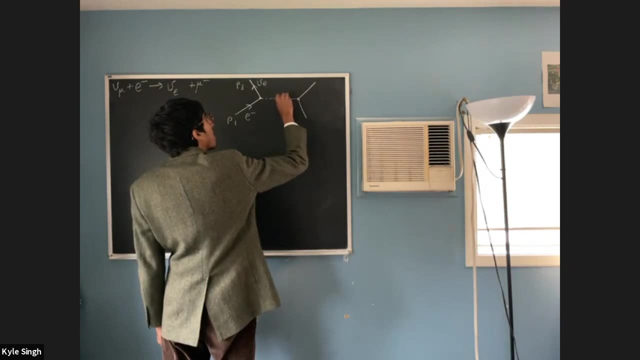 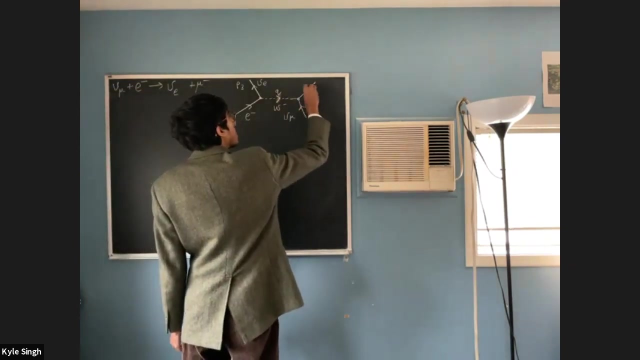 All right. so now the internal, the virtual particle that's exchanging the forces, the W boson. we're looking at negative interactions For now. So, and some internal momentum. Q right, This is the muon neutrino, This is the muon right, And we'll say: this is P2 and P4. 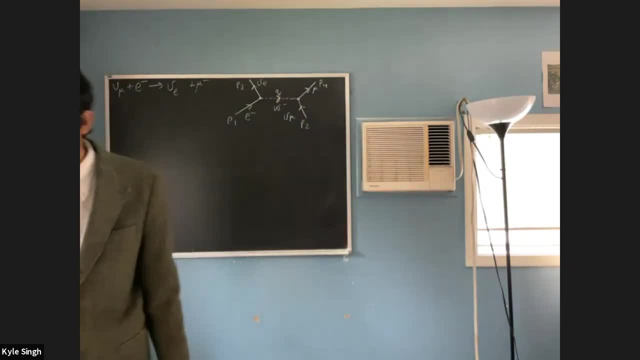 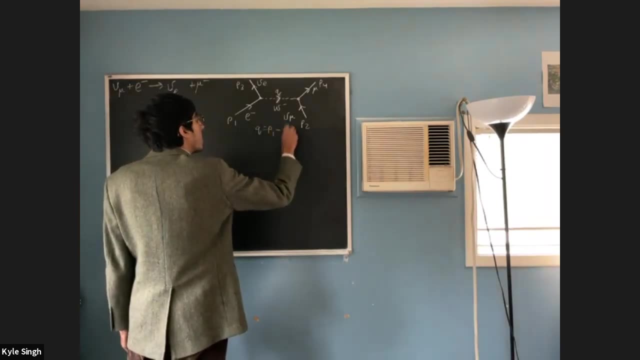 So I'll give you a second to write down the amplitude. Right and just just remember so. Q equals P1 minus P3.. Right and just just remember so. Q equals P1 minus P3.. Yeah, And we'll work in the limit again where Q squared is much less than M squared, right? 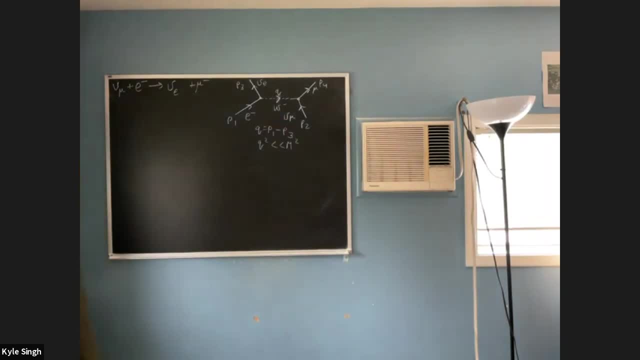 Which is the basic kind of like weak interaction limit, And we'll call this Mw for W boson, just because it's a different mass than the Z. Okay, so I'll give you a second work that out and then I'll give you the answer. 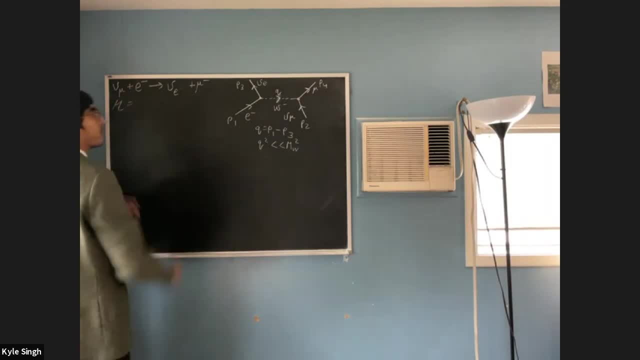 So, remember, we want an expression for the amplitude And I'm gonna write down the magnitude of theasa, Okay, So I'll give you a second here. So what we'll do is: let's take a look at this wave, So let's maybe write down the amplitude, right? 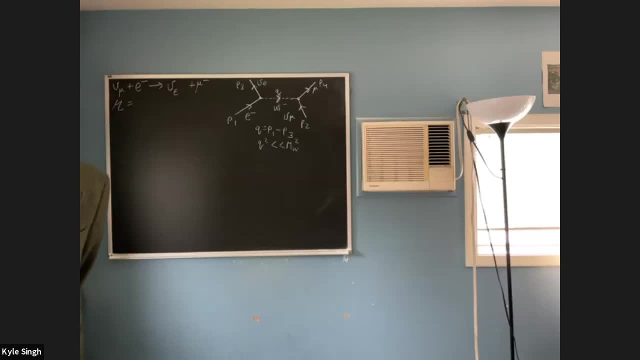 Okay, Because we know that for a second this is going to be negative. So we're gonna write down the magnitude. Let's write down this wave. Let's take a moment to think about this. So we've got another wave. This wave, these waves are coming from the beginning of the sieve. 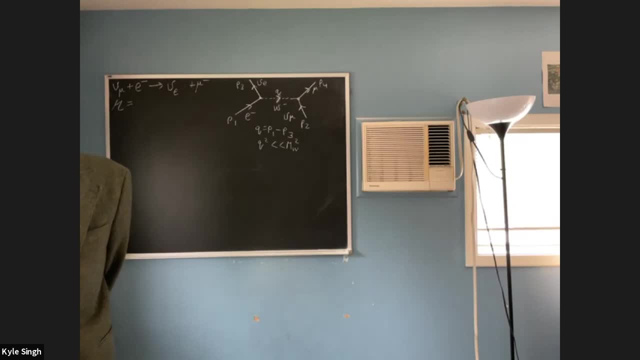 okay, let me write it down. so we have two vertex factors, so we're going to get like gw squared over eight times mw squared, right. that's just from the two vertex factors, okay. and then we have some spinners, right, so we have one. they're all. they're all. particles no. 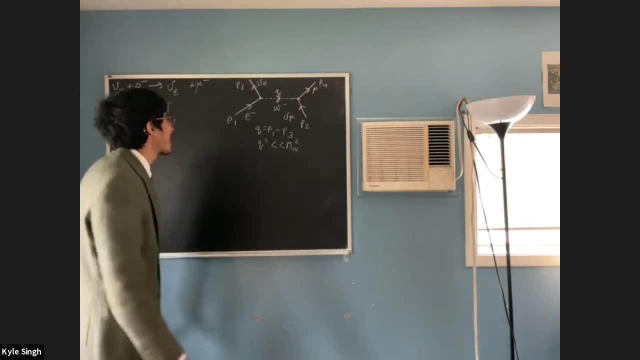 antiparticles. so they're all going to be. have u's right, that's, that's the thing. so i have some u? uh of p1, okay. then i have that vertex factor, so the axial electric coupling gamma u1 minus gamma 5 times u bar of. i'm just going to write the numbers. so u bar. 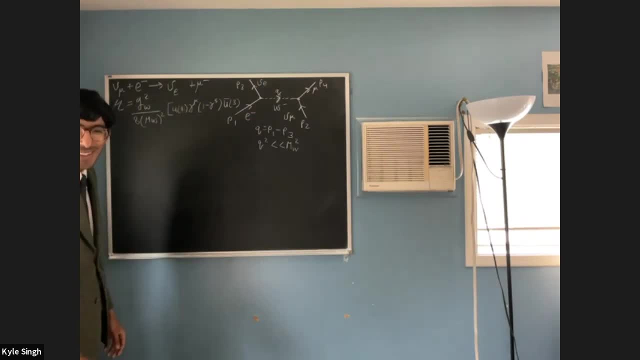 three. we'll do it in the basic like uh, spinner helicity language where we just write the numbers. okay, so that takes care of all of that. i have my propagator. oh, i need a propagator right, one propagator right for the internal stuff. actually, wait a second, this handles the propagator right. 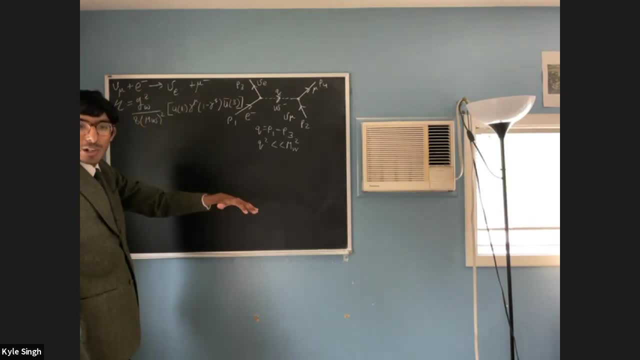 because this mw squared pops out. i don't need the q squared term, right, that drops out because i'm working in that limit. um, yeah, okay, so then i get one more term. i get some like u of two, gamma, mu, one minus gamma five, u bar of four. that's it right. 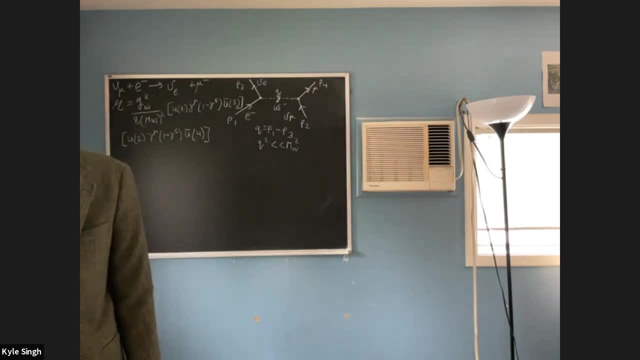 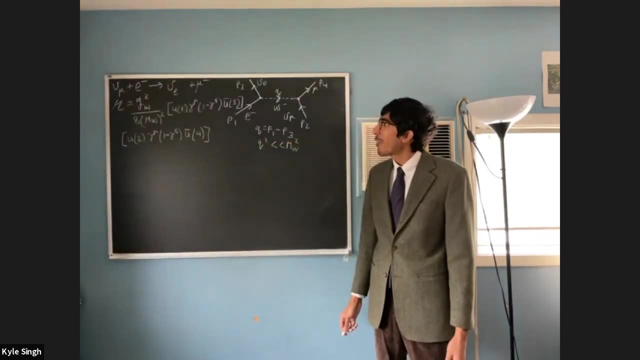 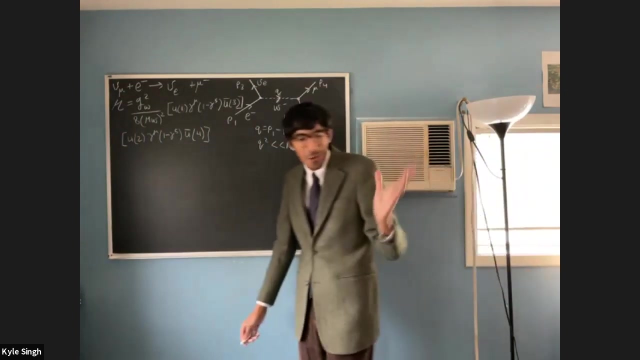 on. yeah, this is okay, this is. this isn't going to work. just to figure out like you enjoyed it sometimes. the easy part. now we have to. now let's do our basic procedure where we sum over the spins, use the trace rules, do all of that. you know annoying stuff which when we did QED. if you're 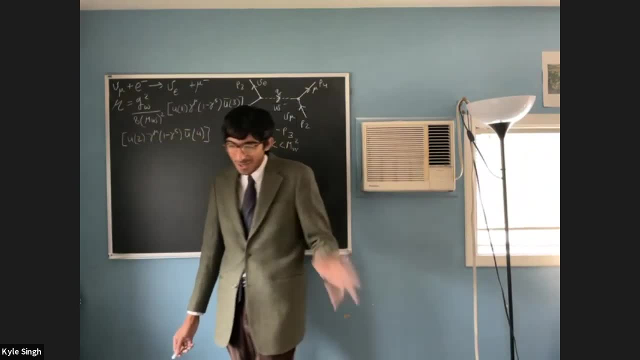 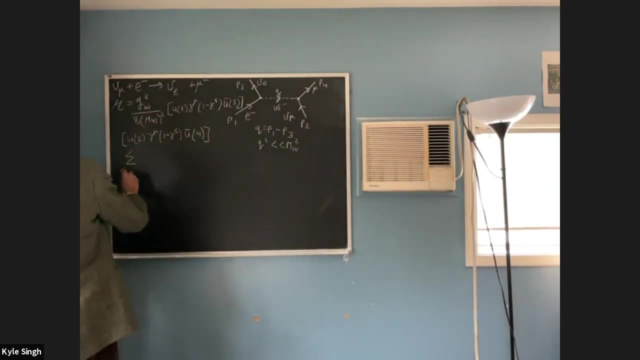 confused. you watch that lecture because we did that really slow, but I'm just going to do it fast today, when you've done these long enough, you can just stare and then get the answer. so I need some sum over the spins right of of. obviously m squared right. that's the whole idea now. 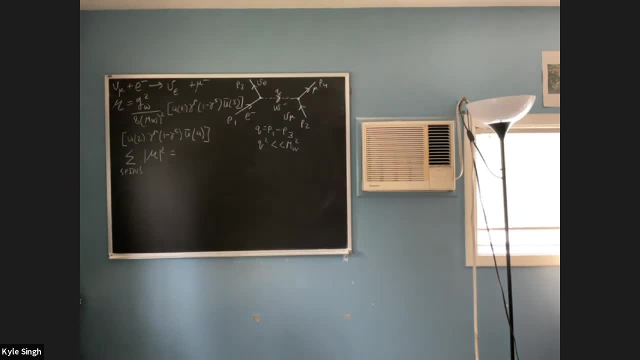 so the easy part: e w squared over eight m w squared squared. that's the easy part. okay, so trace gamma mu times one minus gamma five. that's that's okay. okay, right, okay, this one's actually not bad. p slash one plus m e. I'm just using the trace. 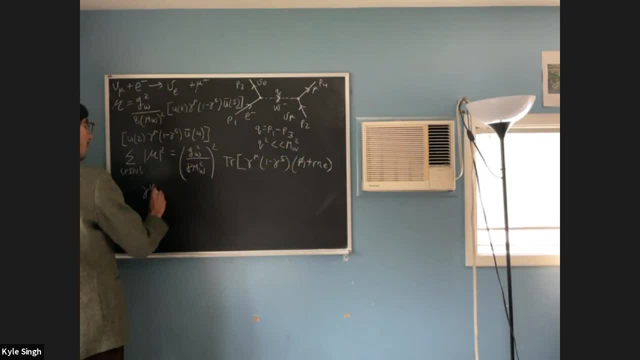 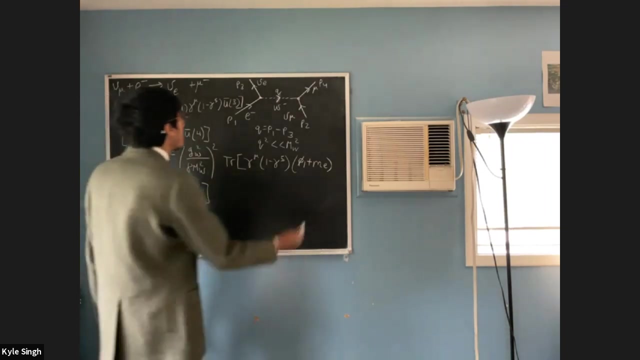 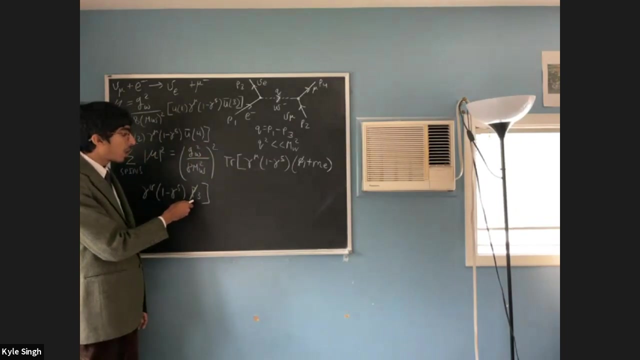 properties: gamma, mu one minus Gamma five p slash three done. So that's the first term right, Because this p one is massive, So it gets some mass term right. But then the neutrino, the p slash three, does not get any mass term right. 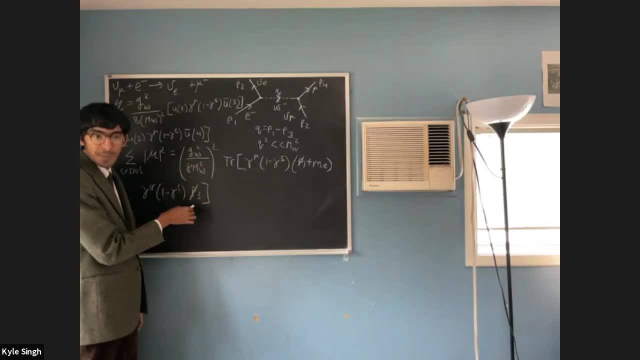 Because neutrinos are practically massless for our intents and purposes. okay, Okay times. now I have to translate this term right, Using the trace rules, because I just did this term, Now let's do this term. it's the same game. 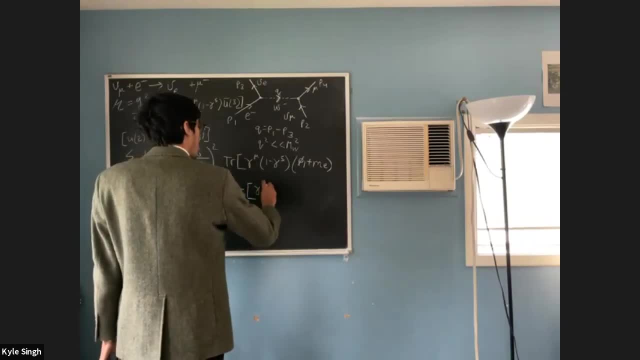 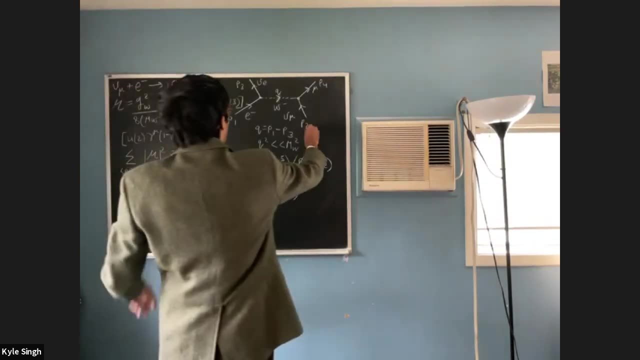 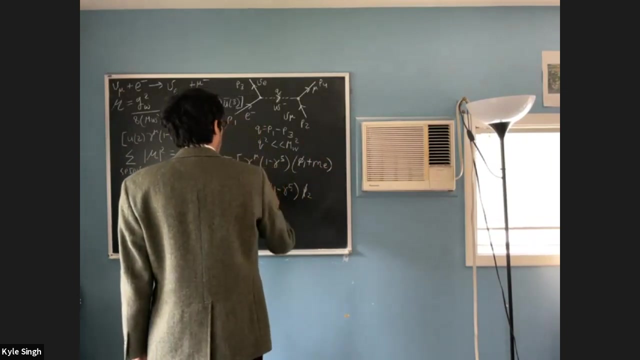 So times trace gamma mu one minus gamma five. And now this time the massless particle is gonna be two. So I get like p slash three, It's gonna be two. right, This should be a lower index. actually, It's gonna contract with that guy. 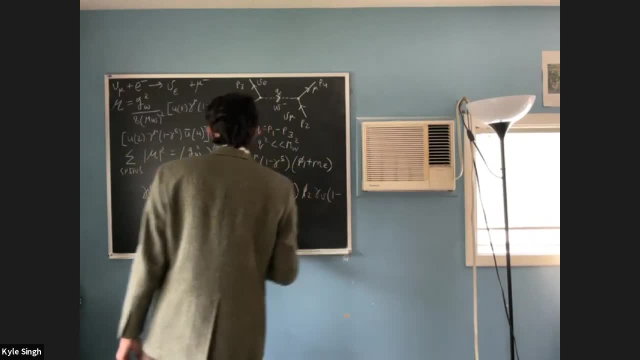 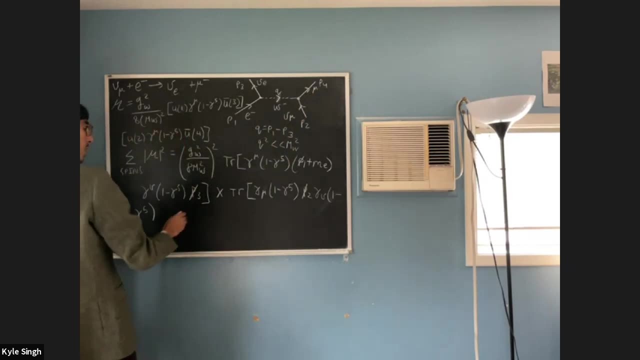 And then I get some gamma mu one minus gamma five, And then I need from this guy. So then I get what I get: p slash four plus m mu. okay, That's the second step. So let's work out the traces. 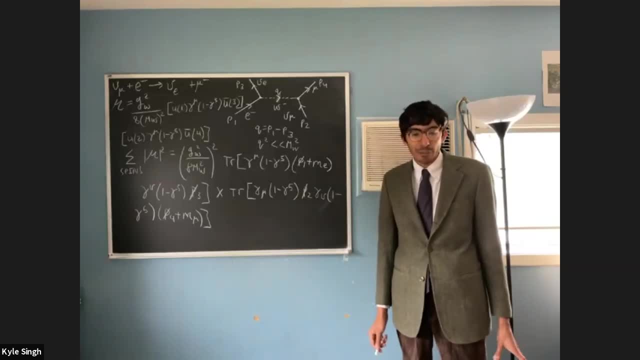 By the way, like, even if you're really confused, right, You should go into the book and, like you did Jenna, where you followed all the spinner helicity, you should follow the steps for these kinds of things, Because if you can do this kind of calculation, 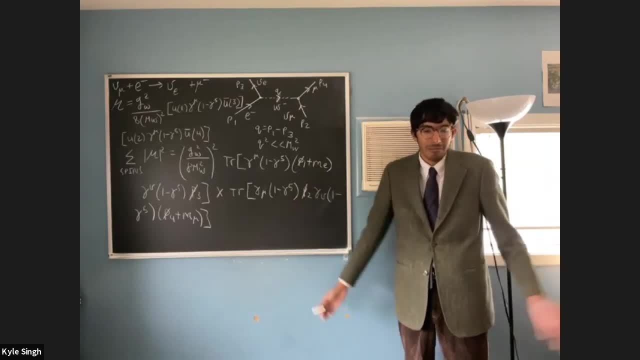 you can calculate any basic amplitude, at least at tree level, right? This is all there is to it. It's just the trace properties and that kind of thing. And then at loop level, let's not even talk about it. We know what happens at loop level. 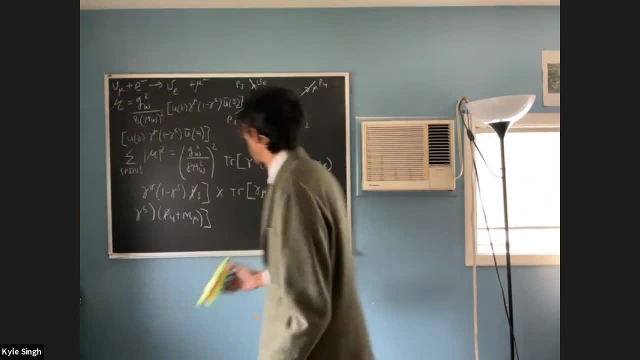 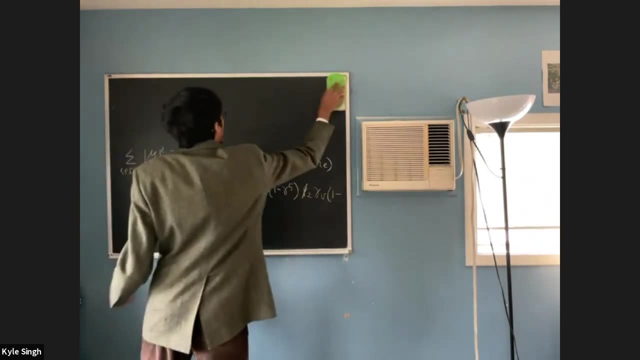 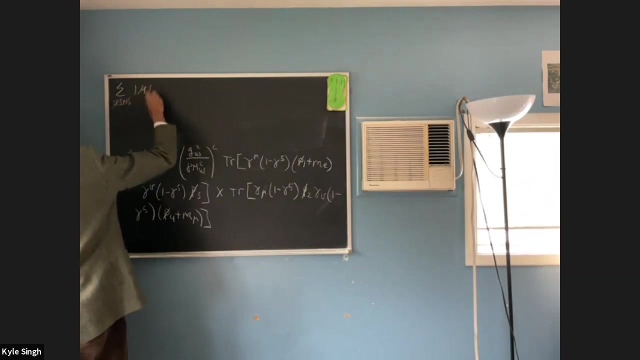 We have a lot of issues, Okay, so let's evaluate the traces. I'm just gonna rewrite this term on top, All right. so then the sum over the spins. I'm just rewriting this guy, So I'm gonna write m squared pw squared over eight mw squared squared. 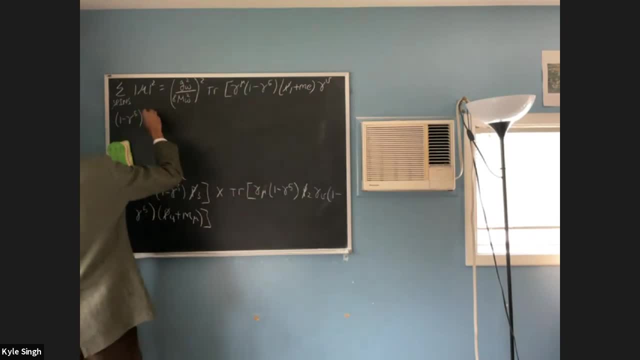 I don't know if a lot of people understand this, because I'm good with it, But I'm not gonna say why I have three sets of three. I'm gonna write the patters: theбы's, they, ys and ys. 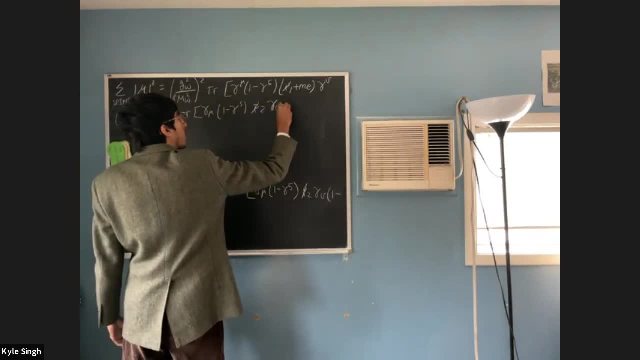 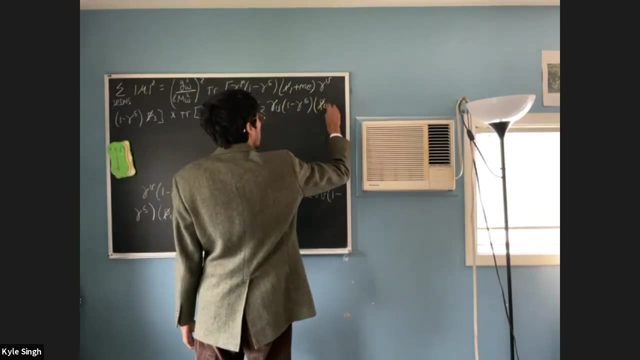 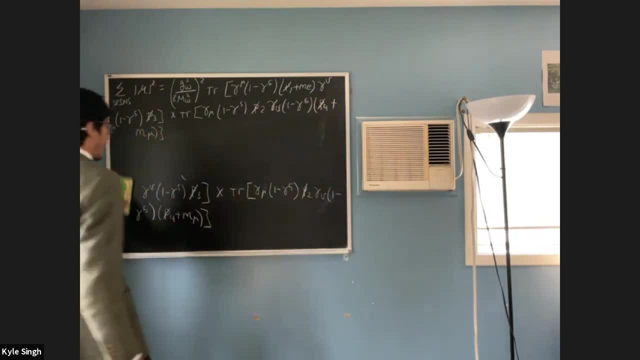 Let's take the data back. So that part, you're gonna do that, All right, Great, Okay, Let's evaluate the first trace. Okay, So I'm going to call this first term. So we'll call this first term rho. We'll call this second trace term sigma. 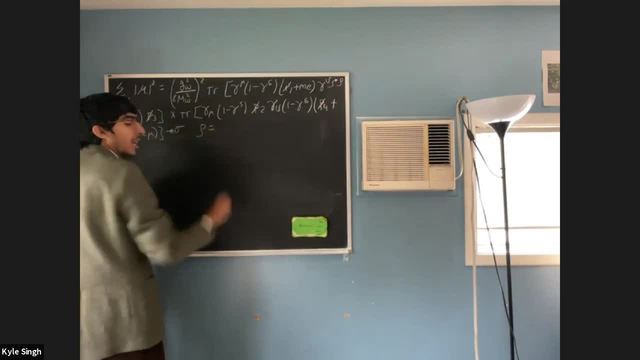 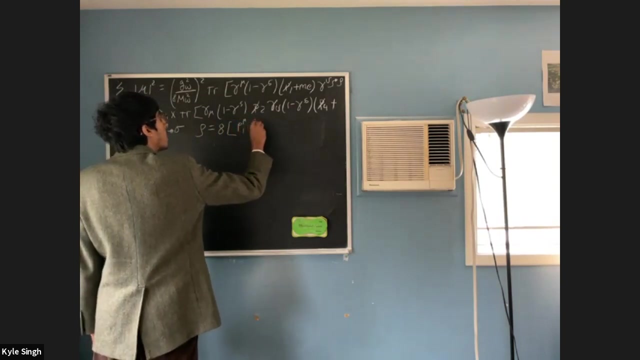 So let's evaluate rho. So rho equal. I always like to do that because then it's easy. I just like labeling them. So rho is just what I'm going to get: an 8, p new 1, p- new 3.. I'm just using the trace properties. 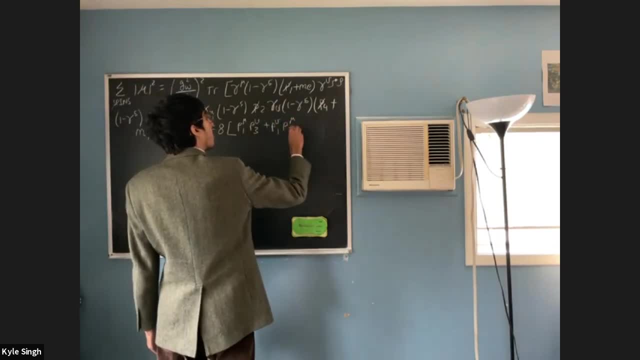 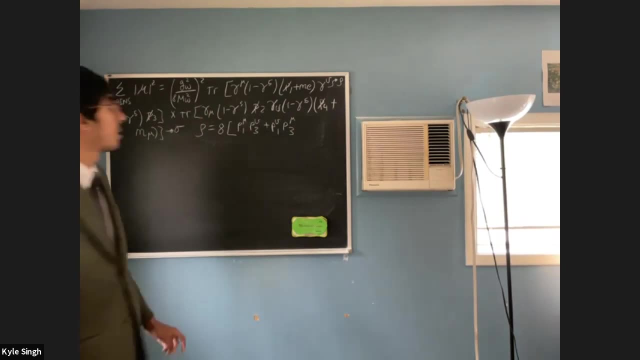 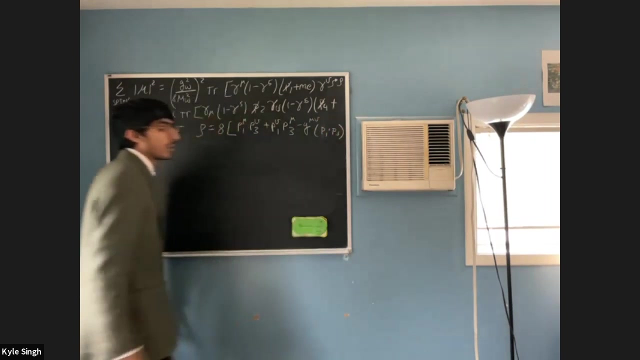 Plus p new 1, p new 3.. Once you start getting the patterns, it's actually pretty easy. Minus g mu nu p 1, dot p 3.. Minus i epsilon, mu nu lambda sigma. Epsilon is just the standard, like for index Levy-Civita. 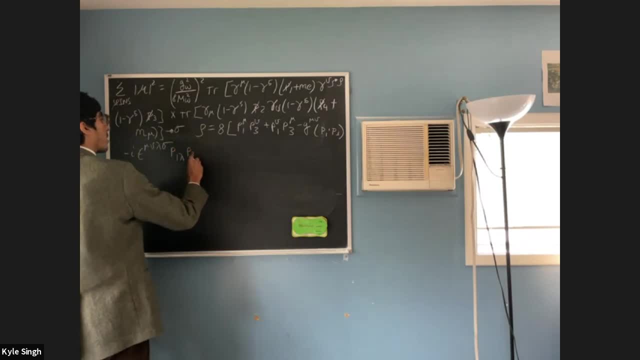 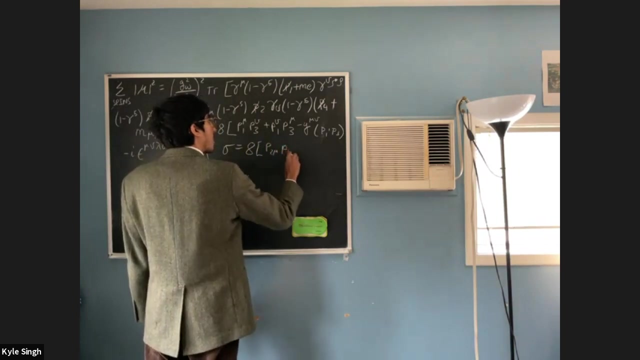 And we get some p 1 lambda, p 3, sigma. That's the first trace. Now the second trace, so, sigma, I get an 8 again. But now I'm going to have sort of the same expression just with the 2s and 4s right, So p 2, mu, p 4, mu, minus g, mu, nu, lower, p 2, dot, p 4.. 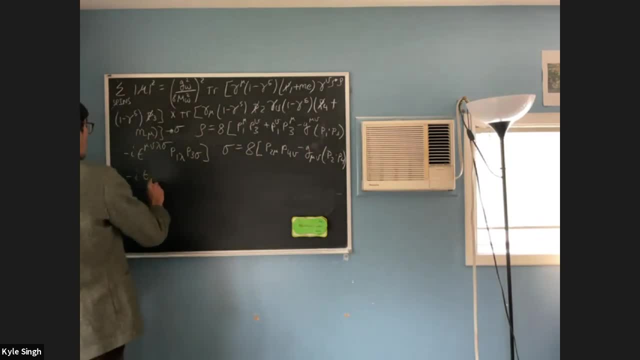 Minus i epsilon mu nu. we'll call it chi tau, Chi tau. p 2, chi p 4 tau. Okay, That's just using the trace properties, So we're going to make use of the following. Oh no, I have the epsilon. 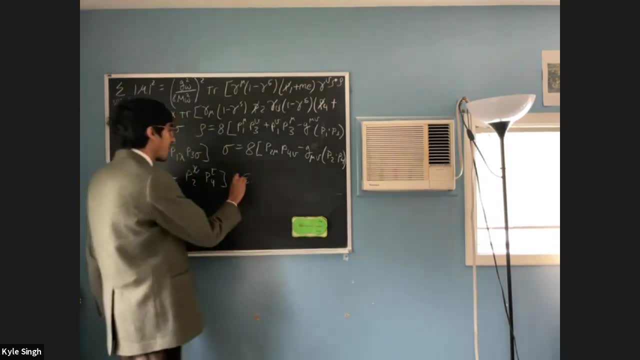 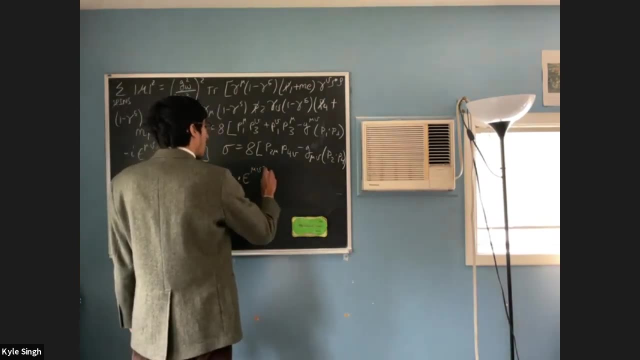 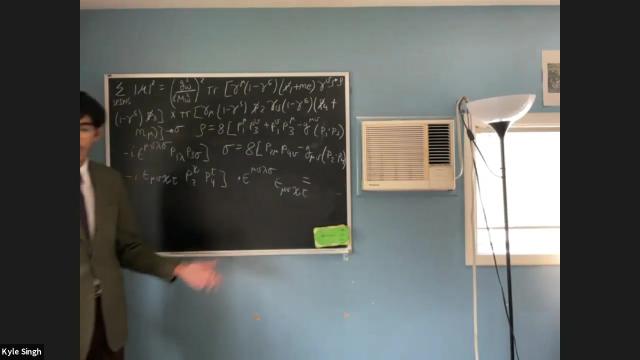 We're going to make use of the following identity between Levy-Civitas, which is a nice one for index Levy-Civitas, And that is that epsilon mu nu lambda sigma, epsilon mu nu chi tau can be just written as a series of Kronecker deltas. 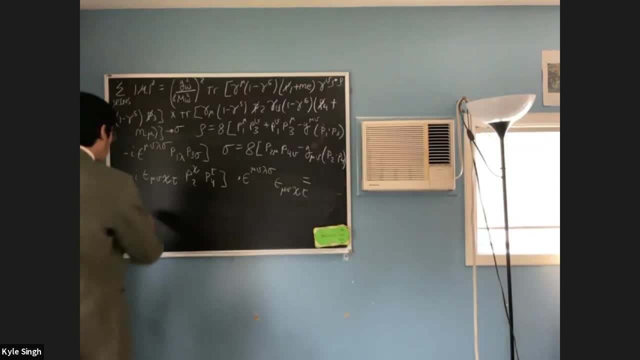 That's a useful technique. So: 2 delta chi lambda- Let me just make sure I'm going to do this right. Delta sigma tau. Delta lambda- tau. I'm going to need one more. Just let me just make sure what indices I'm missing. 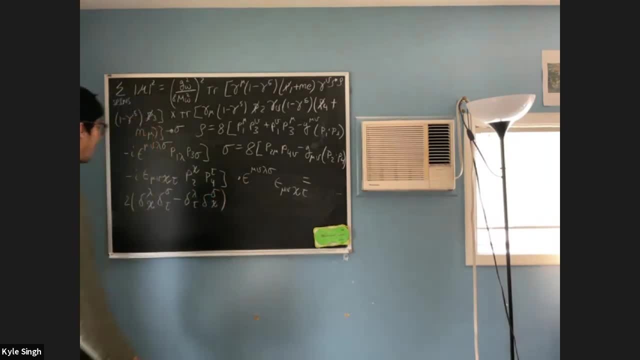 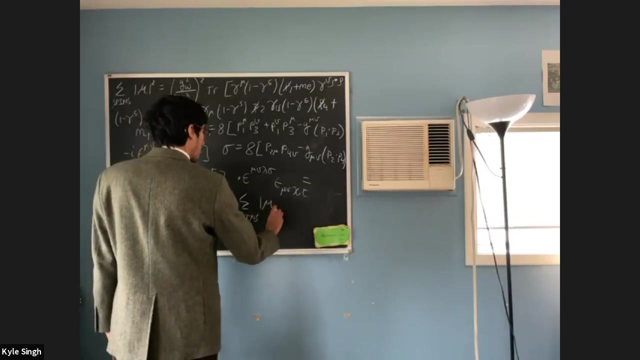 Delta, sigma chi right, And using this identity, now I can just basically, and then multiplying everything out, which is a pain, You can write down that the sum over the spins. let me just do it really quick. It's the following: 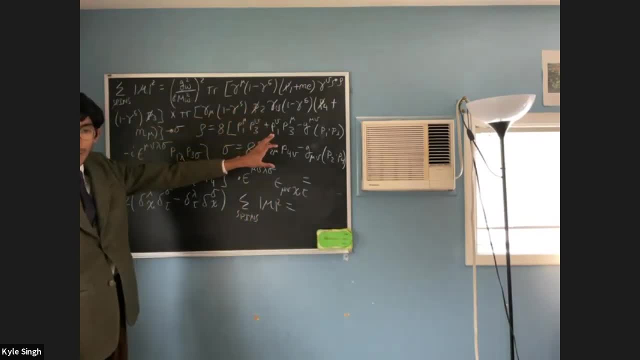 So I remember. now I just have to multiply rho times, sigma right And then turn the crank, That's. that's the easy part. It's tedious, but it's easy. In sigma or in rho, didn't you have another p1, p3 term that you didn't have in sigma? 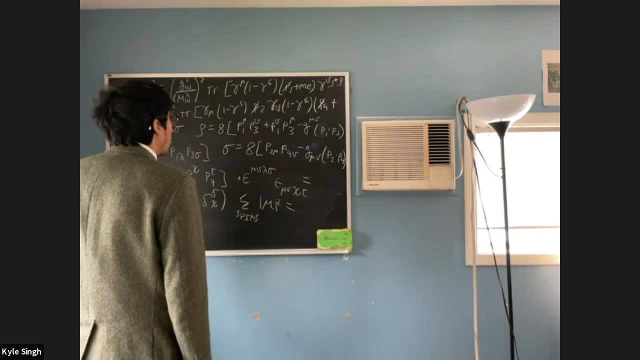 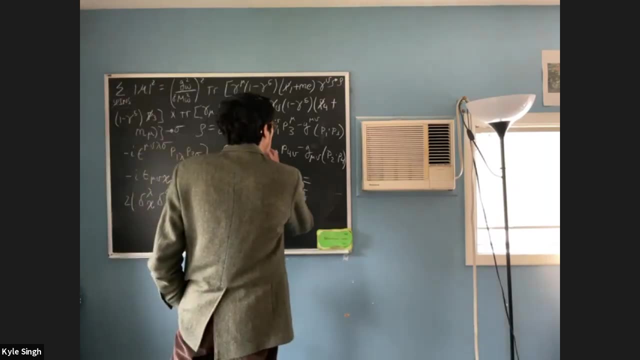 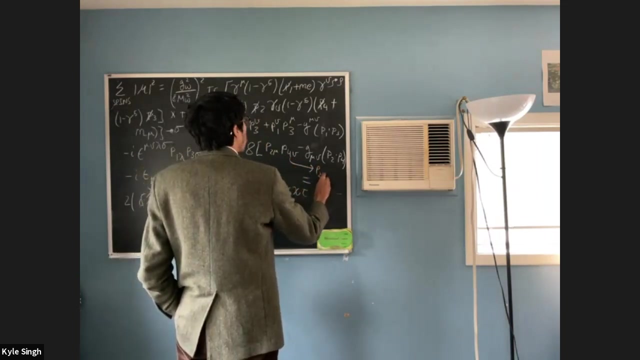 Like at the beginning, In sigma And in rho. Oh yeah, I'm missing the term. You're right, you're right, you're right. What am I missing here? Yeah, good catch, I'm missing a p2 mu, p4 mu. 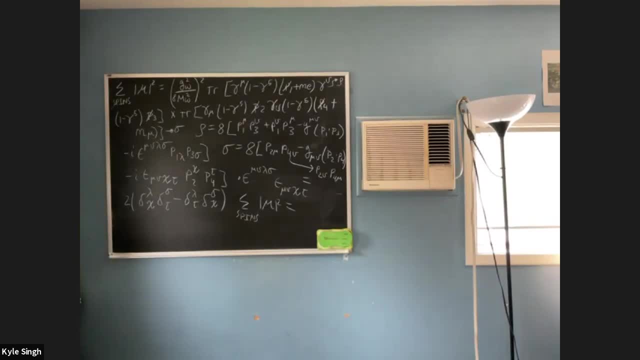 There, Sorry, Good catch, Yeah, yeah, absolutely Okay, good, Okay. So let's write down the final expression. So we're going to get some 4gw over mw to the fourth p1 dot p2.. It's a very simple expression actually. 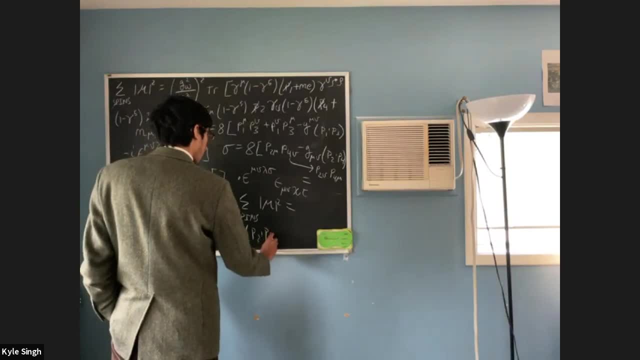 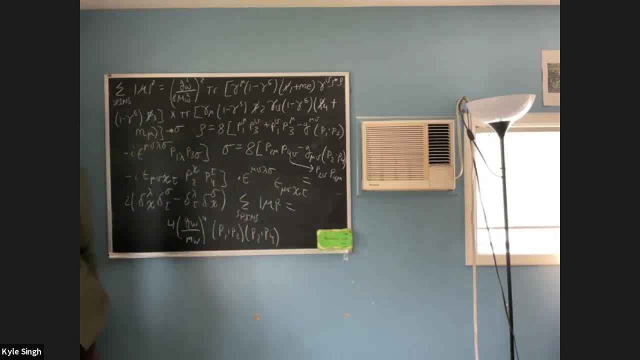 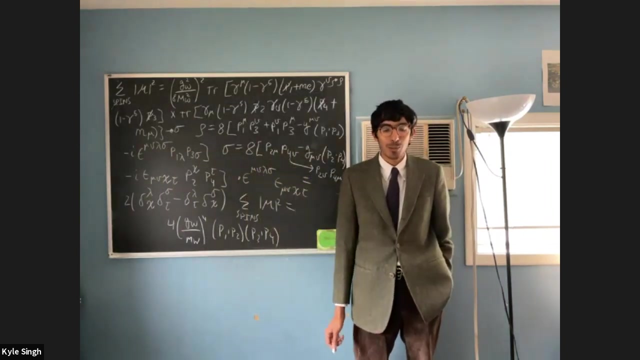 If you just think about it: p3, dot, p4.. So that's that's what we get when we sort of wrap everything up. Let's write down a cross-section. This should be very kind of like. you know you're looking at this having seen some spinner. 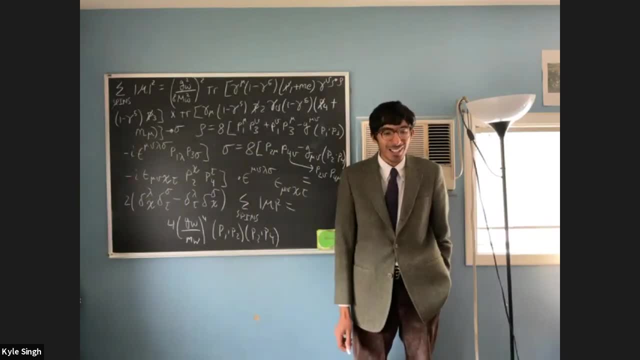 helicity right. This should be very like suggestive that you can write down general amplitudes of just dot products of momentous right If you ignore the mass right. So this is a nice kind of thing because, like it's no, it's no surprise you get such a nice. 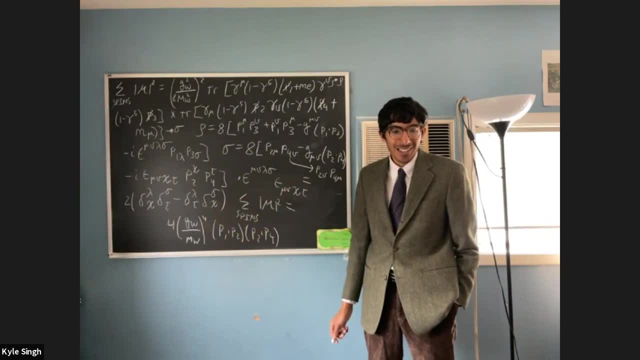 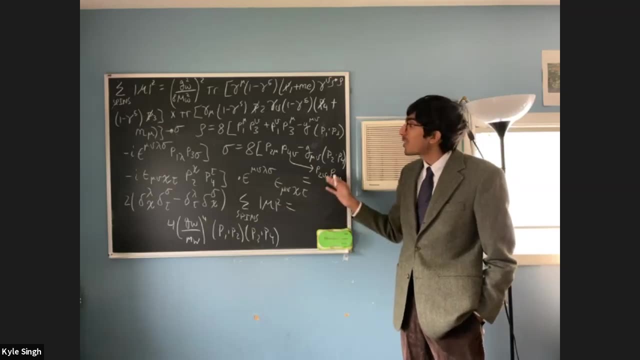 simple answer, right, It's kind of nice, Okay, so I hope this is somewhat instructive. I you know it wasn't a waste of time, I would go through all the algebra slowly and look up the trace properties. see where. 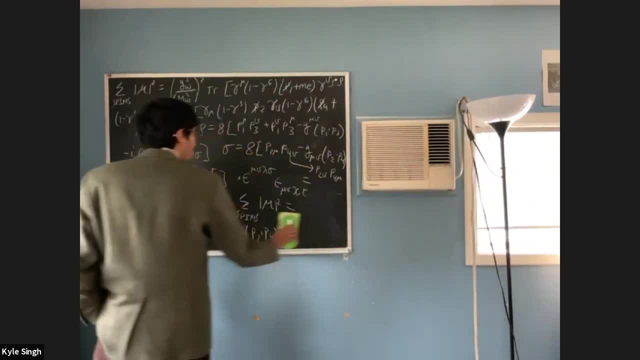 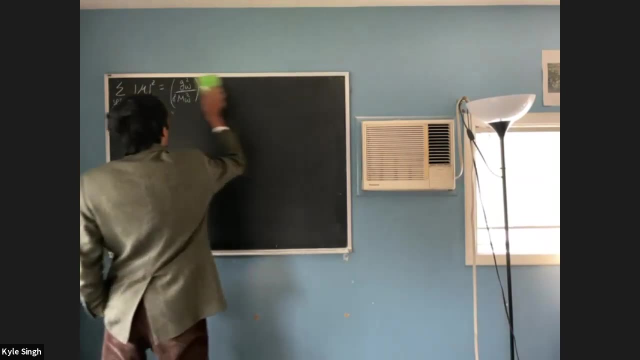 it's all coming from. Okay, let's just write. I'll just write down the cross-section. That's not really a difficult thing to do now Because we have, once we have u squared, we can write down m squared, sorry, and write. 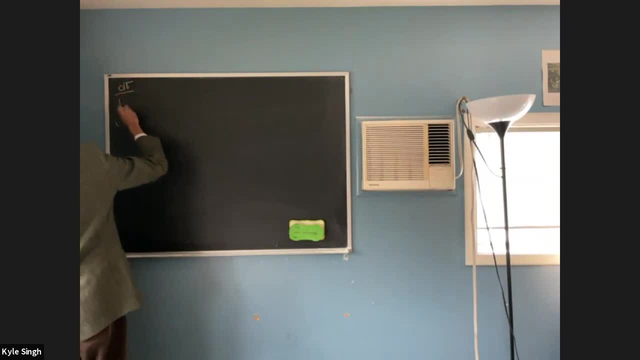 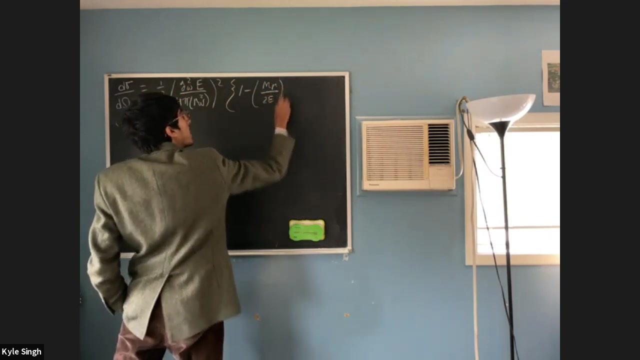 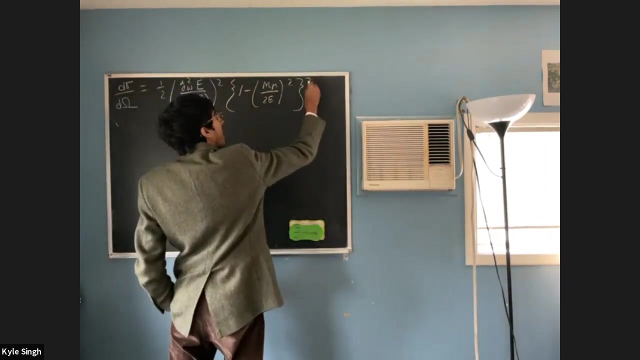 down a cross-section, So d, sigma, d, omega. So let's write down some differential cross-section: One half w squared e Four pi m w squared squared. One minus m w over two, e squared squared Should be squared again, if I remember correctly. 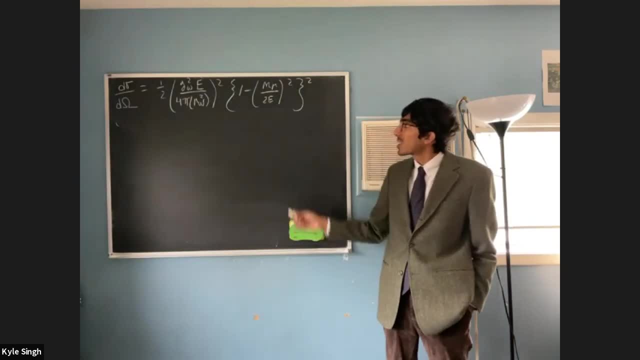 But check that okay, Because- but this looks similar to some of the QCD stuff that I've been putting in the document, Some of the cross-section, except there's some cosines and sines which will be introduced to today. 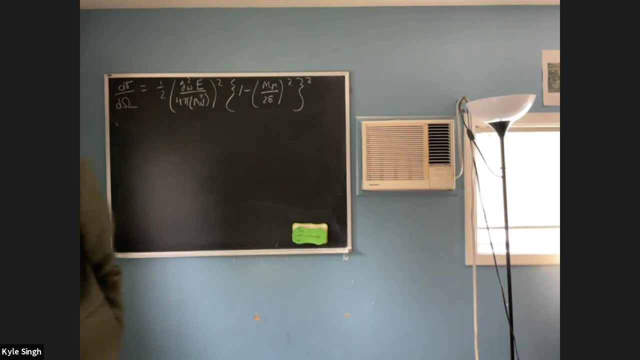 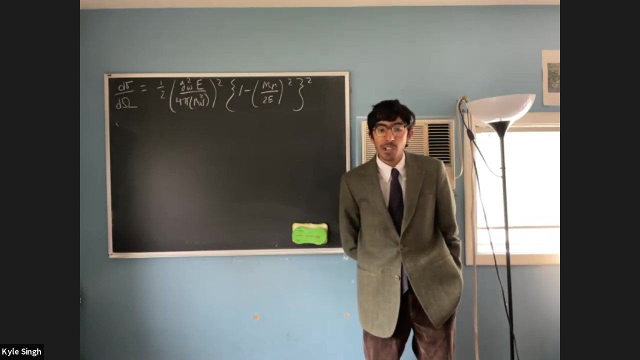 Why, why, why they come up. Okay, so actually the first person to try and come up with a theory of a weak interaction, really a beta decay interaction, was Fermi right, And Fermi wrote the first paper on the weak interaction, on his theory of the weak interaction. 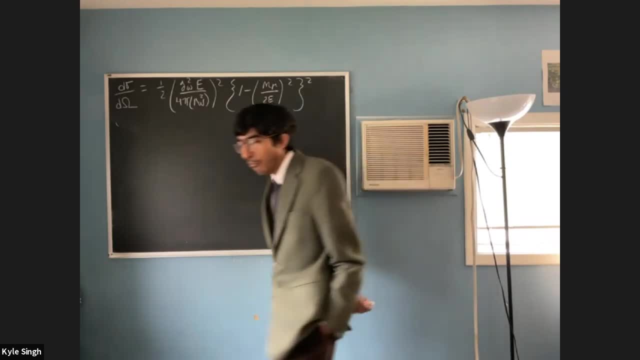 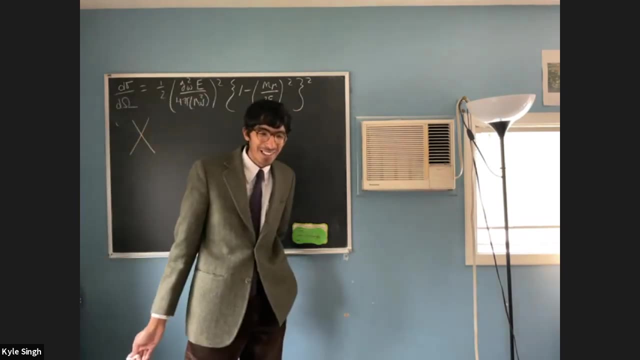 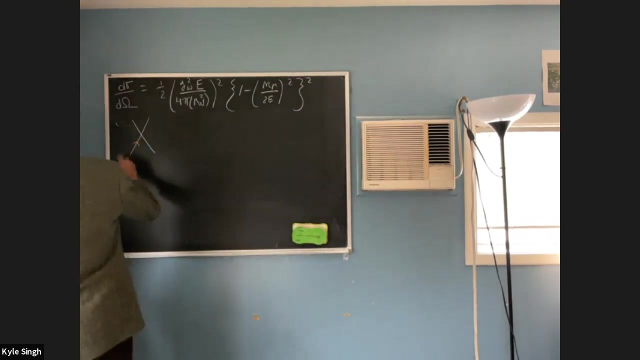 in 1933.. And he had the following diagram. So this is what Fermi- I mean he didn't draw a Feynman diagram, but this is what he was describing. He said that you would have some e go to mu right. 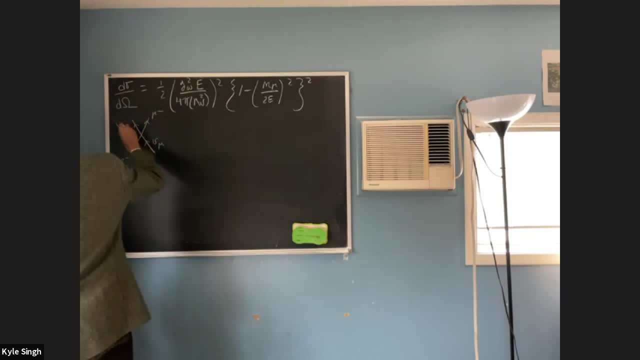 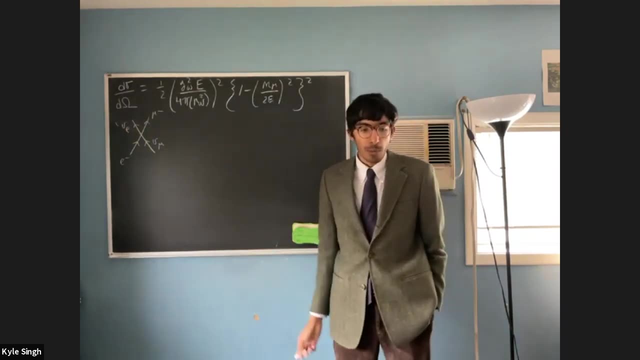 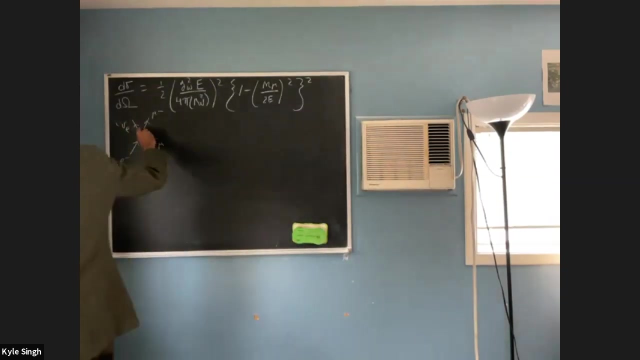 And then give off a muon neutrino and an electron neutrino. But he did not have any massive muons, He just had a virtual particle. You just had a direct four particle coupling. Okay, That was what Fermi thought was the correct theory. 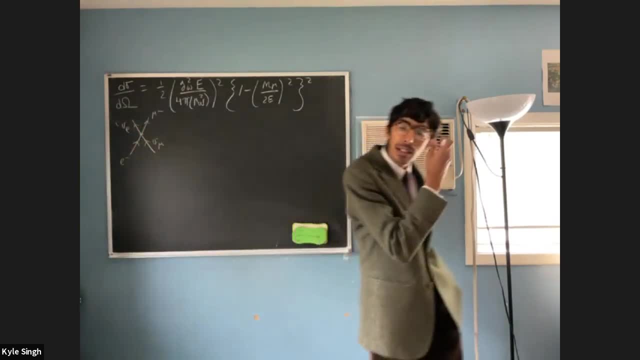 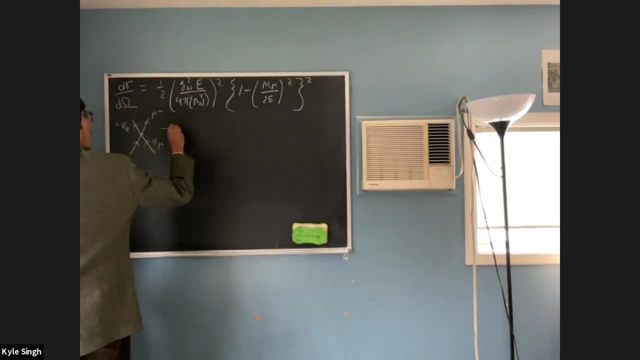 And it didn't work. obviously The cross sections didn't match up. A lot of this stuff was not correct, So people had an inkling. So this was. let me just write it down. So this is Fermi. This was Fermi's theory in 1933.. 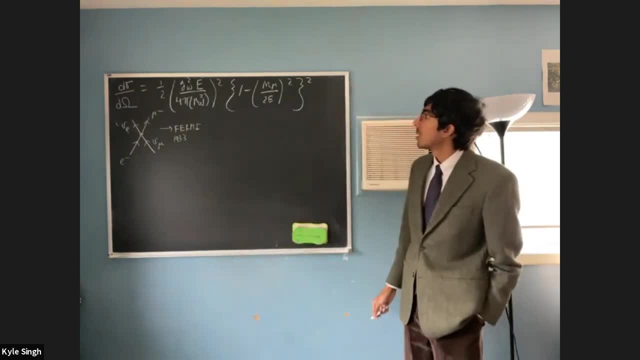 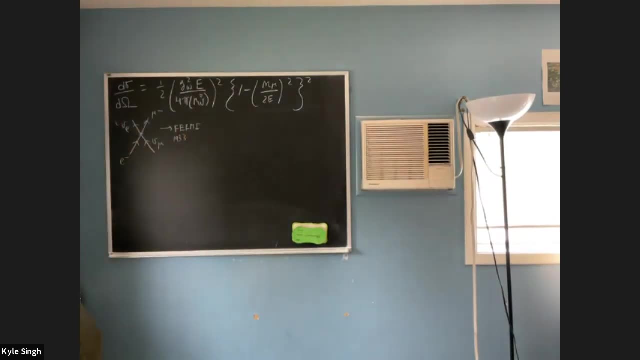 So it became apparent that something had to, something had to resolve this. Okay, Let's look at another very famous sort of weak interaction process. Okay, Ie pion decay. So pion decay is a very famous process in the weak interaction that. 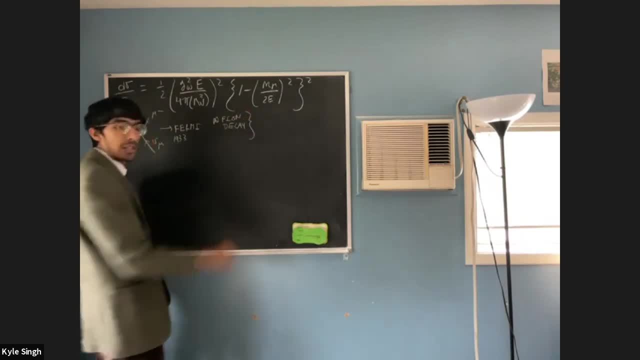 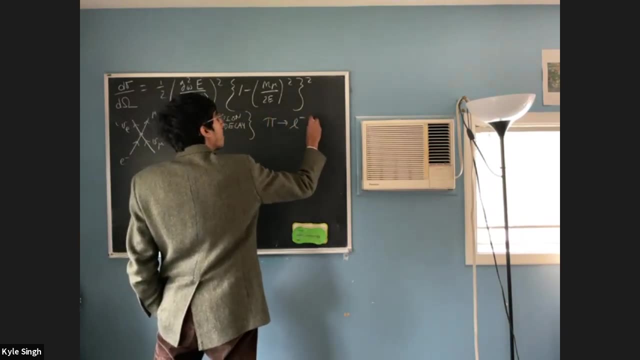 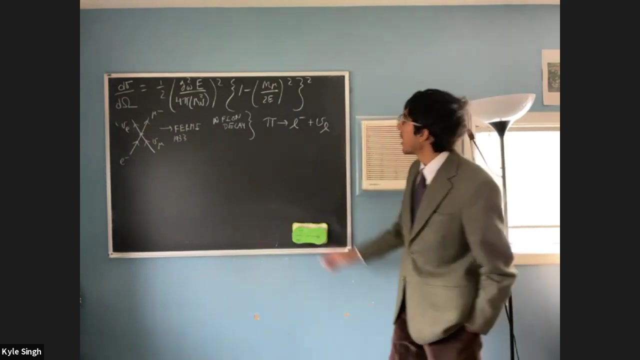 students look at The pion decay. Okay, So pion decay is the process where the pion decays into some lepton plus that corresponding neutrino. Okay, Now, here's the thing. Now I can describe the pion. Sorry, this is pi minus. 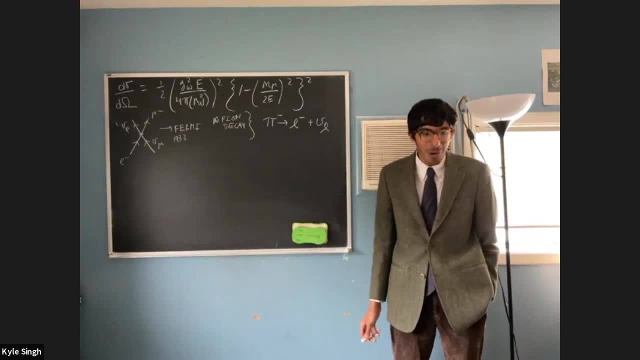 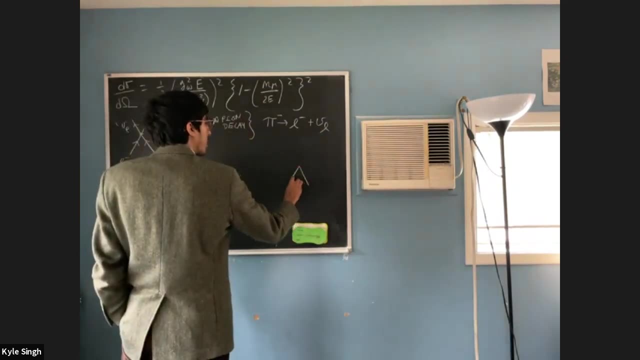 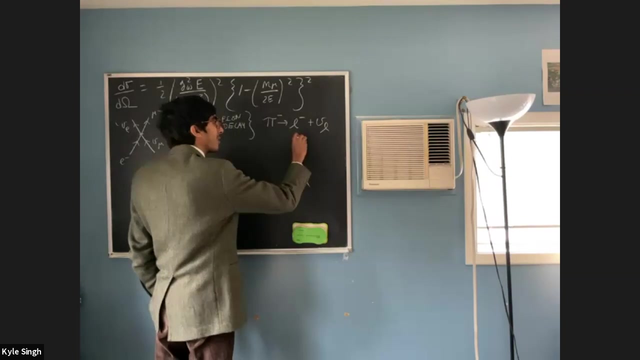 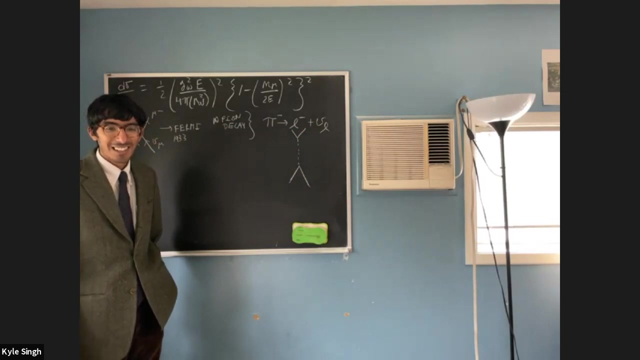 I can describe the pion as quarks. right, It's made up of quarks, So we can describe this weak interaction in the following way. So let's write out What channel am I about to draw: The S, T or U channel? 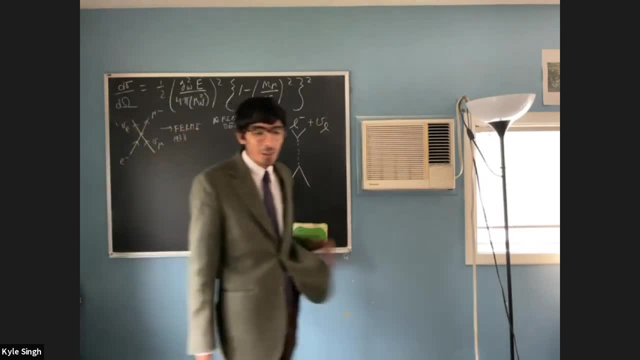 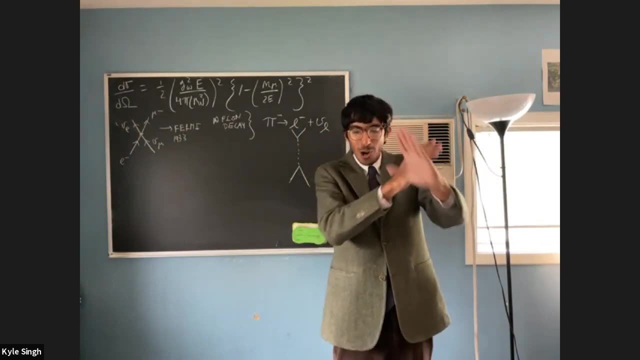 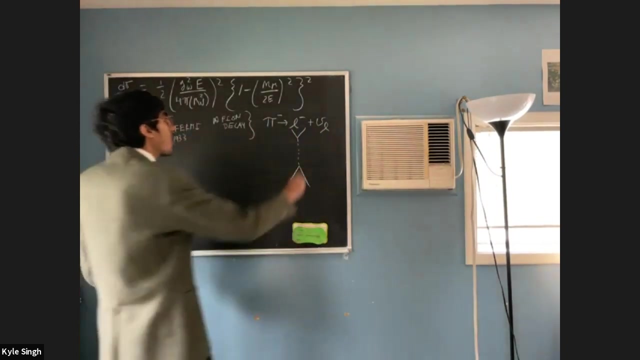 T channel. You know a good way to remember it: S side, T top, And then U is crossed. That's a good way to remember it. Okay, So let's just work out the S channel diagram. Okay, So you have some lepton neutrino. 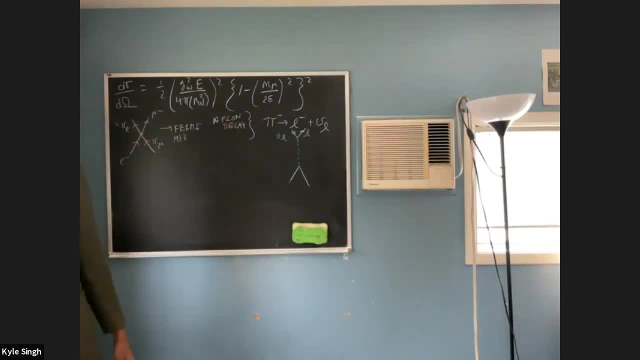 You have some outgoing lepton, You have a vertex here, You have some W boson, W minus boson, Propagating that way. And now the pion I can write down as two quarks: Down quark and up quark. 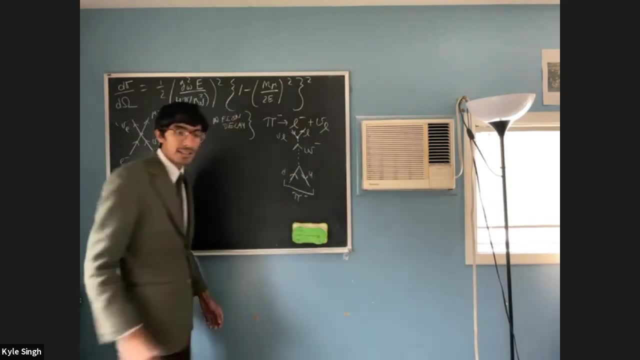 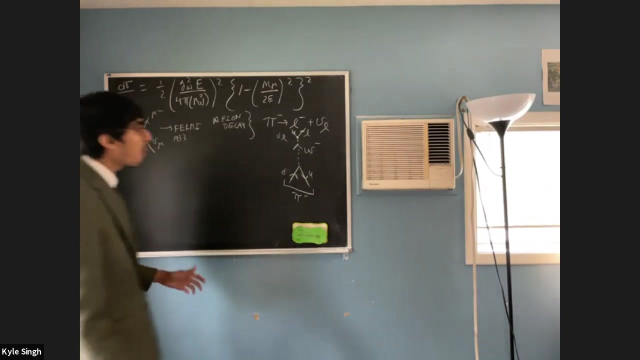 It's a meson. Right Mesons are made up of two quarks. right Nucleons are made up of three. Okay, So that's the Feynman diagram for this process. Okay, Now we don't really. 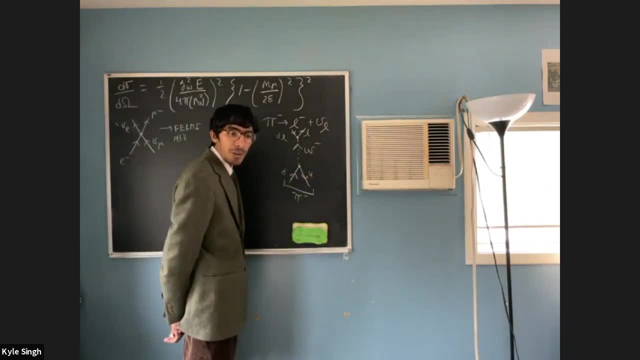 We don't really know how these quarks couple Right To the W boson. That's mysterious. We're not going to get there, And we actually don't even need to know that for this procedure. So let's redraw this diagram. 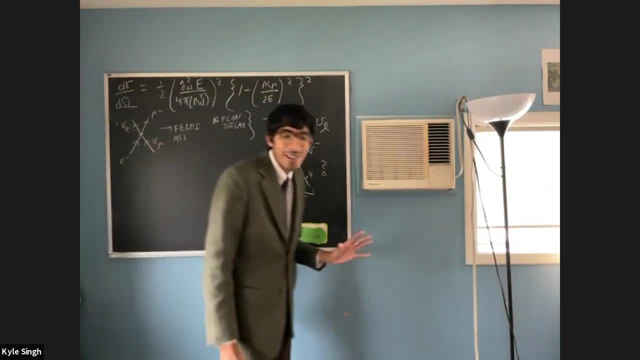 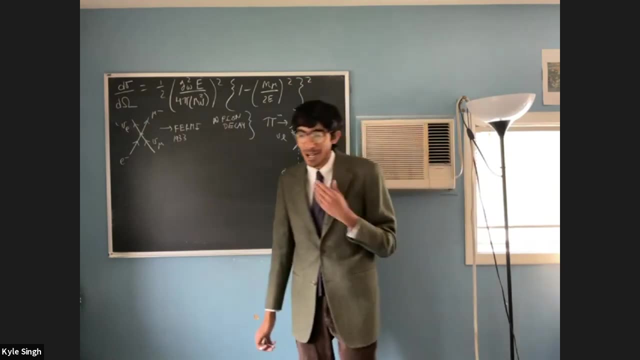 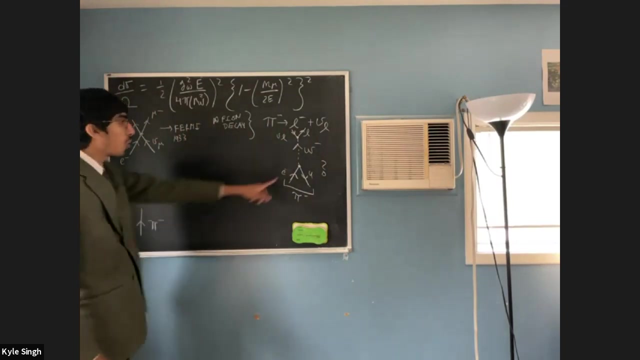 And this is sort of the way it's taught, Because you learn the weak interaction in a particle physics class before. the strong interaction And the coupling is not important. So the classic way this is taught. You have some pion Now. I just wanted to show you that these are. 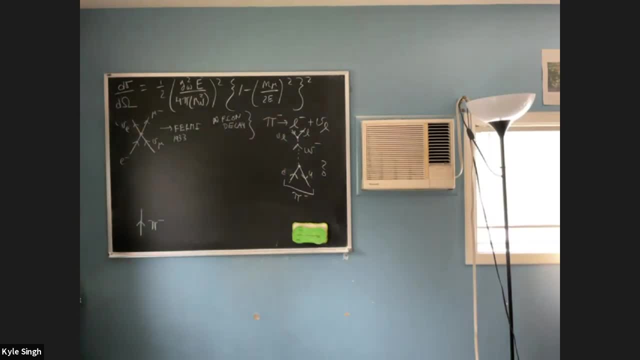 This is why we can talk about quarks in the weak interaction. You have some coupling. We'll call this blob coupling To the W boson. Okay, So now the blob is some coupling, And then there's a vertex factor, And then there's just your standard. 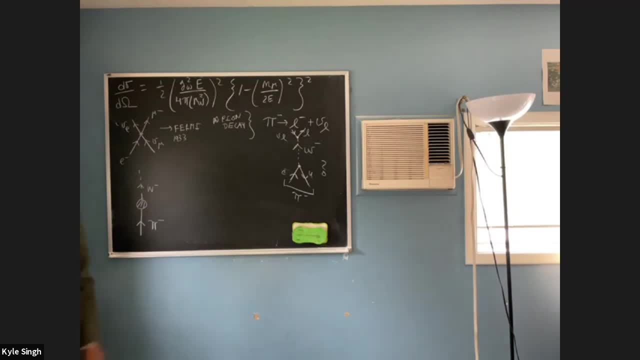 Vertex factor, where the neutrino- Oh actually, Wait a second. I think this goes to this. This is an anti neutrino. Sorry, Sorry. That's why this arrow. I'm like, why am I drawing this arrow? This is an outgoing anti neutrino. 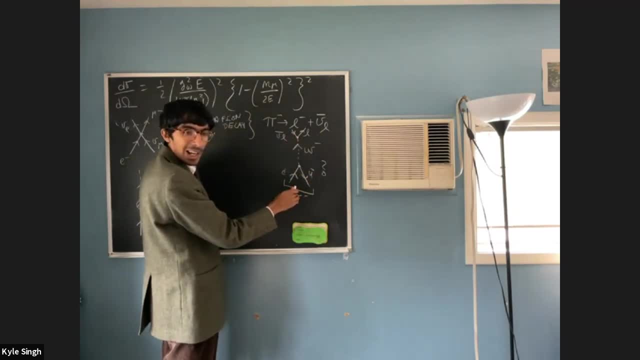 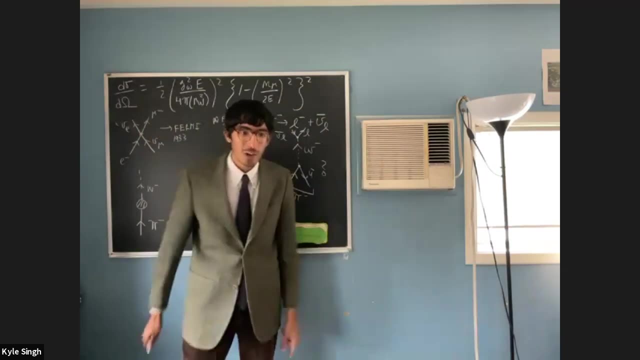 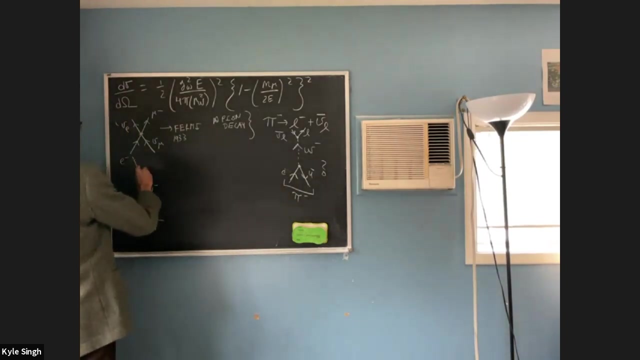 Okay, And this is an anti quark. Okay, That makes sense, Right, Because the arrows are flipped, Because those are both ingoing, Okay. And then you have Again the anti Antine neutrino corresponding to the Laptop. 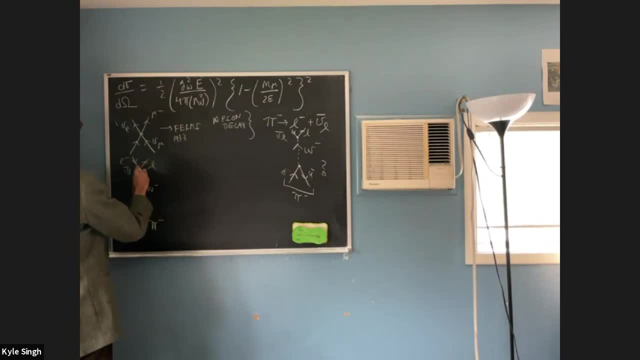 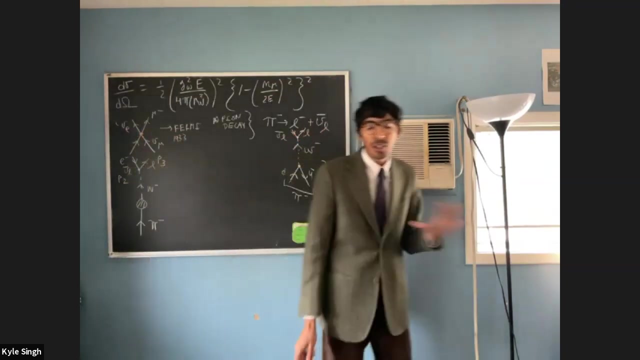 And the left time And a vertex factor, Okay, And we'll say: this has momentum P2.. This has momentum P3.. Okay, So we've seen blobs like this before, right, Yeah, when we drew out sort of like when I wrote out the schematic for you for a general scattering- 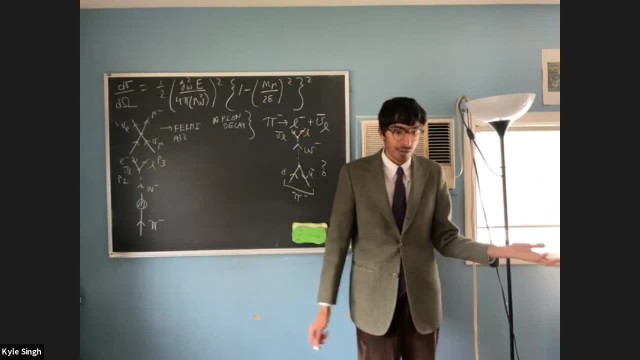 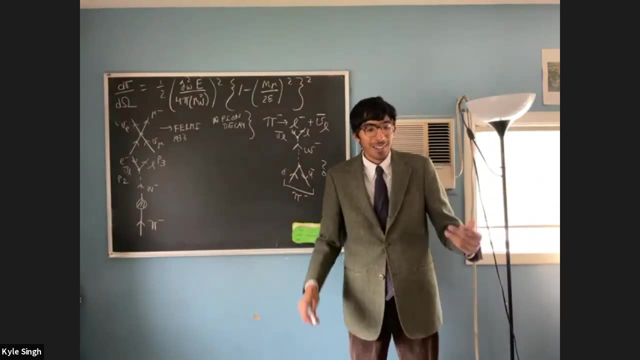 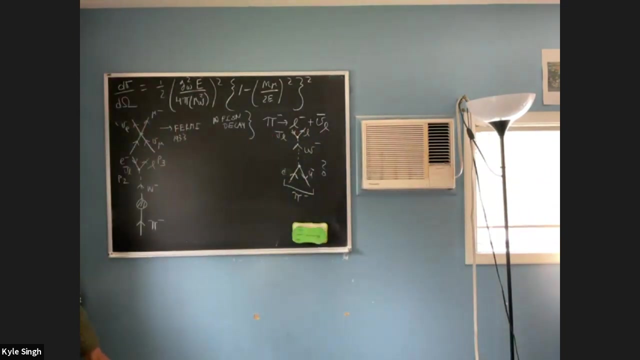 amplitude, right, And these are just called form factors, right, And we can write them as just functions. f, mu, with some factors They're just form factors. So I'll give you a second to write down the amplitude, except this time we're going to call: 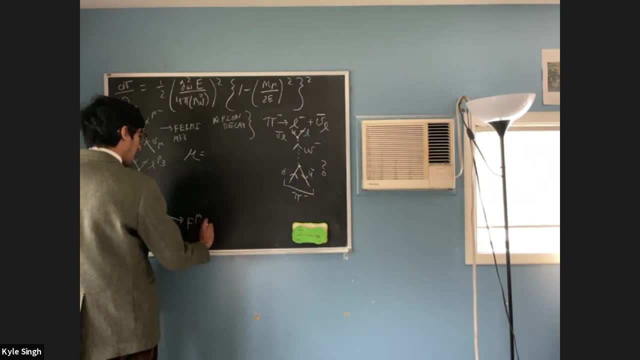 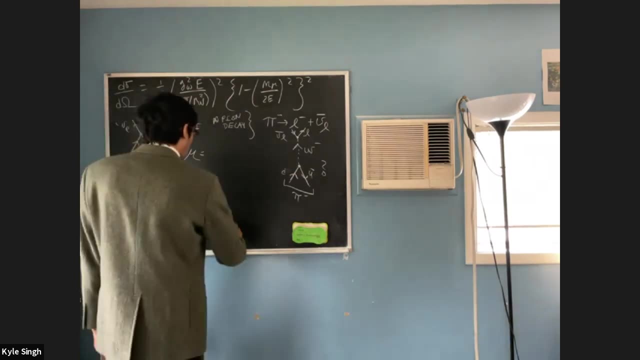 this blob, the form factor f mu, And we're going to say it's equal to f pi times p mu. So it's just some constant that's proportional to the momenta, because that's the vertex factor has to be equal to the momenta. So it's just some constant that's proportional to the momenta. So it's just. 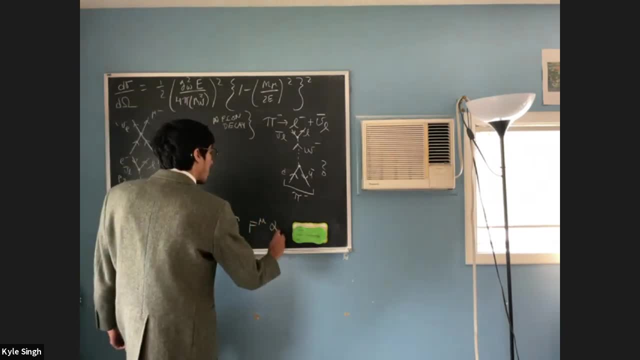 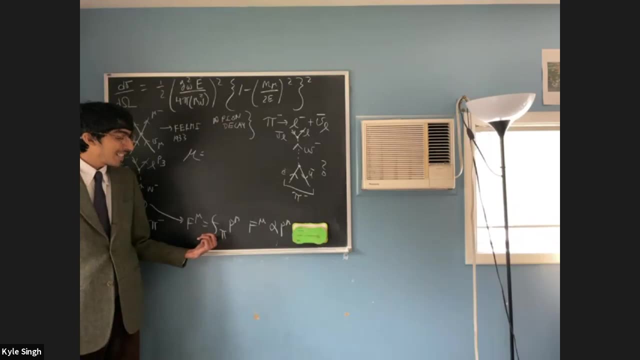 right, Because any vertex factor, so F mu has to be proportional to P mu, right? And then we have some constant of proportionality, right, That's just. and this is actually going to be called the pion decay constant. So you get some actually rate of decay from this calculation. 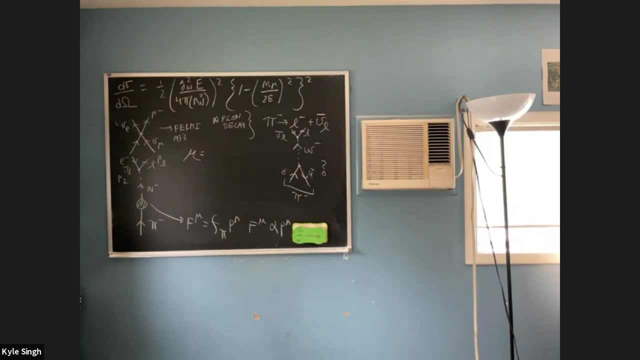 Okay, So I'll give you a second to write down the amplitude. It's really kind of simple, because now you only have to worry about P2 and P3, right, There's only one term, So take a second and just write down that term, So I'll just get you started. So, of course, this coupling is just 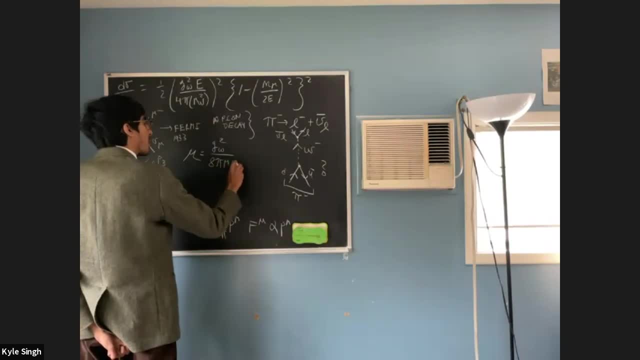 GW squared over eight pi MW squared right. That's from the vertex factor and the propagator. Then you're just going to get one term for the amplitude, So I'll give you a second to write that down. Okay. On the other hand, let's look at this: two area plus or minus work. So we've got. 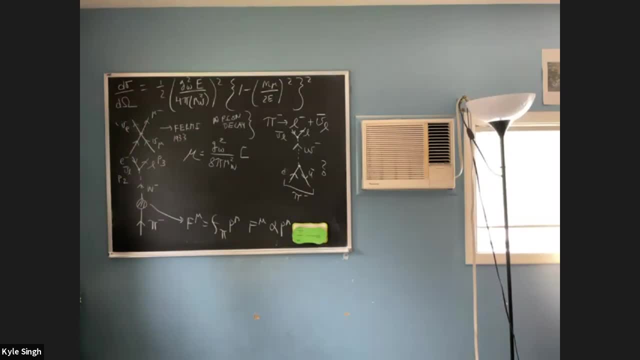 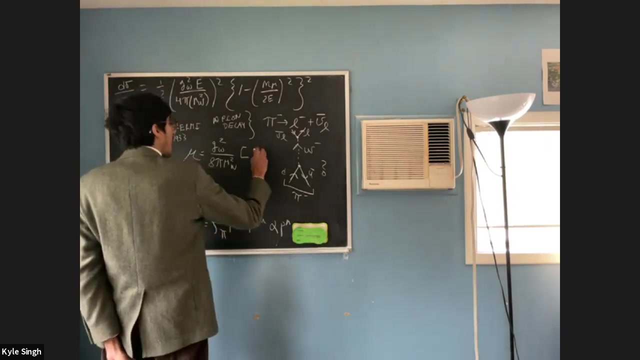 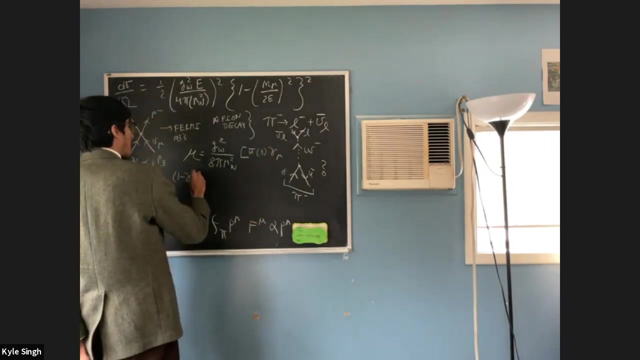 some P0 here, total P2 here. what's the P1?? P2? Yes, P0, lead government. Hence our immediateș. in other words, Tell the Okay. so let's write that down. So we have some like u bar of three. the outgoing particle gamma mu lowered times one minus. 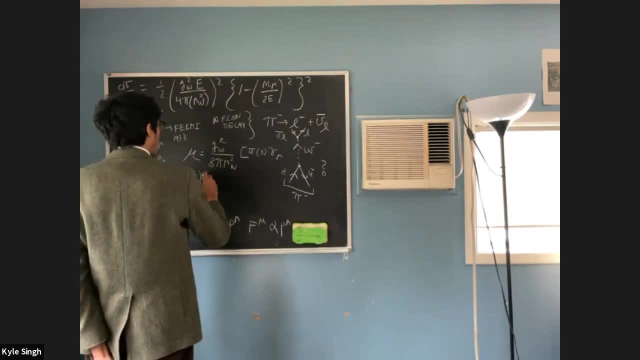 gamma five times what v, because it's an outgoing anti-neutrino v of two, all times f mu. That's just the amplitude. Okay, can I erase the board, or are we still okay? okay, so let's just write down the cross. 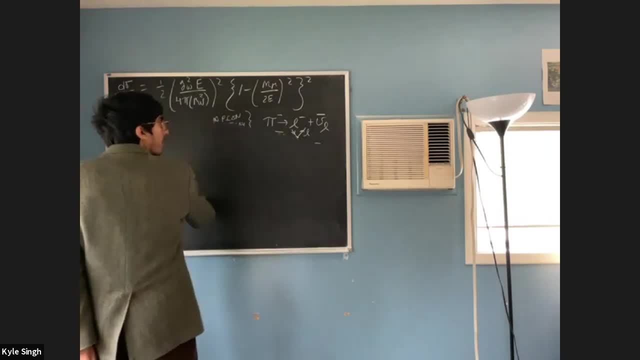 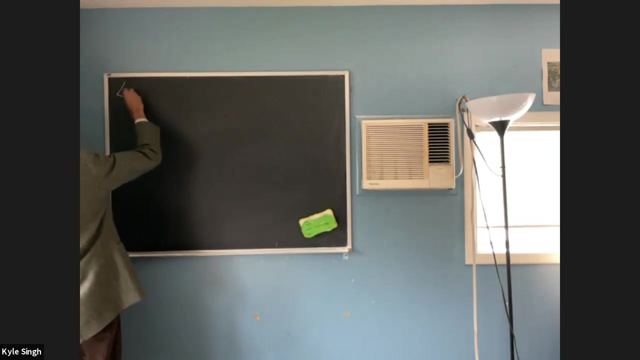 section. I'm not going to do the whole trace stuff, but you can work that out and then you can confirm: Okay, So you get the following expression: for mu squared, for m squared, So m squared becomes the following: So you should check this that you get gw over: mw. sorry, two mw. 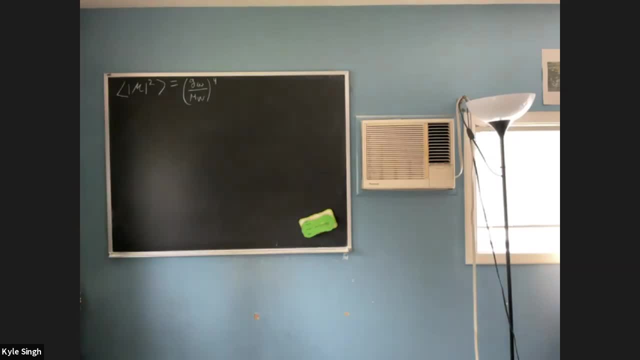 Okay, So that's the expression. Okay, So, that's the expression. Okay, So that's the expression. Okay, Okay, So that's the expression. So that's the expression. Okay, So that's the expression. Okay, So, f? pi squared ml squared mass of the lepton. m pi squared minus ml squared. 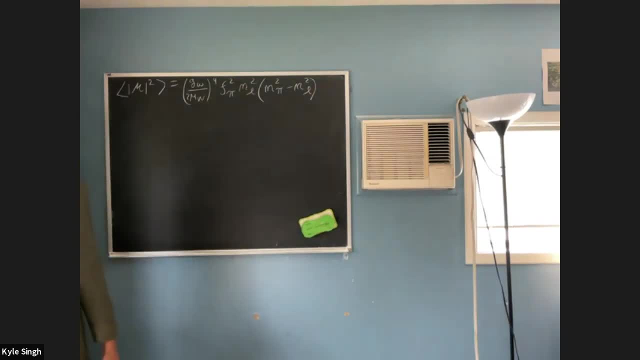 And so you should just confirm that. that's what you get, And we can write down the decay rate gamma. so any decay rate is defined in the following way: formula is just equal to p, so the absolute value of all the momenta over 8 pi h bar. 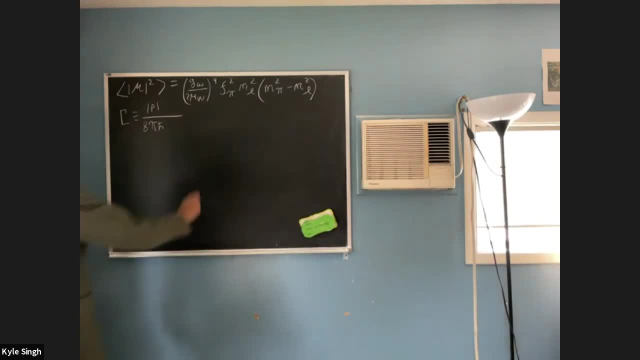 I'm only writing the h bars here, because it's an exact formula: m squared c times m squared, And so you can compute now the decay rate from this expression we just derived. And yeah, and you can write it down. I'm not going to write it down. 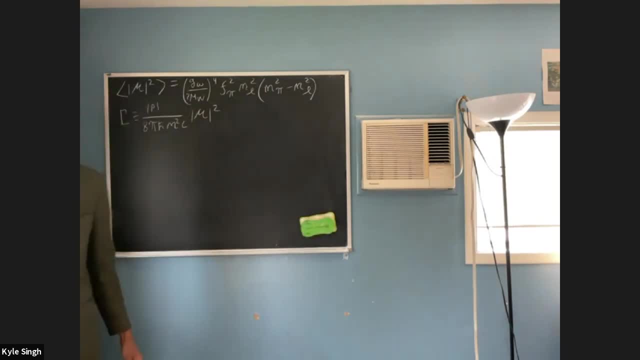 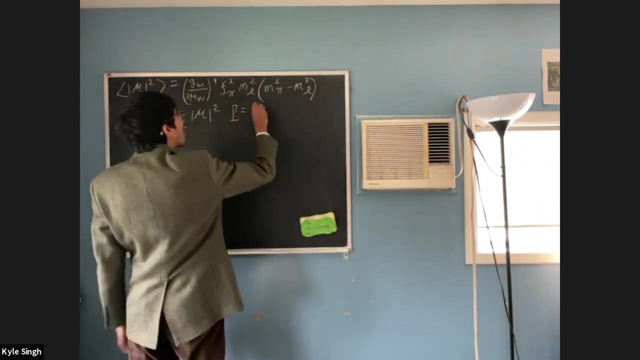 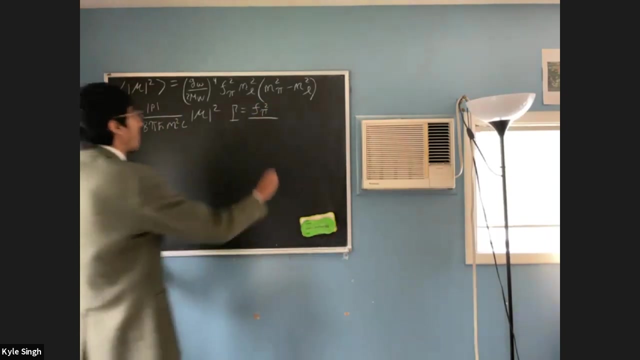 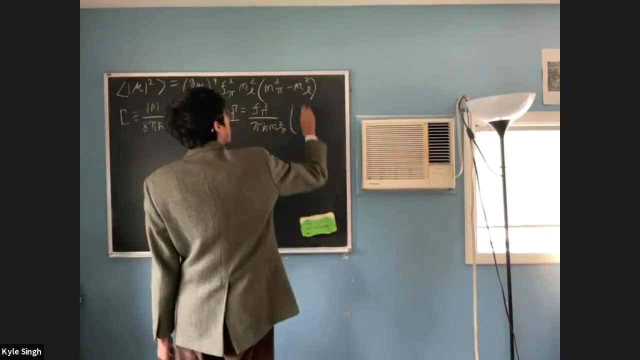 It's a simple thing, because I just gave you one square, Just plug it in. OK, I'll write it down for you anyway, just so we're on the same page. So f? pi squared over pi. h bar m pi squared. pw over 4 mw. over 4 ml squared. 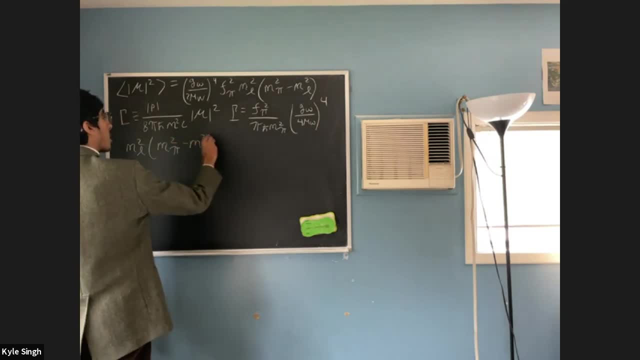 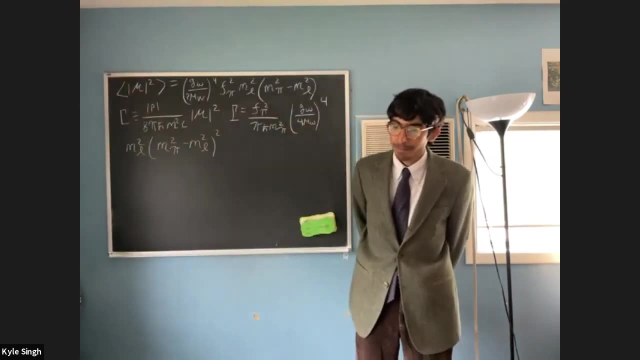 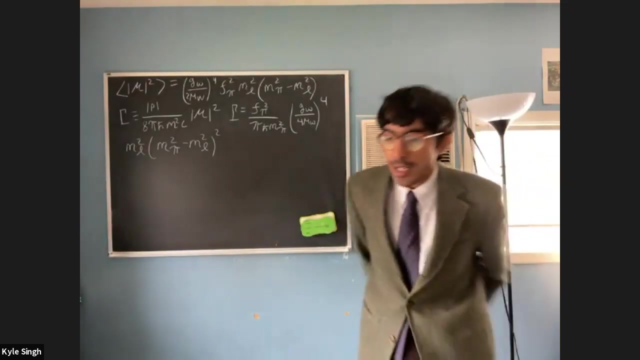 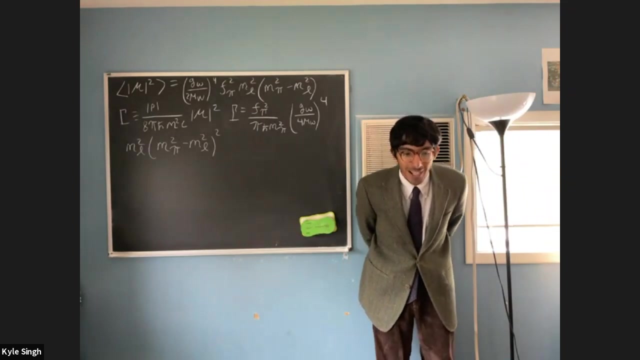 And that's the decay rate. So there's a very interesting thing that people calculate using these decay rates. You may have heard of the term branching ratio. You ever heard of that in your reading? OK, The branching ratio tells me sort of. 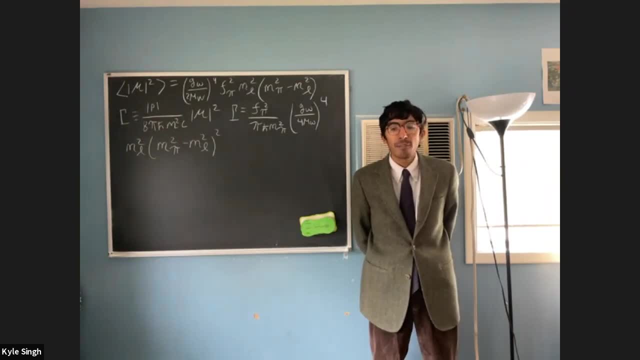 Part of the relationship between the decay rates of two different processes. So you're finding relationships between decay rates of two different processes in the hopes of learning more about the physics. So one very famous branching ratio that people sort of wrote down was gamma of this process. 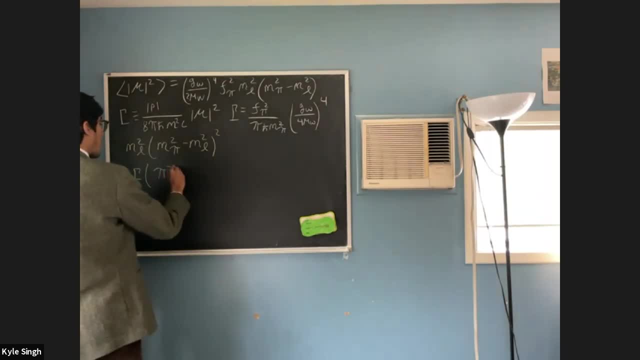 So pi minus what we just computed, Pi minus t, E minus plus electron neutrino, And they compare that to the decay rate of pi minus to a muon neutrino. Sorry, these should both be anti. I don't know why I keep doing that. 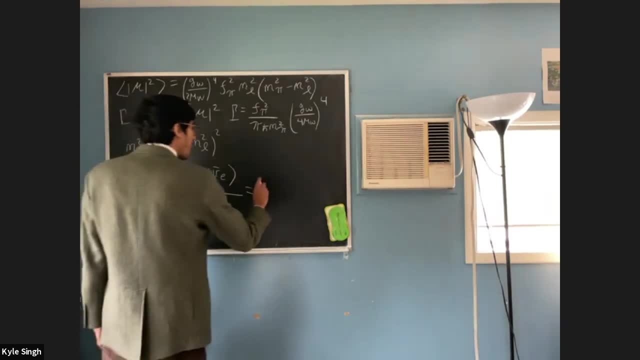 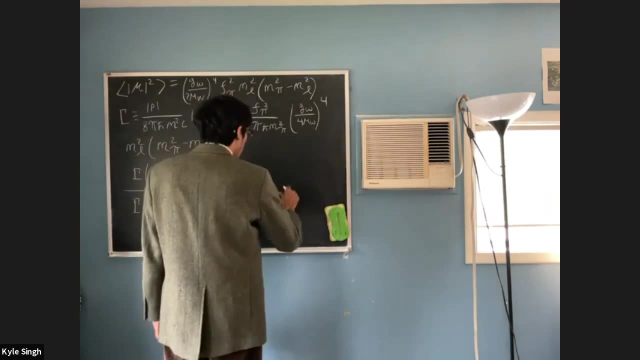 And, And This is called a branching ratio, and they found that this was 1.2, some number 1.24.. I have the number written down: 1.28 times 10 to the minus 4.. This is what theory predicted. 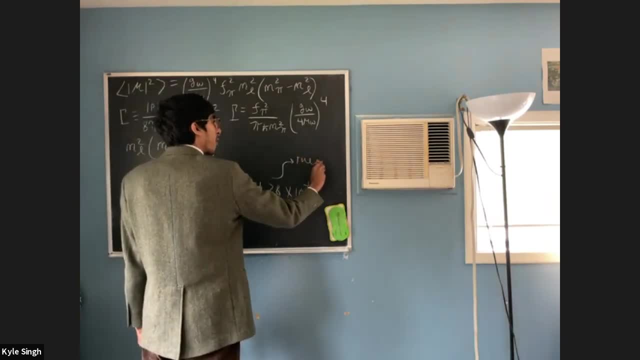 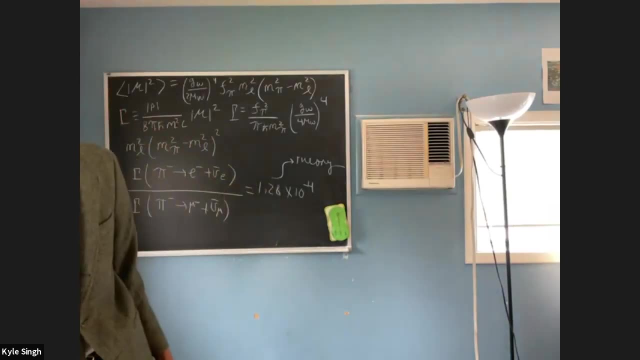 So this is theory in this branching ratio, from just computing the amplitudes and using all the numbers right instead of the letters, And except for this Right. So the experiment found that this branching ratio was pretty close, 1.23 plus or minus. 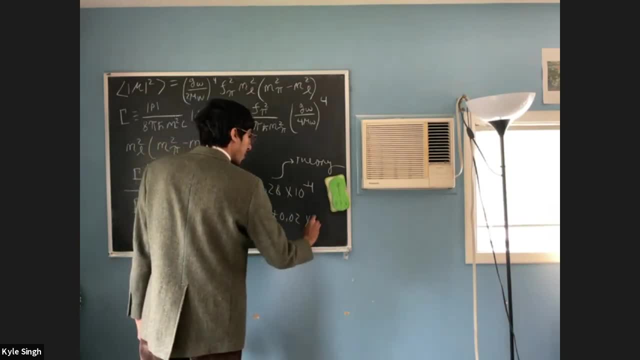 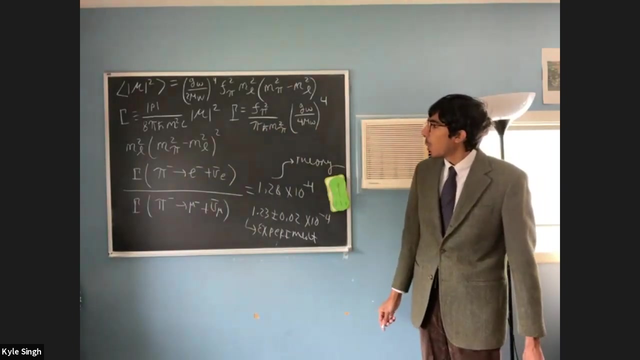 0.02 times 10 to the minus 4.. This is experiment. So they match pretty good, Pretty good match right. So now the question is is: why is there a discrepancy? So that's why that's what I leave to you. 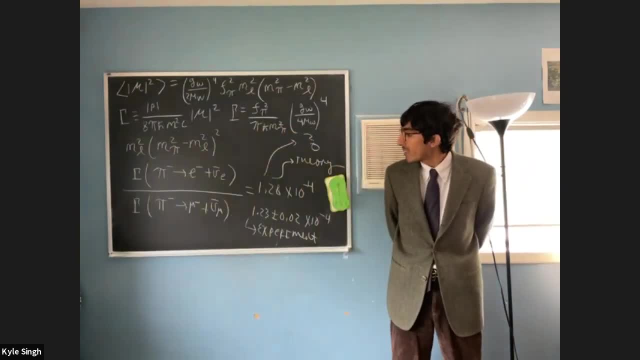 So why do you think there is a discrepancy between the two processes? In other words, what is this branching ratio telling me? Does anyone have any inkling of this? And this is kind of an interesting point to understand because it sort of will help you. 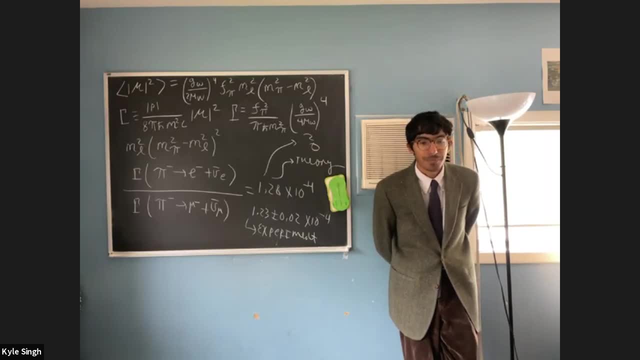 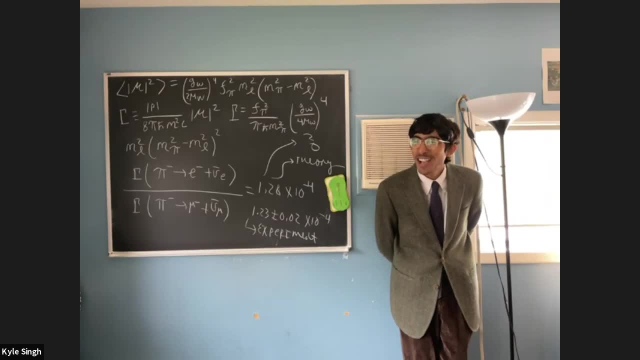 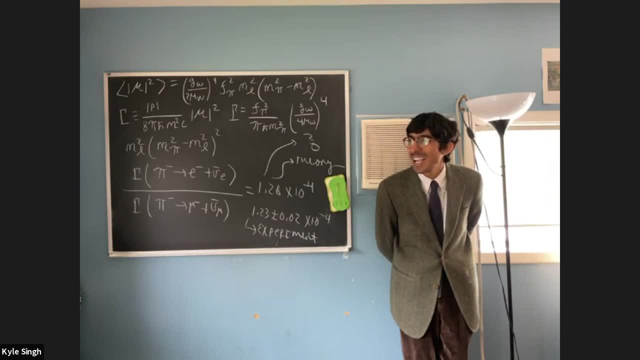 I don't have a pion. I don't have a pion. Do you know what it's going to decay into Beforehand? No, There's different probabilities. right that it might go to an electron or it might go to a muon. 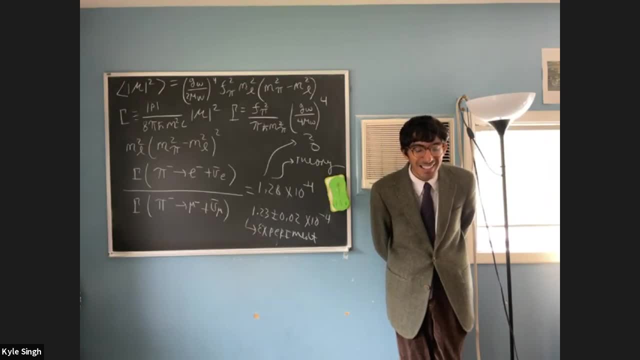 That's the beauty of this. That's for this quantum mechanics stuff comes in And this tells you what process is more likely Right Than the other Right. So that's what this is, It's telling me: is it more likely for the pion to go to an electron or a muon? 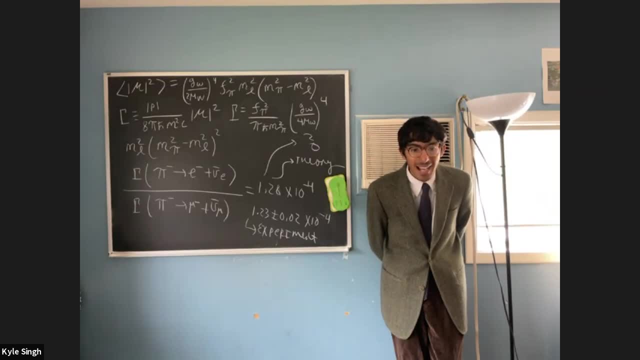 Muon, Muon, exactly, Exactly, Okay. so that's a good thing. So you can always kind of do these little things. You can compute two different amplitudes. Of course, the masses are going to be different. That's going to impact the final result. 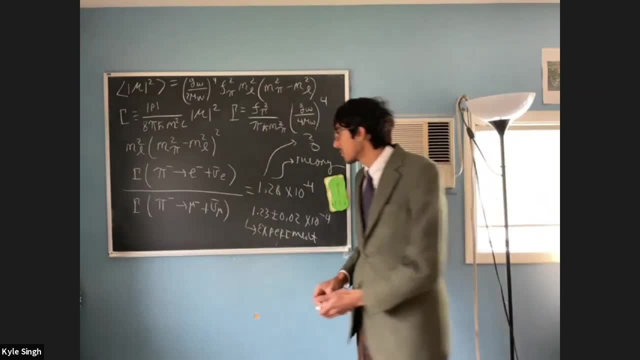 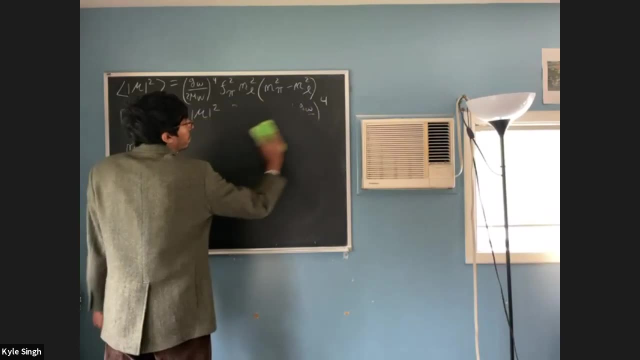 And it's subtle, but it's not that subtle. So that's a nice little exercise. Take two random weak interactions, compute the amplitude and see the branching ratio and see if you can get it to match. That's kind of a fun exercise to do. 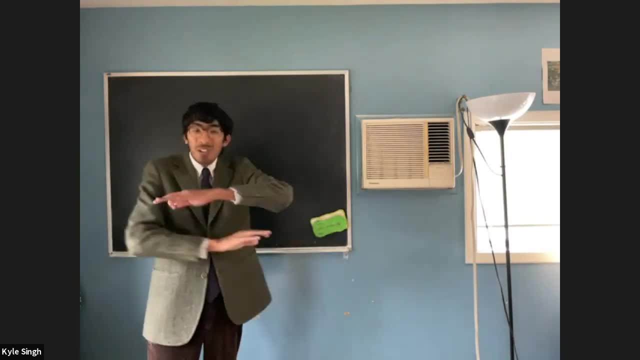 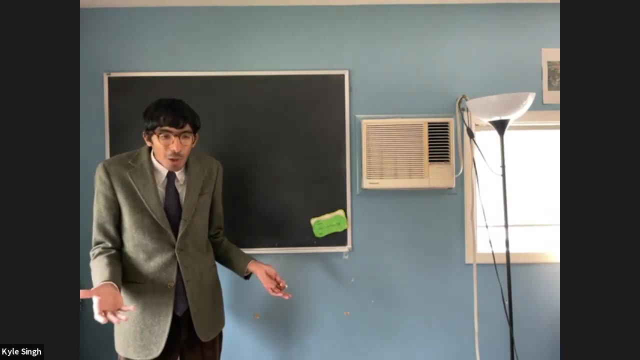 You may even discover that some processes are totally suppressed. You know, this ratio was still kind of close. It's almost close to zero, basically, Or close to one. sorry, No, Yeah, it was close. It was like 1.28 times 10 to the minus four. 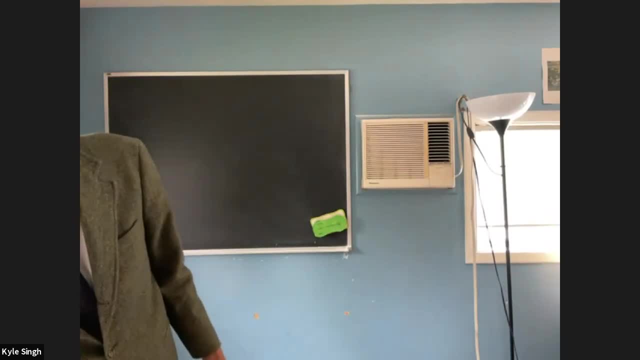 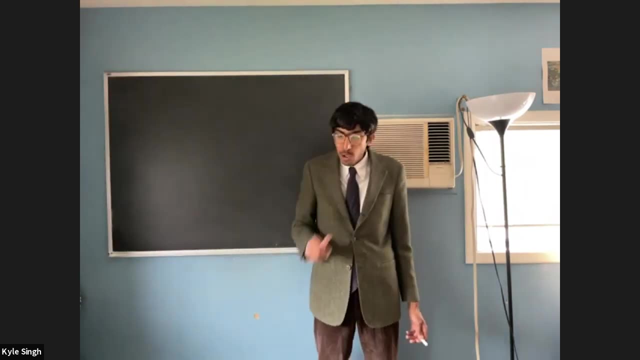 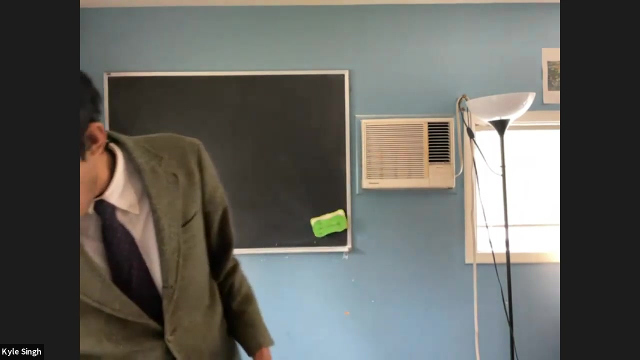 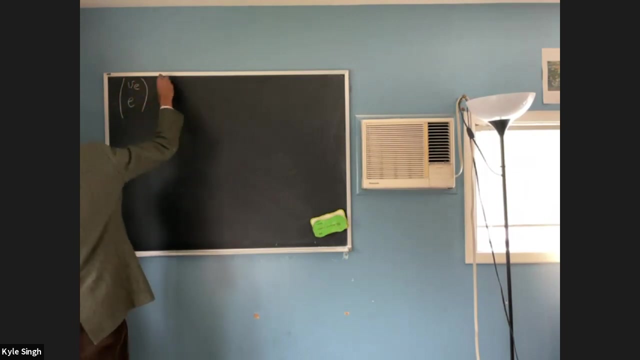 It was pretty small. Okay, great, Let's talk a little bit about the weak interactions of quarks. Okay, let's dig into that a little bit. So if I have leptons, so I have an E electron neutrino, I have a muon, I have a muon neutrino, I have a tau, I have a tau neutrino. So three generations of leptons. 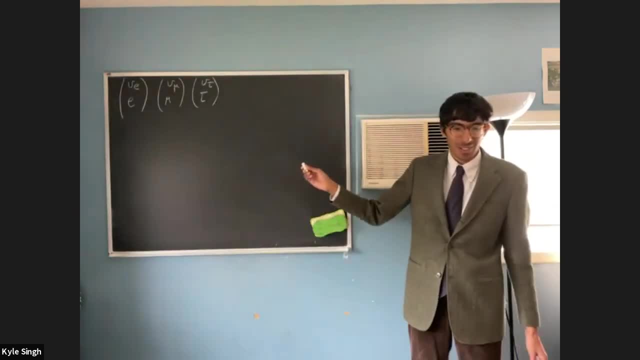 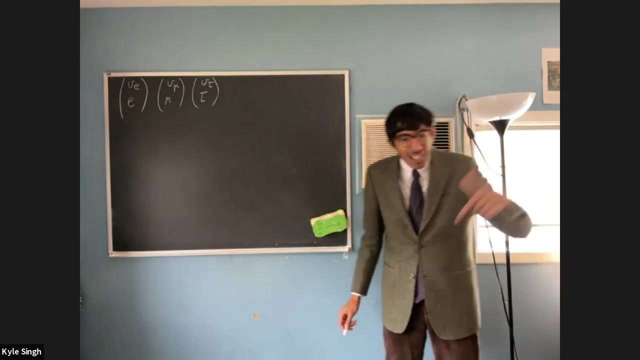 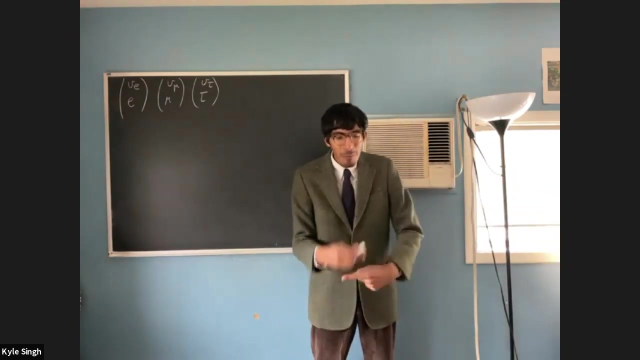 Okay, Oh, we call these generations. Okay. that's a particle physics word. You may have seen that word. so In the weak interaction between the leptons it's all in the family. An electron can only go to an electron neutrino. A muon can only go to a muon neutrino. A tau can only go to a tau neutrino. There's no mixing. 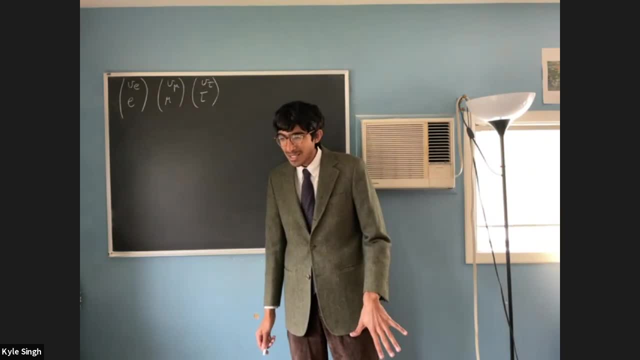 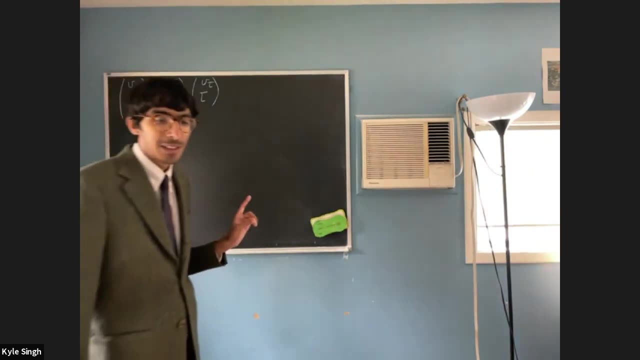 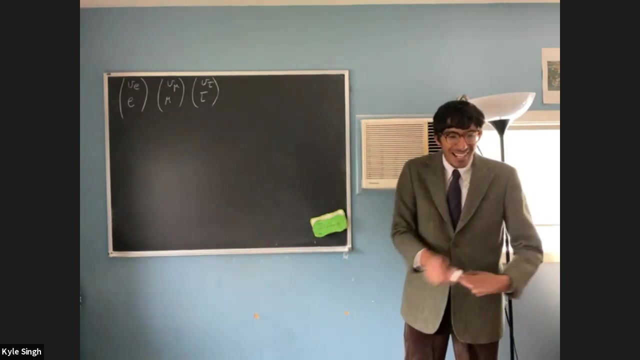 Okay, So leptons couple to the W bosons in the same generation. Get that? That's a nice little thing. Quarks are runs. They don't do that. They mix and they couple with each other. and we have to see. See, this is where these angles are going to come in. 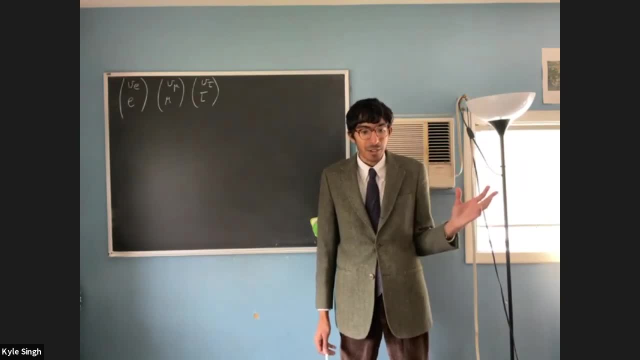 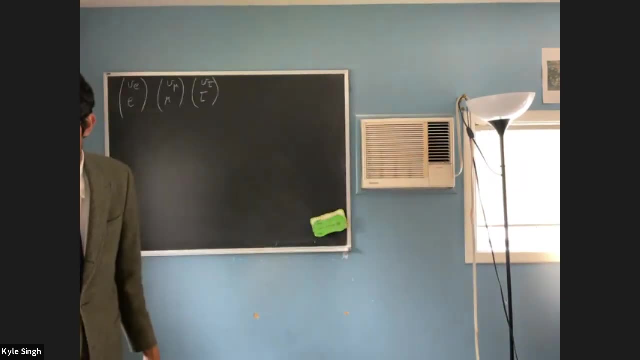 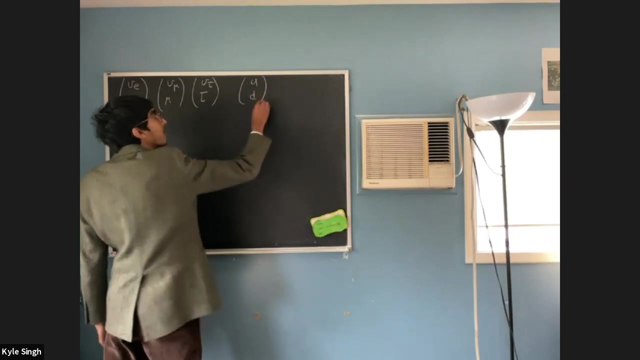 Or these datas. They tell us how to mix these different things. They give us a little parameter to multiply by. That alters the amplitude. Okay, So we have three generations of quarks up-down. That's the first generation, And by generation it really means they're organized by mass, Right By mass. 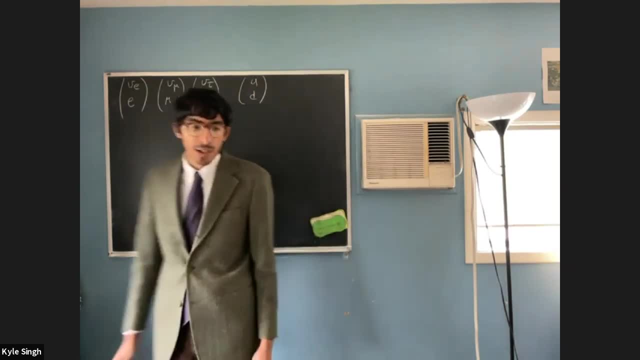 So we have three generations of quarks: Up-down, That's the first generation, And by generation it really means they're organized by mass Right, By mass- Yes, that's what we mean by generation: Charm, strange and top-up. 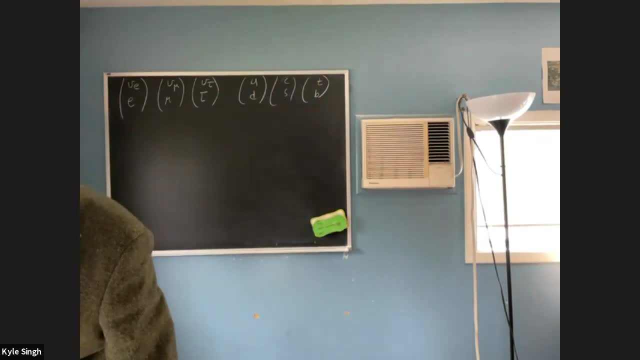 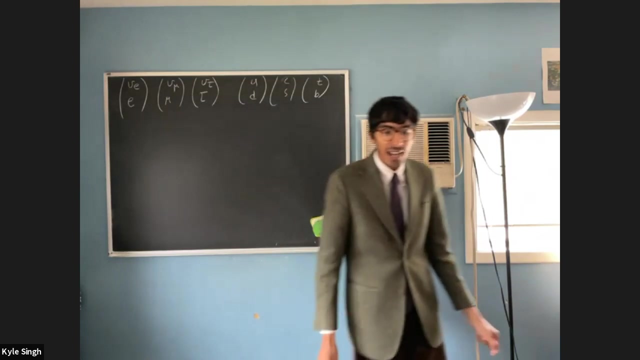 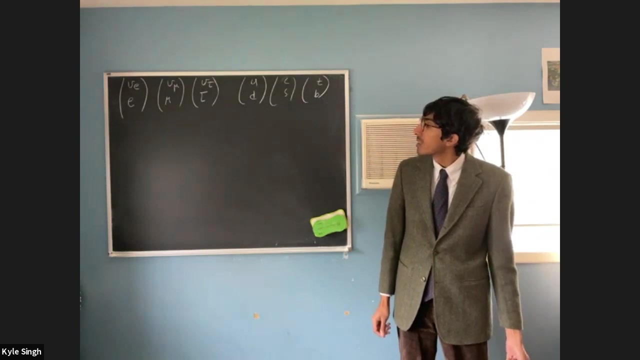 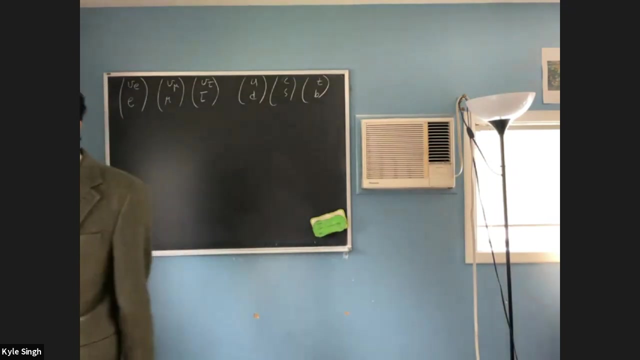 These are the three generations of quarks. Okay, so people started to realize that the quarks and the weak interaction did not stay all in the family, so to speak, right, That their various processes were intergenerational. And so there was a great physicist in 1963.. 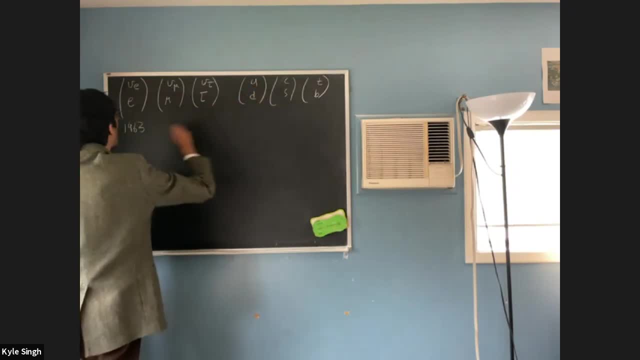 So in 1963, we only knew that up down and strange quarks existed. So we only had up down and strange quarks And his name was Khabibov, who Galman talks about a lot actually. 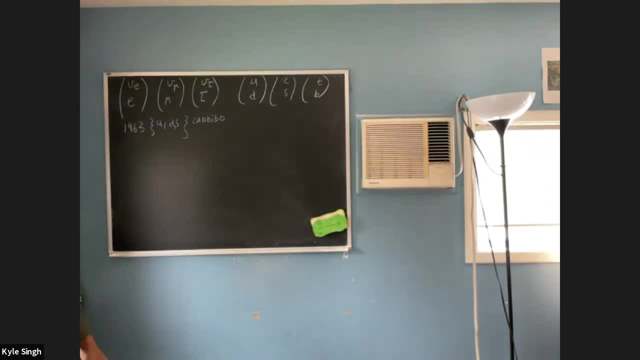 And so Khabibov postulated that if I had the process down goes to up plus W plus- sorry, W minus- that it would carry a factor of cosine beta, We'll put a little subscript C, And if S goes to up plus W minus, 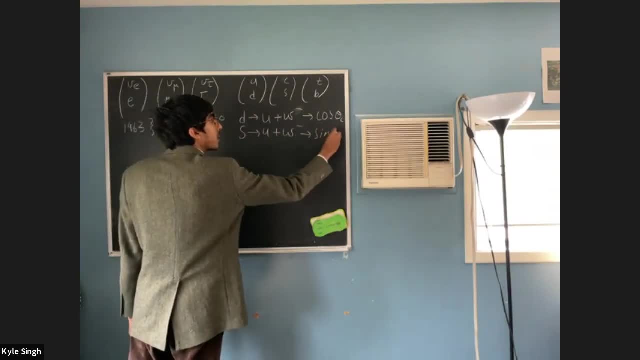 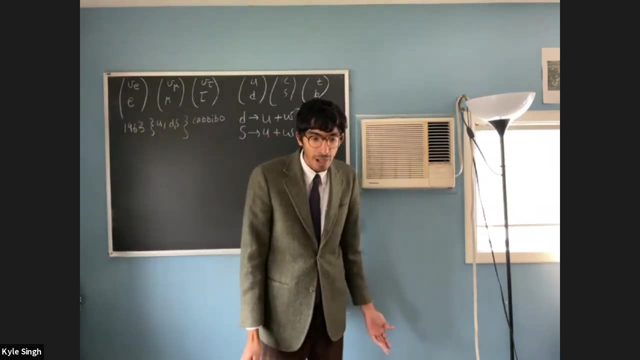 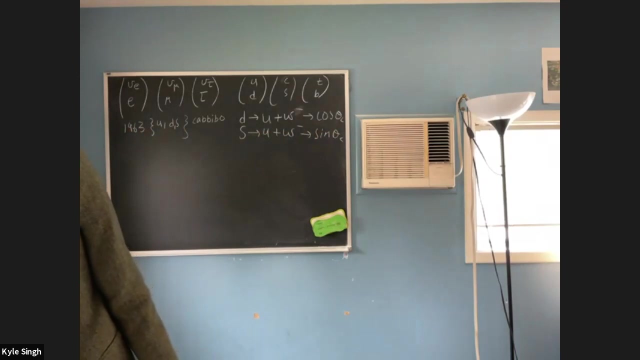 so now intergenerational. then I get sine beta C. Now, in effect, sine beta, cosine beta, is just multiplying by some number. It's just an extra factor that's gonna take us from one to the other. Okay, so the vertex factors now. 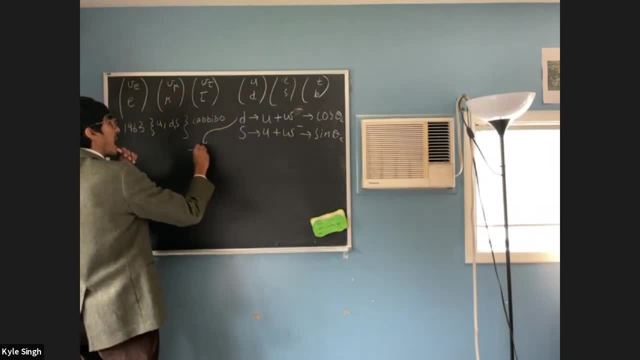 so this vertex factor is just minus I GW over two root two. gamma mu one. minus gamma five cosine theta C. So that's the new vertex factor, And then this one is the same thing. So minus I GW, two root two. 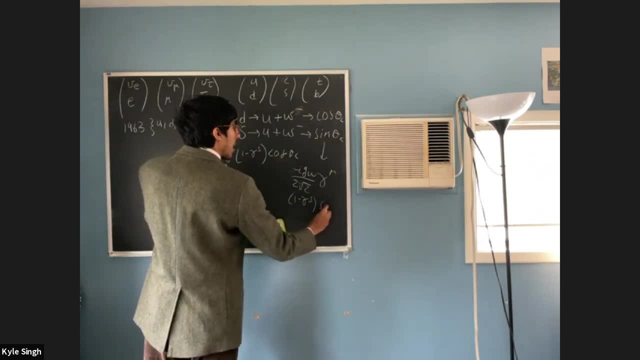 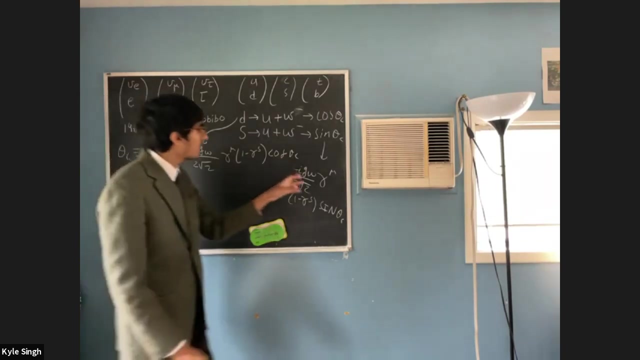 gamma mu one minus gamma five sine beta C. okay, So that's what Khabibov postulated And experimentally, this angle, this Khabibov angle, is 13.1 degrees. Yeah, so that's where the C Khabibov? 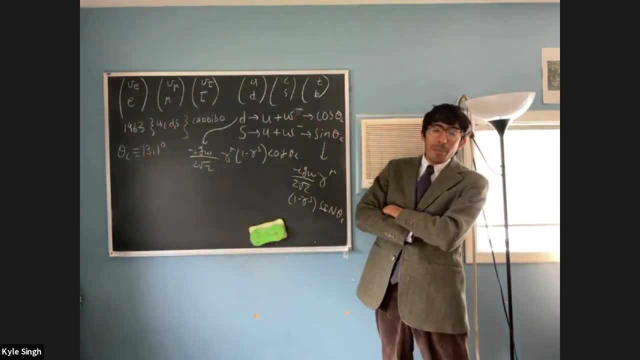 So this started working for many, many processes. It was like, wow, you know, you add this silly new parameter and the amplitudes work and you can account for the intergenerational mixing of the quarks and the weak interaction. until one day some experimenter tried the following: 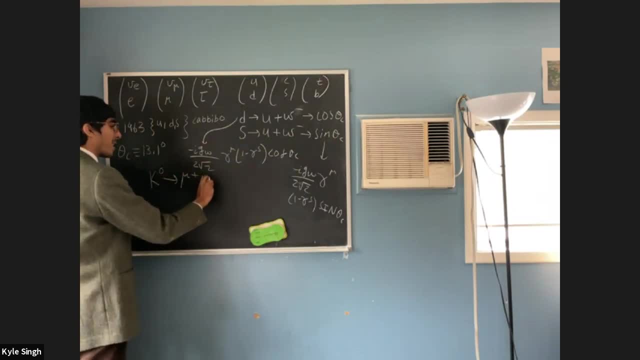 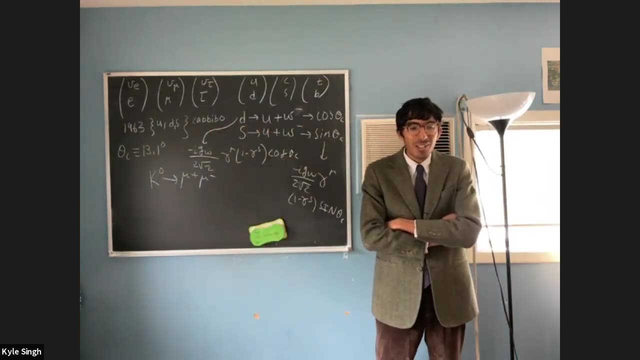 They decayed a K naught until a mu plus, mu minus, And they found that the Khabibov prescription gave you the wrong answer by a factor of 10. It seemed as though you know, because you see, this is why. 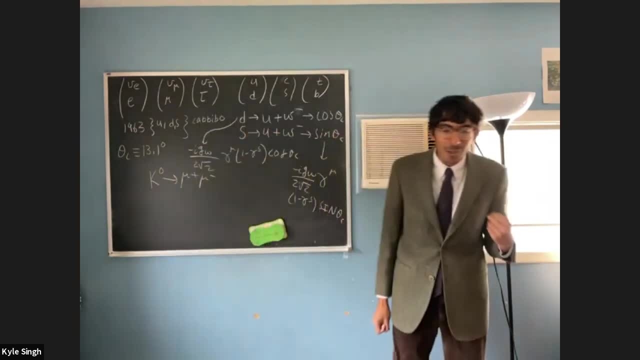 It seemed as though you know because you see. this is why It seemed as though you know, because you see. this is why is why? this is you know. when people say in science, okay, what are the truths of science, i say: 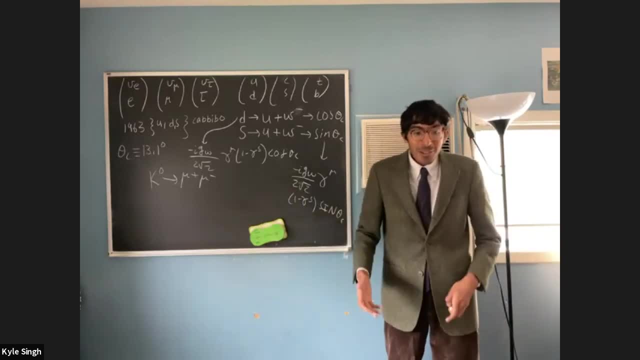 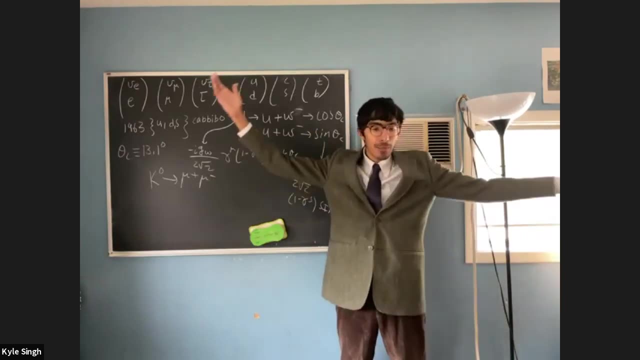 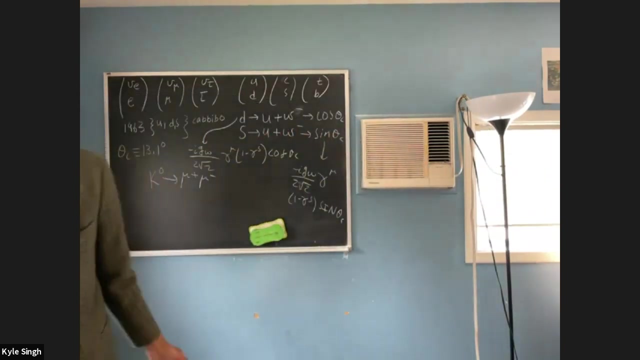 absolutely nothing because. because so they're doing all these experiments, capito's theory works. i mean, look it works, it's good they do this random thing and it's completely off. so they had to come up with some solution for this. okay, so they found that actually, the amplitude was not proportional to a factor of sign times. 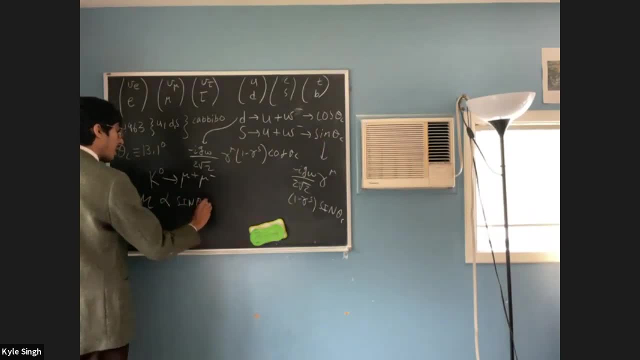 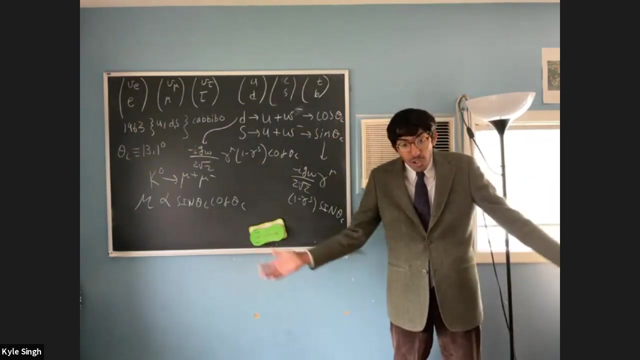 cosine theta times. this could be going though. so who came to the rescue in 1970? Sheldon Glashow, you can tell. Glashow did a lot of incredible work at this study, and if you look at the bottom of this graph you can see that. 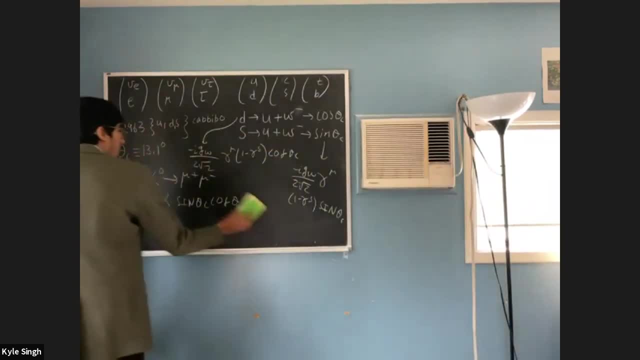 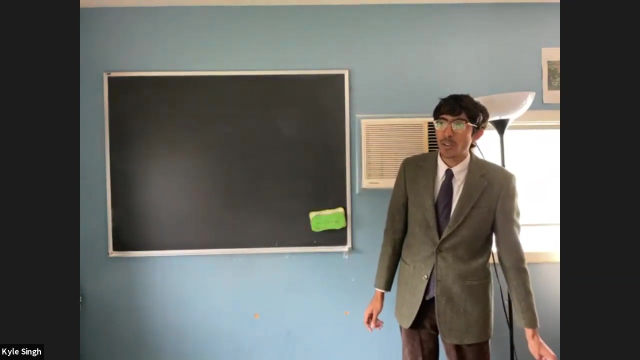 time. i mean, there were many people, but so glashow comes up with the solution to this now? okay, you have to keep this in perspective. people were still on the fence at this time, whether the weak interaction was axial vector, was axial coupling, as jetta knows, people were still on the fence at this. 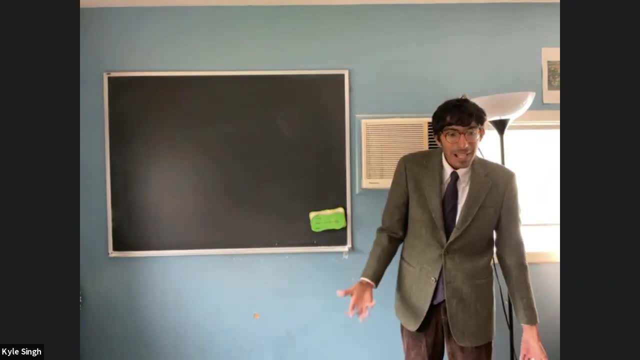 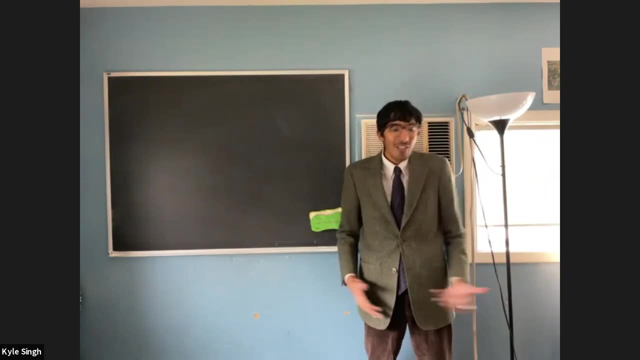 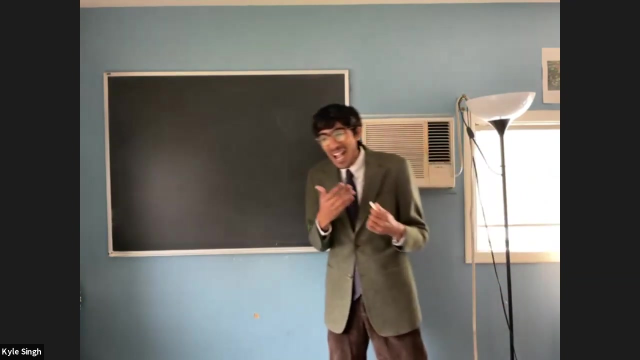 time whether quarks existed, right like people. this is not so. there was. the whole weak interaction program felt a little speculative at this point, even though the experiment matched theory. but people didn't really know if quarks were a thing we didn't. they didn't know if what was actually 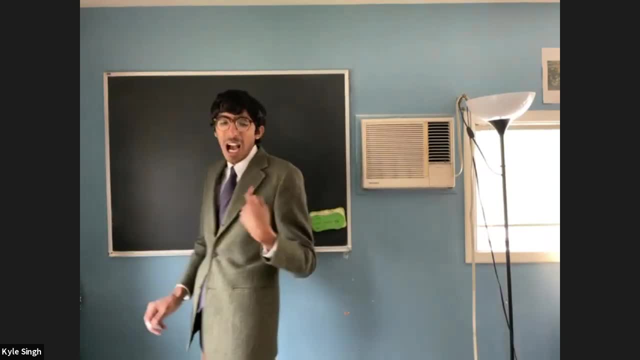 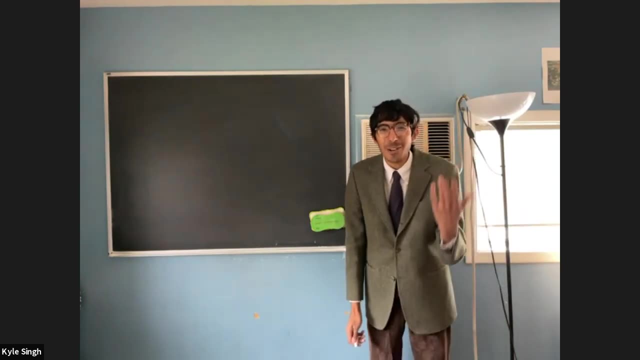 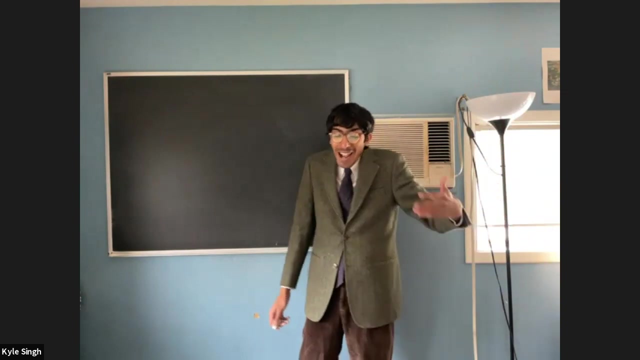 accounted for was this phenomenon. so a lot of speculation. and then, on top of that, now you have this issue, and when i tell you glashow's solution, people were even more skeptical. what was glashow's solution? he had introduced a new quark, so his solution was even more crazy. uh, and all of these people working on? 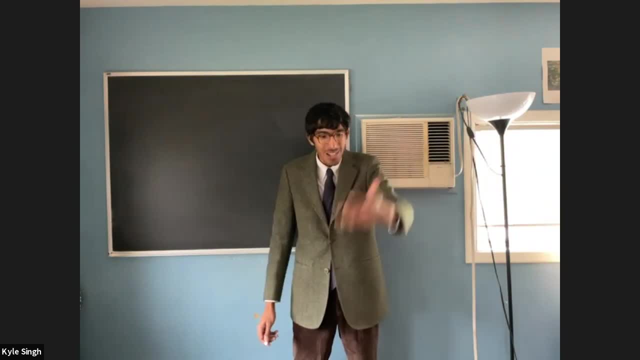 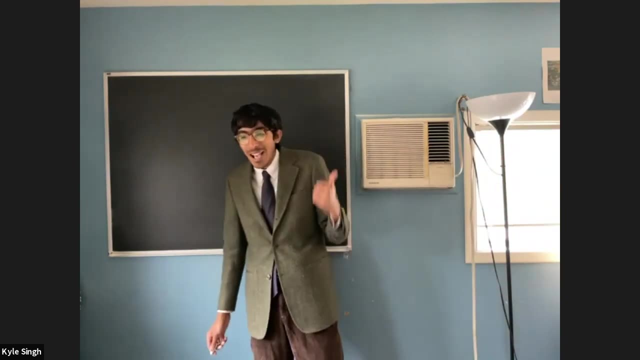 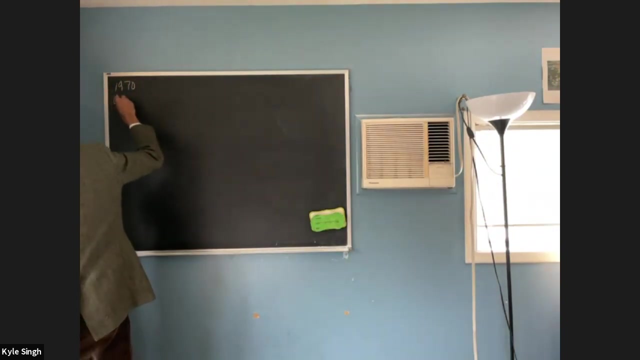 the weak interaction led by glashow and salam and weinberg. they seem a little bit on the fence because, uh, he had to introduce a new quark. so glashow's solution in 1970. so you can read this paper: uh, it's called the gim mechanism, so gim mechanism and uh, quote, unquote. i. 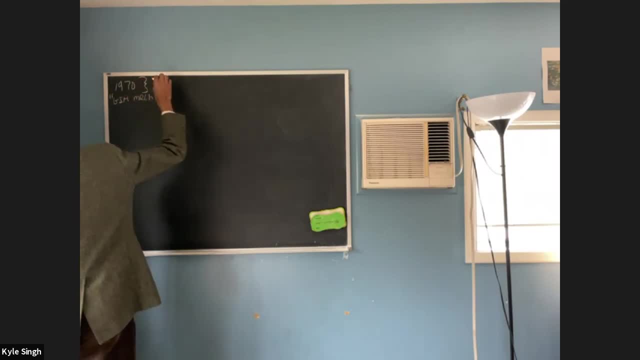 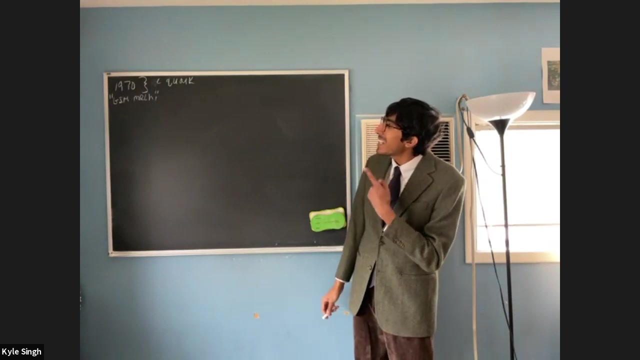 just glashow was the first author and it's called uh, and they introduced the top quark. so the top quark was introduced. oh sorry, not the, not, not the top court, the charm quark. oh my god, sorry. so this was four years. okay, so in 1970 was four years before they actually discovered the charm quark. 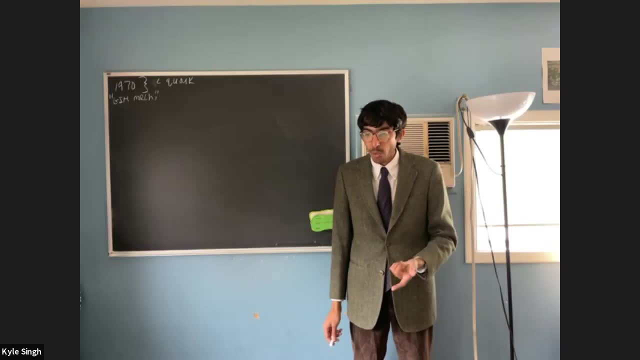 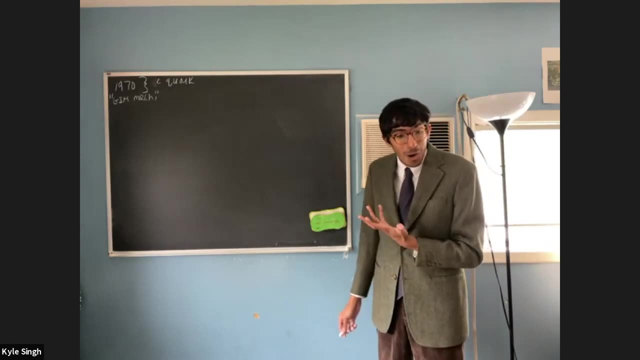 okay, and they predicted the mass and i'm going to show you the right vertex factors, the right coupling. but can you imagine they were left on the hook? if this thing was real when they found it, can you imagine the relief? yes, this works and there's a special name, if you look. 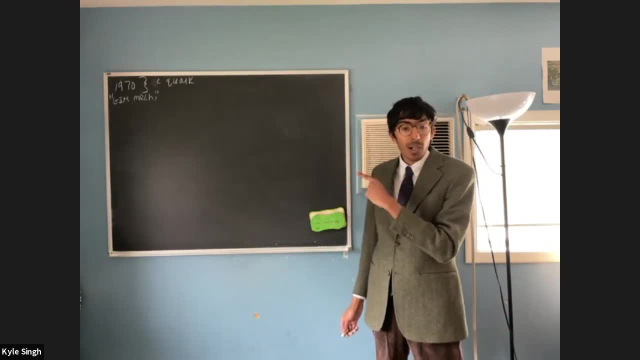 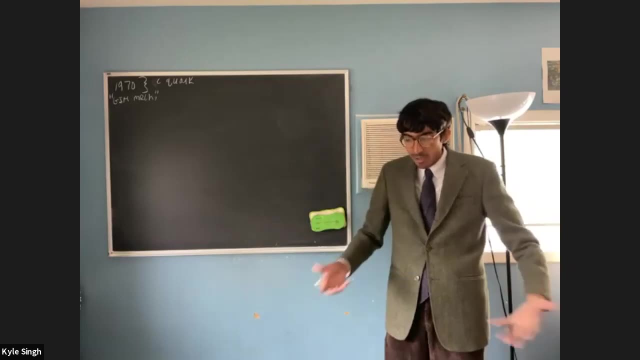 it up. 1974, when they found the charm quark, they were left on the hook. if they found it, you could was referred to as the November Revolution, because that's when they found all of these quarks, all of the weakened the whole sort of apparatus of the standard model, and this was 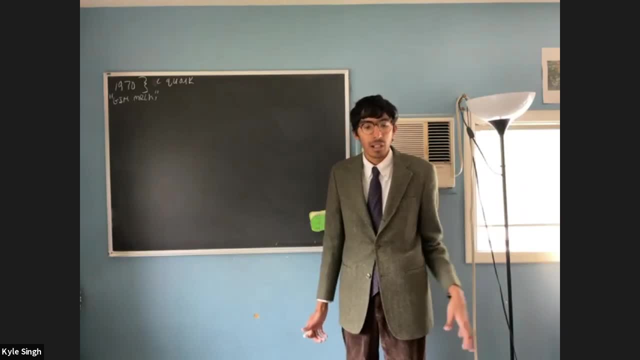 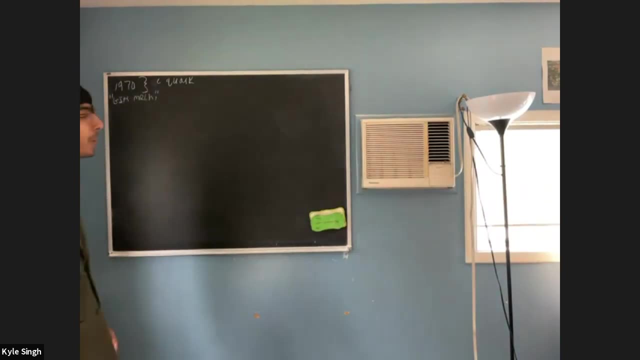 all at the LHC, not the LHC. sorry, it was all at CERN. they didn't have an LHC at that time. they had a smaller collider, but it was all at CERN. okay, so let's write down the right coupling. it seems trivial, but at the time it was introducing a new particle. that's not really trivial when you. 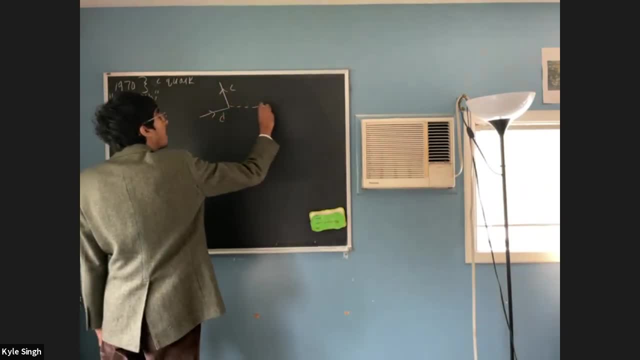 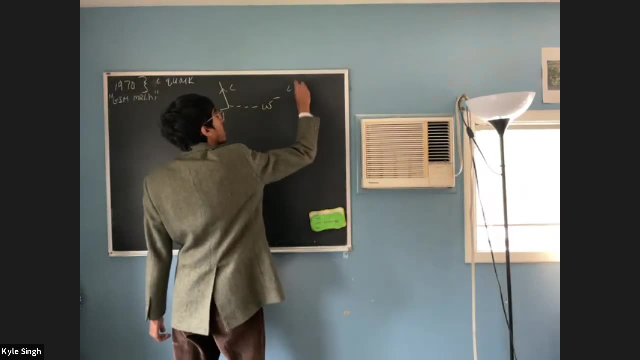 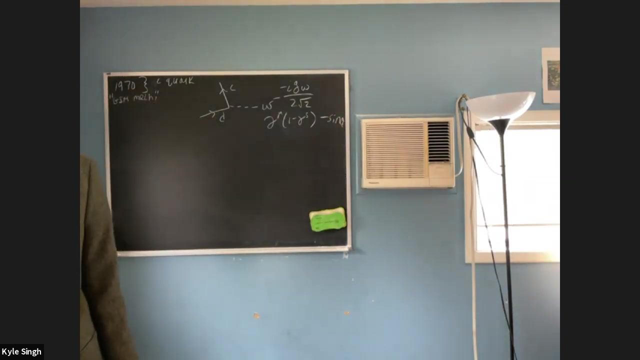 don't even know if the quarks really exist. so again it's coupled to W minus and now we just get a minus. I W two over root two gamma mu. one minus gamma five, but minus sine theta C. okay, so now mu m is proportional to minus sine. 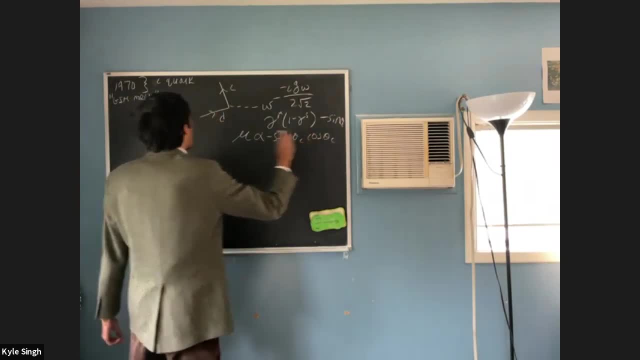 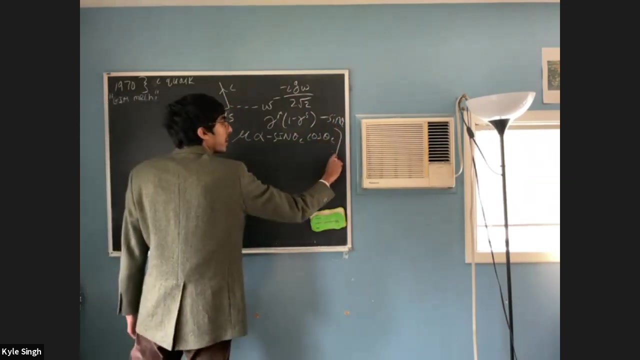 C, theta C, cosine, theta C. and if you just couple this down to a strange quark, now you get a factor of cosine instead of minus sine. so we'll just write this as upper strange and we'll put this as sine, theta or cosine. that's the couple. oh sorry, not up down. 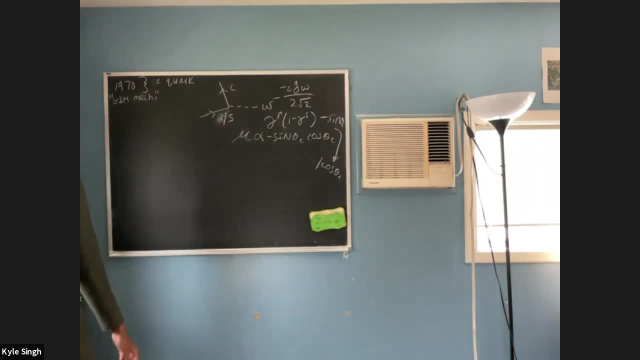 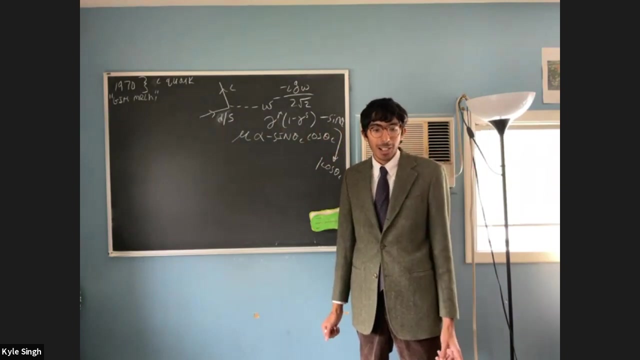 because they all have different masses, so it's very important to distinguish them. okay, this is kind of a big deal. I mean, this was crazy. at 1970, people thought this was crazy. first of all, we don't know if these exist. now you're just saying there's another. 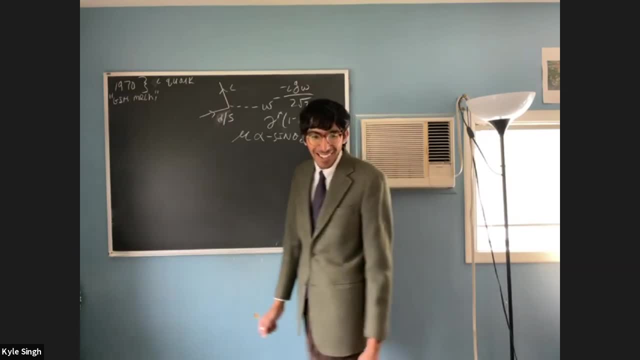 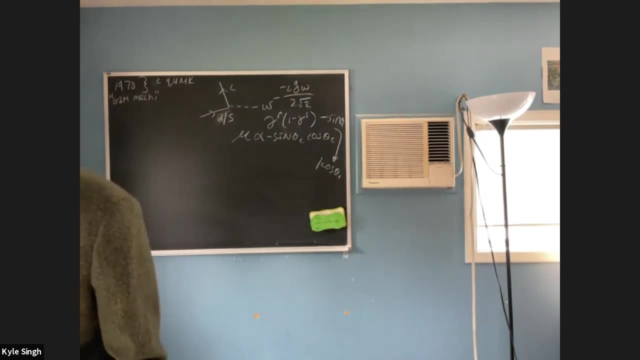 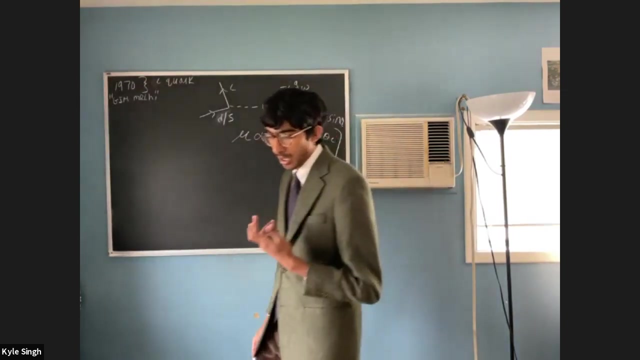 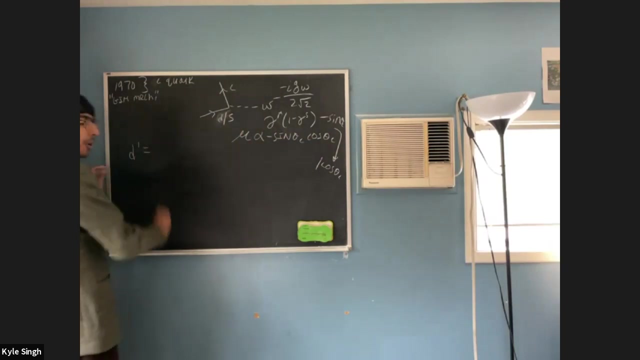 seem like string theory. okay, okay, great, okay, so we can go. now we can go between sort of generations of quarks. so I'm going to erase, I'll keep it. so if I have some D' some new quark, I can now write the new quark as a superposition of the old quarks: D cosine, theta C plus S sine theta, C plus. this is just D косine theta without Medic, and that's past. the thing is, if we fucking do this, 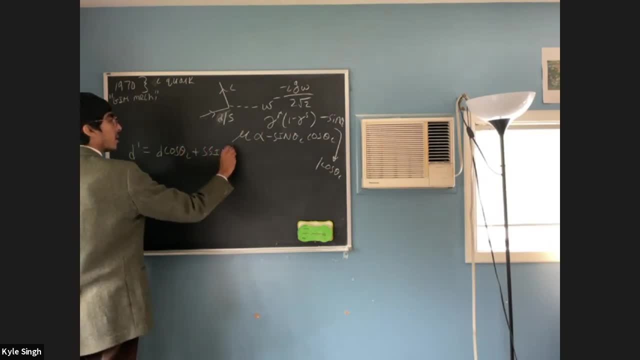 the thing is. the thing is, if we fine tune the equation we still get like a new quark. but then, as we're like, oh so we have some użyctiou s sine theta c, And if I have some s from, I can write this as sorry. 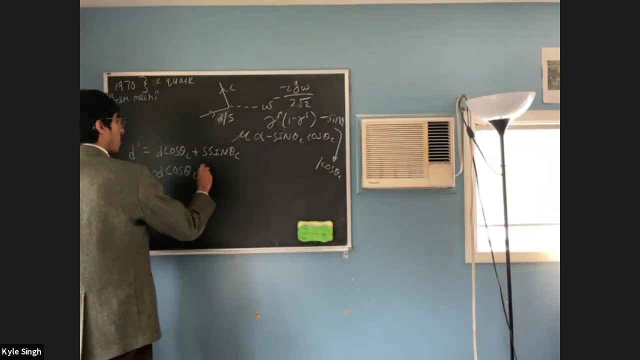 this should yeah. minus d cosine theta c plus s sine theta c. Well, no, this should no. sorry, sorry, sorry. This should be minus d sine theta c plus s cosine theta c. I can put this into a matrix. 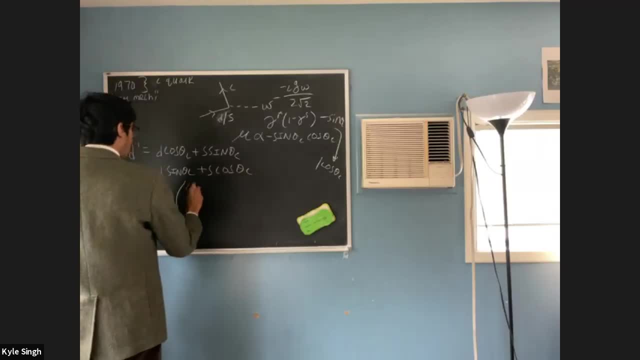 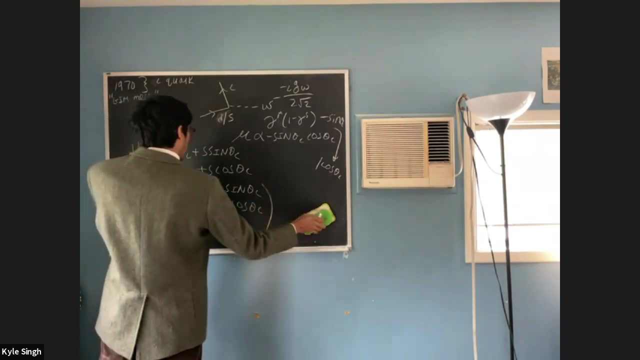 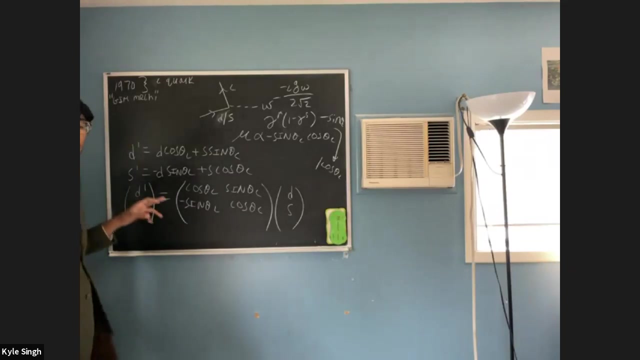 This will be useful. So I have the following matrix equation: OK, So I can put this into some matrix that looks like this Matrix equation. And so now this d prime and s prime are referred to as Kibbebo rotated states. 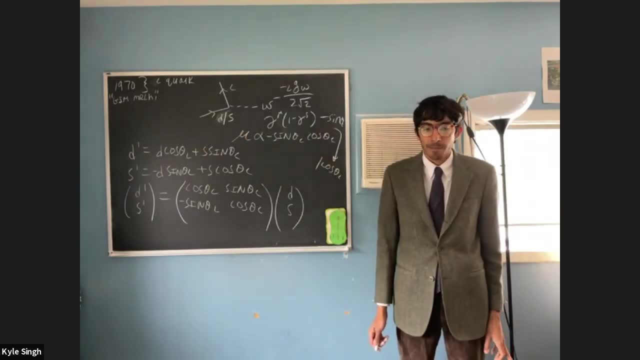 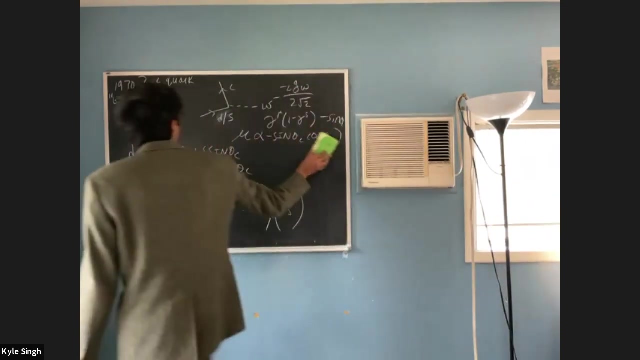 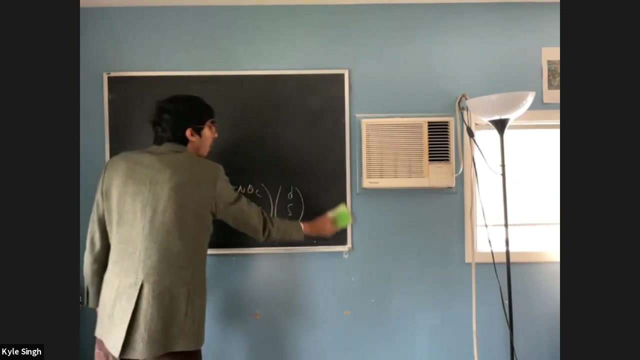 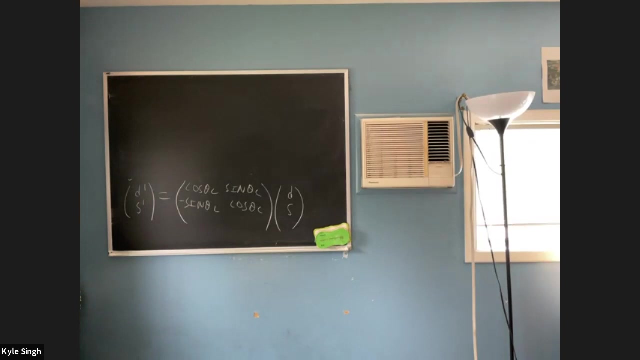 They're superpositions of quark states, They're Kibbebo rotated states. They're not actual quarks right Right Now. so this argument, so this is for down in strange quarks. OK, And two, three, four. 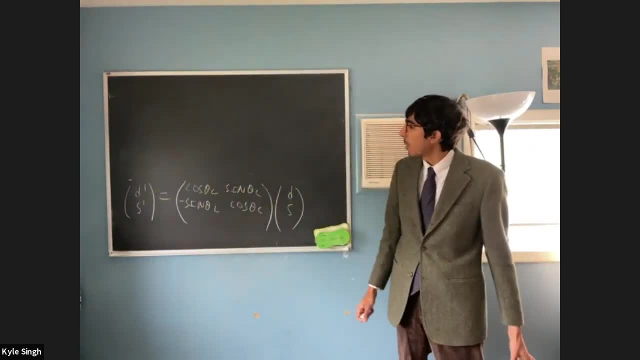 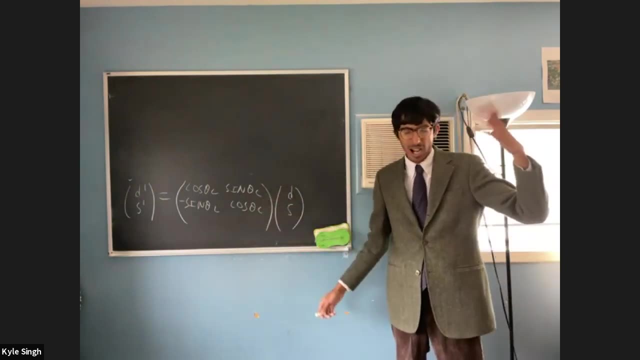 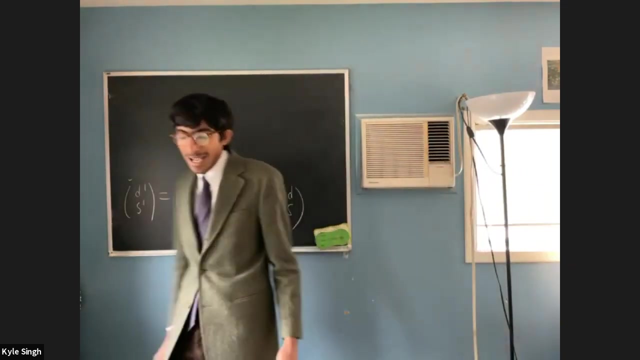 Two Japanese physicists, Kobayashi and Masakawa, generalized this argument to show the mixing of all quarks, and this is the Kobayashi-Masakawa matrix. it's some long thing, I'm not going to write it down, but it's just all of the different combinations. it's not so important and of. 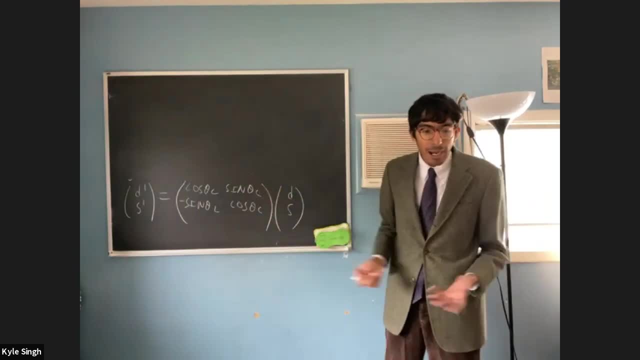 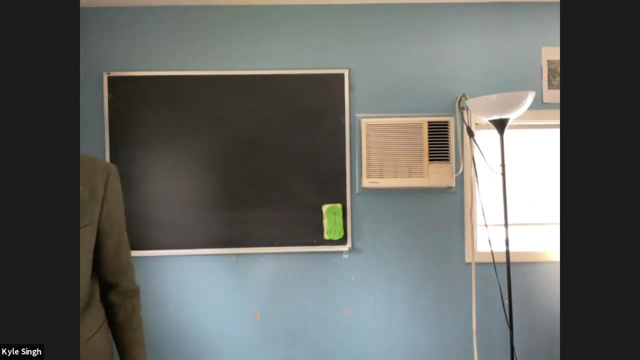 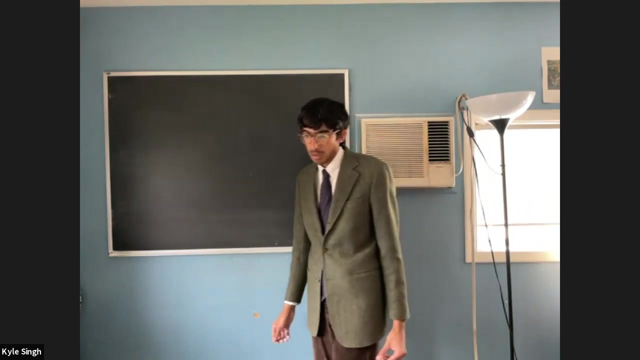 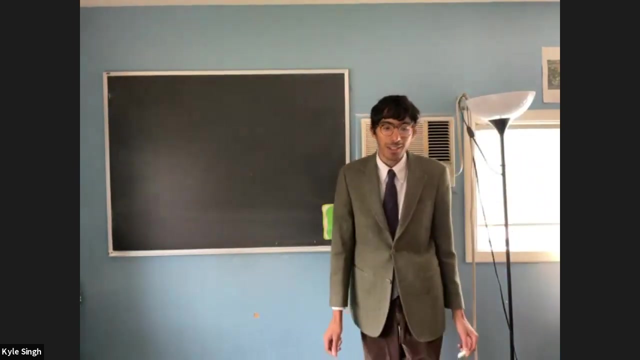 course, each combination gives you a different number, different parameter. okay, so that's the, that's the big thing. so the GIM mechanism. I forget the other two guys- Glashow. okay, so 1961, which I should. I should have had you read this paper, but I'll send it to you guys. 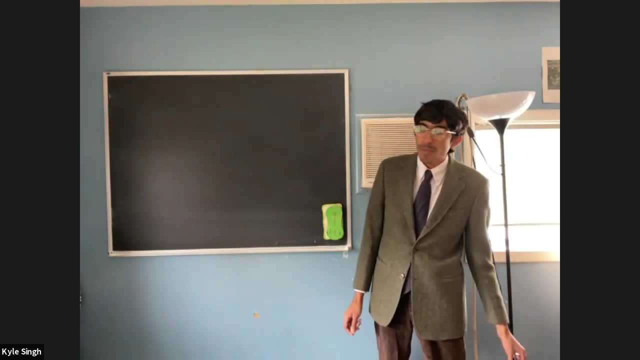 1961, Glashow writes the first paper postulating the idea of electroweak unification. who gave him this idea? I watched an interview of Sheldon Glashow. you should watch it. amazing interview with Lawrence Crass, the only interview I know of him on YouTube. it's not really. he's still alive. 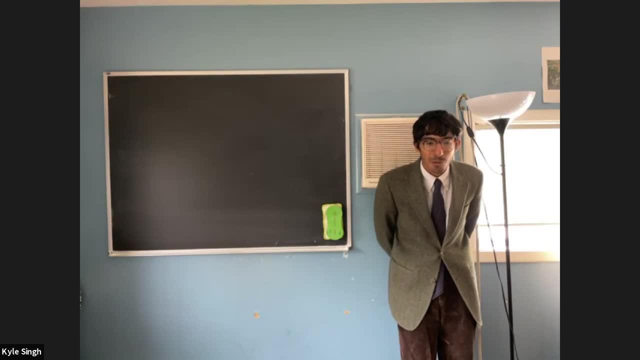 actually all these guys are pretty much alive, except Salam, which is kind of cool. so- and he's talking about how he gets the idea- so Lawrence Crass, so he goes. so he calls him Shelley, so I guess they're on a personal basis. he goes, Shelley, how did you get the idea for? 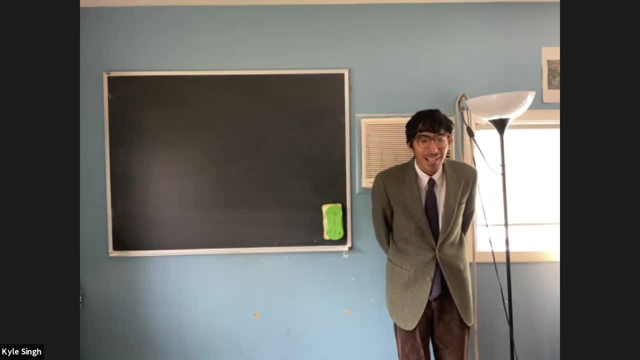 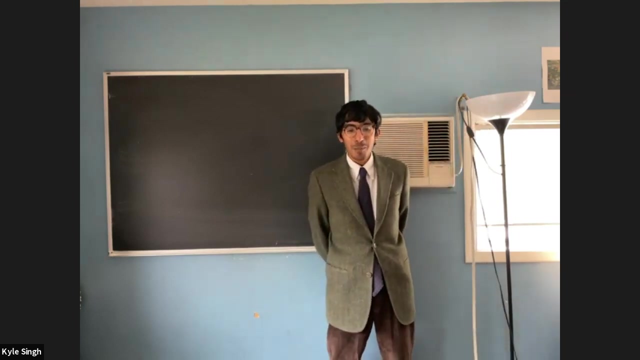 electroweak unification. right, that seems like such a. he said it wasn't my idea. he said it wasn't my idea and Lawrence goes whose idea? he said it was Schwinger's idea. I was shocked by this, so he goes. so Sheldon Glashow was a PhD student of Julian Schwinger at Harvard. 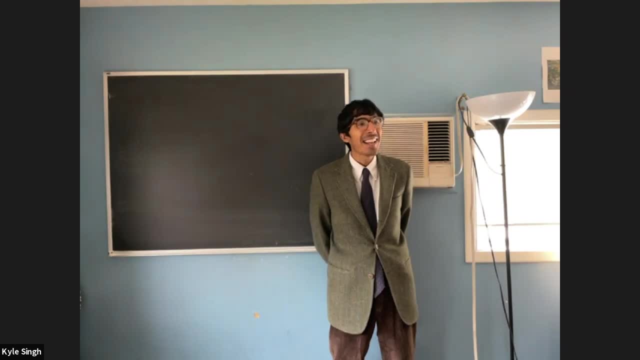 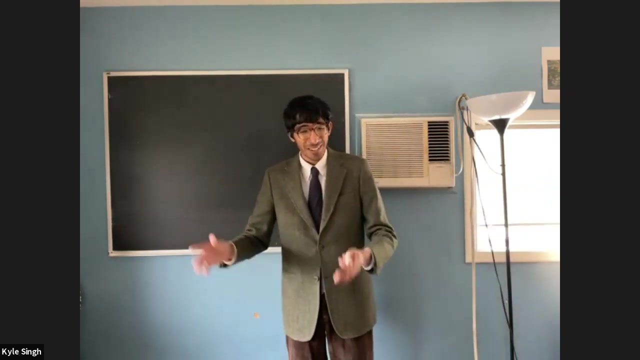 Schwinger taught at Harvard for many, many years and he had many graduate students that wanted to work with him and he had a line of 20 graduate students. this is the story, and Schwinger was going down the line and giving each graduate student an idea. can you imagine? for a thesis? 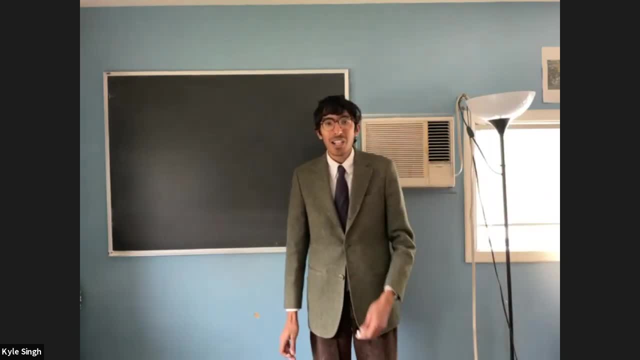 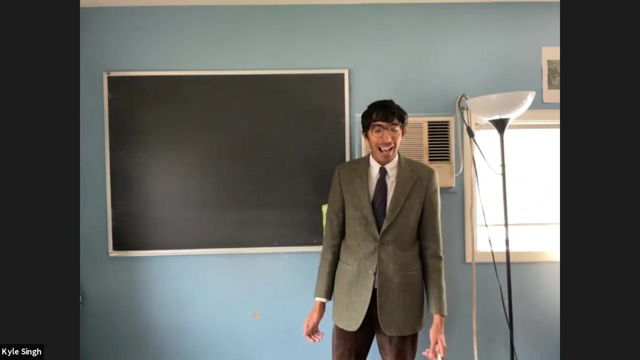 right there on the spot and he gets to Glashow and he goes- Glashow was the last one- and he goes. I want to look and see if there's a way to unify the electromagnetic forces under the weak interaction. amazing, he just said it in one sentence. I mean he had that much intuition and it's what propelled. 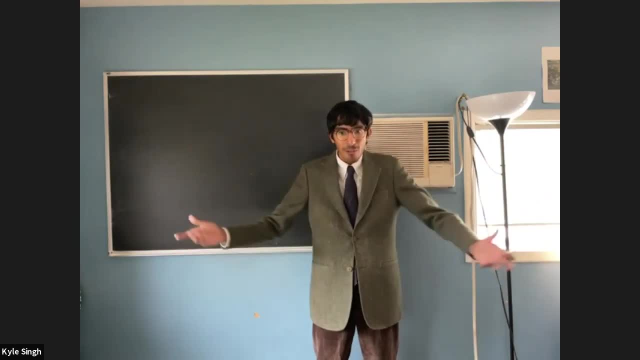 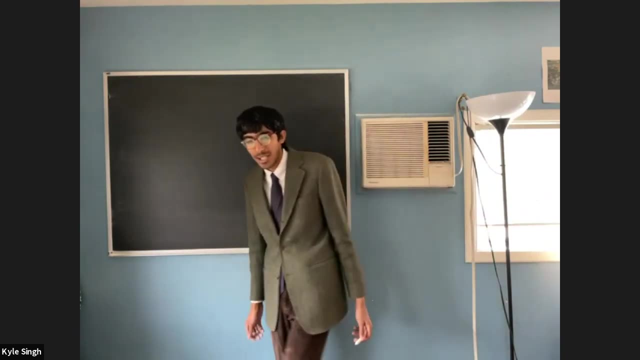 his career, what he worked on for 20 years when he won the Nobel Prize. on all of that- and it was very interesting hearing that from him- he said it wasn't my idea, it was Schroemer's idea. very interesting, just goes to show you these guys had many, many and and then you look at the Gelman-Feinman paper. 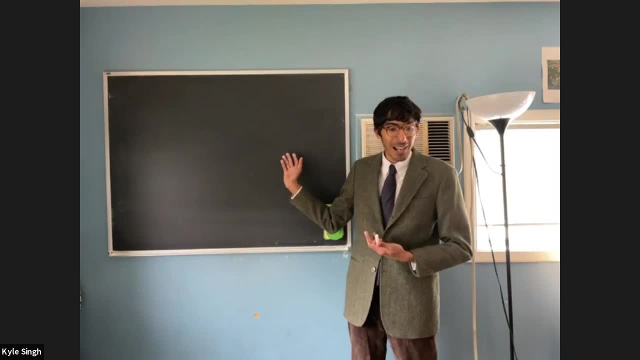 People just take it as a topic. these guys had many, many and. and then you look at the Gelman-Feinman paper. people just think Feynman retired after QED. no, he made a lot of contributions. you know, the public doesn't know about this, and Gelman made a ton of them too. so it's just interesting to to think. 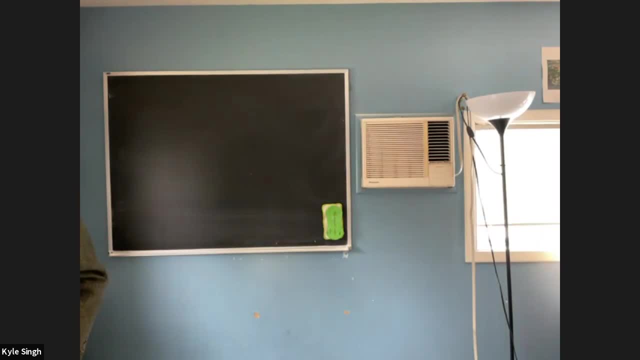 about that sometimes. okay, great, so he publishes this in 1961. in 1967, Steven Weinberg and Abduh Salam come through and they say that actually Sheldon Glashow's electroweak unification scheme is actually a spontaneously broken gauge theory. 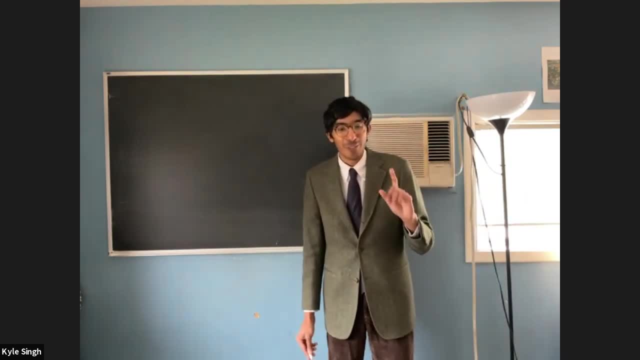 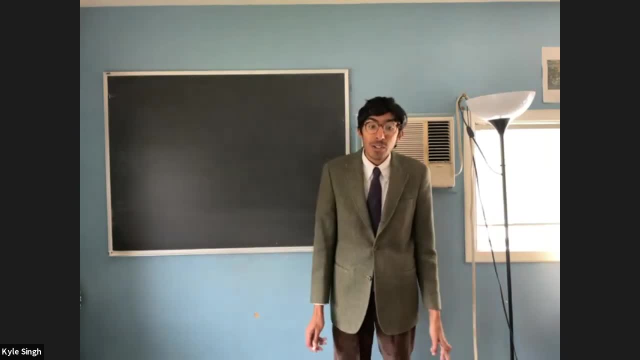 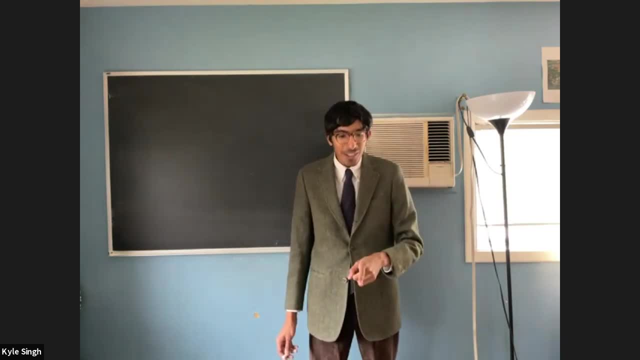 story: Steven Weinberg and Sheldon Glashow- same high school, Mansoor's high school, and they both wanted to go to the same PhD program. but Weinberg went to Princeton, got into Princeton, got rejected from Harvard and Glashow got rejected from Princeton, got into Harvard. so they flipped one. 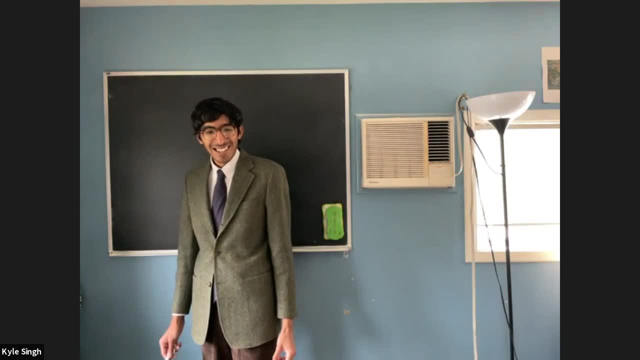 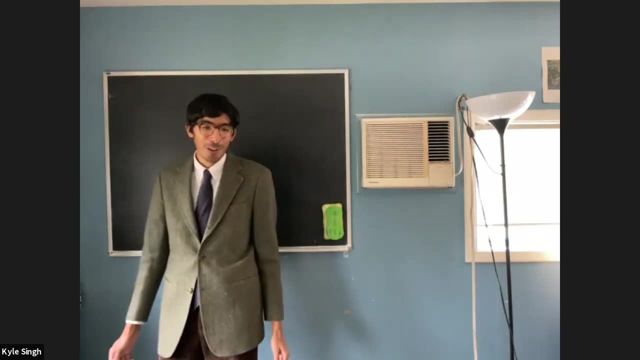 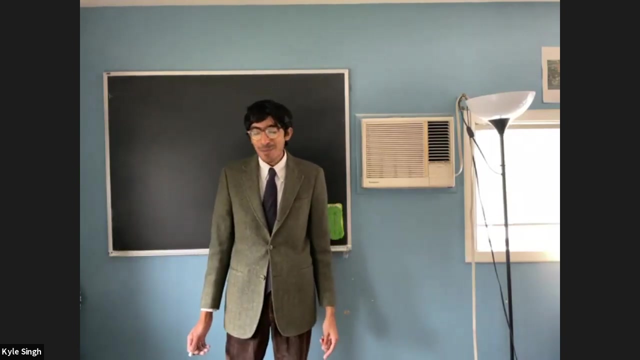 I'm pretty sure when you walk in there's like a poster with them on it. I'm sure, I'm sure I mean they're titans, they're like two of the greats. so that's really cool that they were both in the same year. can you imagine the kinds of conversations they were having? uh, it's pretty cool, it's pretty. 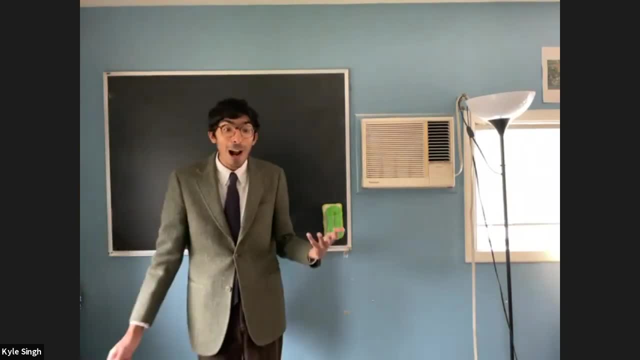 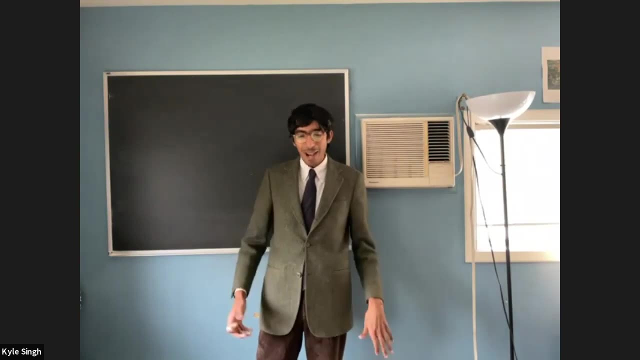 wild and both won the Nobel Prize in the same year. can you imagine that two high school buddies winning the Nobel Prize in the same year for the same? I mean it's just. it's just an unbelievable too bad. the public doesn't. if you ask the public, who is Steven? 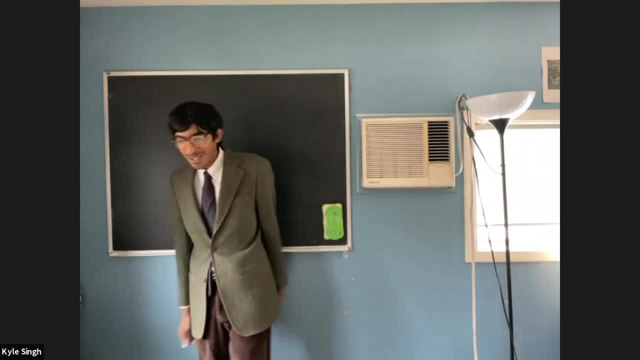 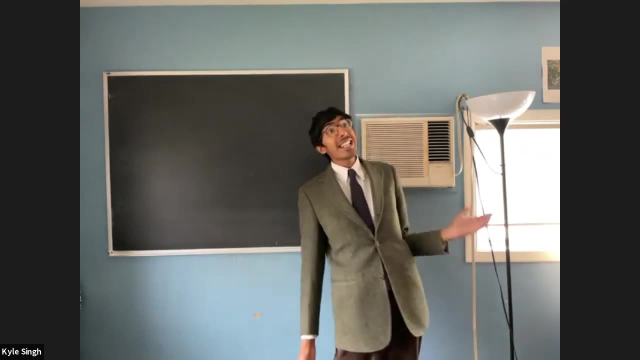 Weinberg or Sheldon, they don't even know. so that's the thing you have: to promote this, okay, anyway. so that happens in 1967. and then in 1971 we had another wunderkind, Herarty Hooft, who proved that the theory was renormalizable. and not only that theory. 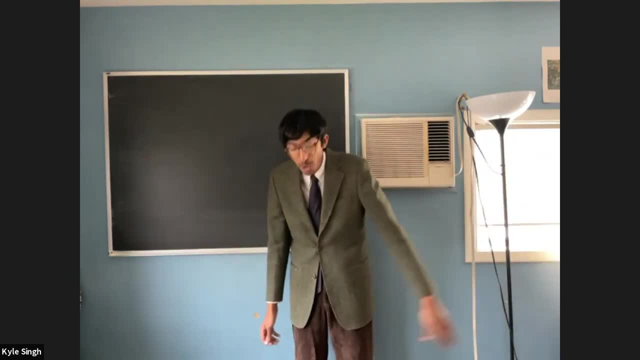 but all non-nobelian gauge theories, for which he also won the Nobel Prize in 1999. so this was a very like I'm just giving. this was an extremely exciting time from the 1940s to the 1980s in theoretical physics, that 40-year stretch extremely exciting. from 1940 to 1980, tons of developments. 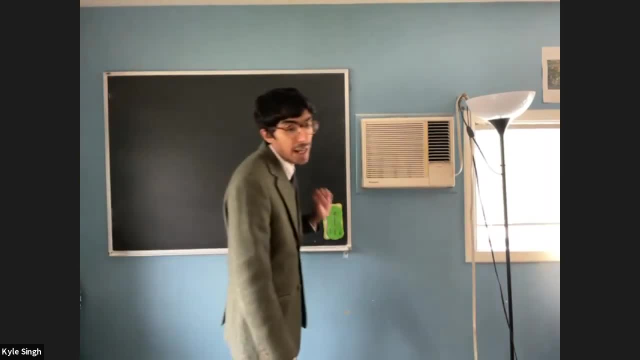 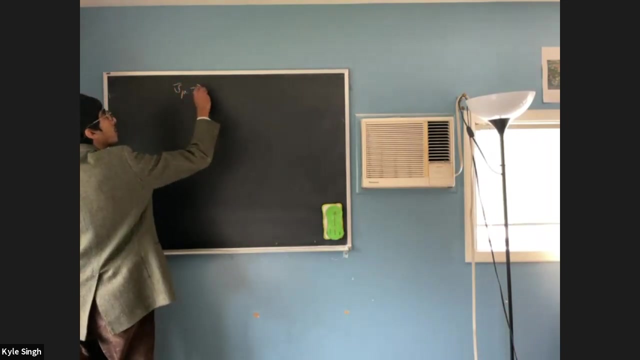 okay, anyways. but no experiment until 1973 at CERN, which was the November revolution. okay, anyways. so let's now look at neutral interactions. okay, which are a little different. so let's have an anti-muon neutrino go to an electron- oh, what am I writing down? plus an electron. 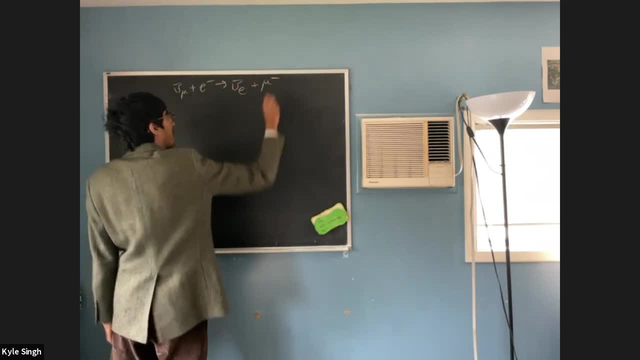 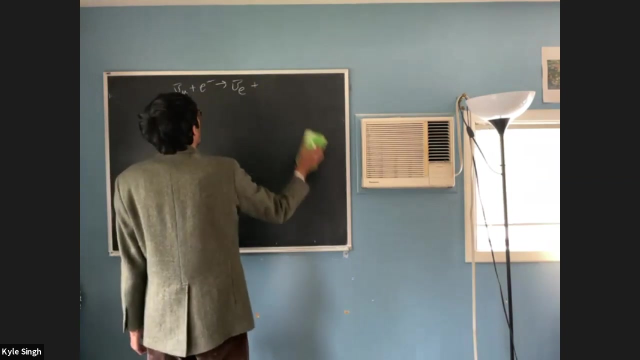 going to an anti-electron neutrino plus a muon. you? oh no, sorry, sorry, sorry. this is a neutral interaction plus an electric. no, no, no muon neutrino plus an electron. so in the neutral interactions they can actually give off a different neutrino, but it doesn't. it doesn't make a difference. 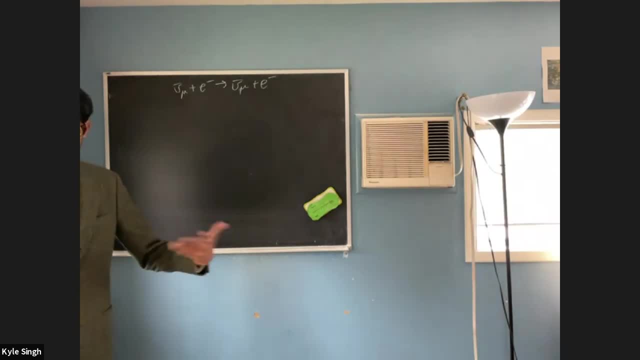 in your calculation. you don't need that extra factor because of the fact that the, the median and particles different. sorry, okay, let's draw the fine. fine, do I have to draw the Feynman diagram? all right, I'll draw the fine. fine, I'll draw the Feynman diagram for you guys. 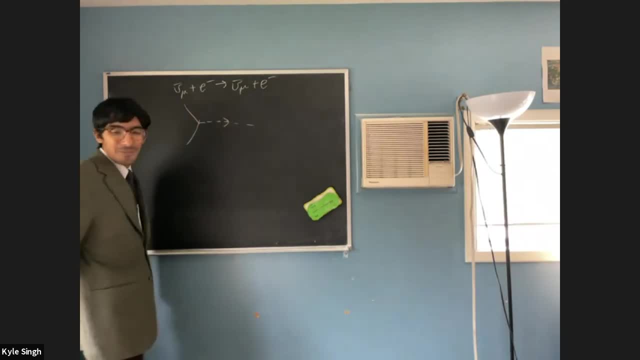 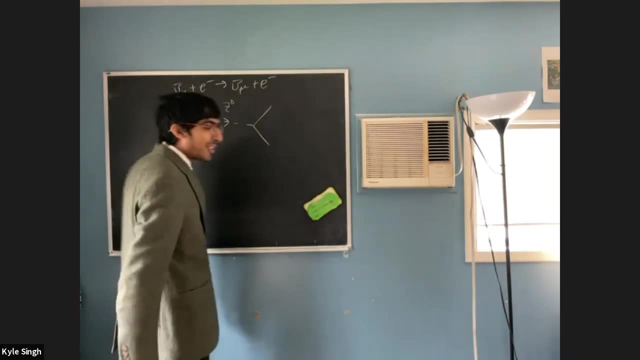 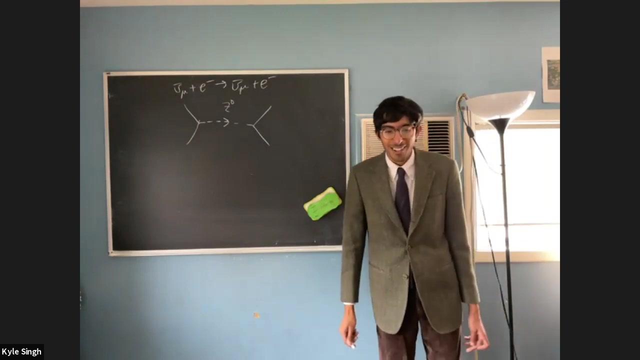 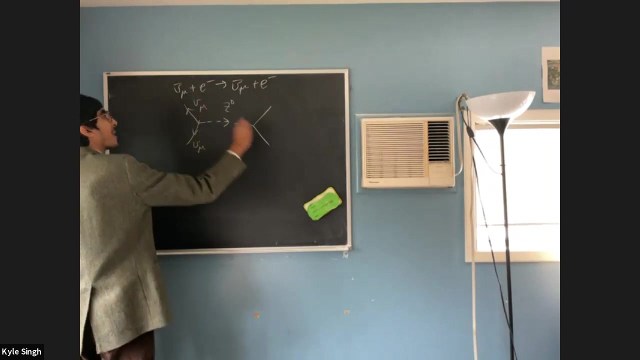 uh, there was a very old quantum field theorist that made a joke. he said: I'm a professor of Feynman diagrams. uh, that's not really. that's probably not accurate. okay, that is not accurate, sorry. okay. so this one's going out, this one, this one's going in. this one's going out. 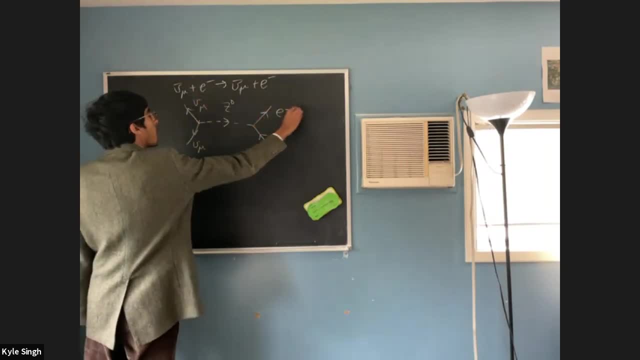 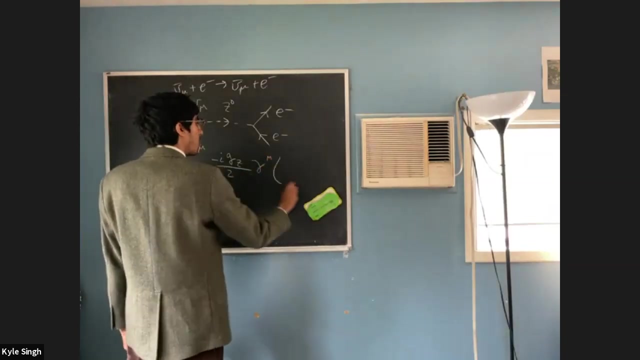 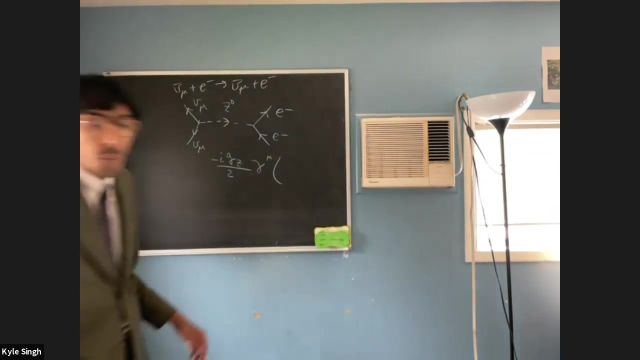 this electron's going in, this electron's going out, and now the vertex factor is now minus. I will call this gz from the coupling to the zebo zone, which is neutral over two times gamma mu. and now we get some weird mess here, by the way, oh, I forgot in that 1961 paper. 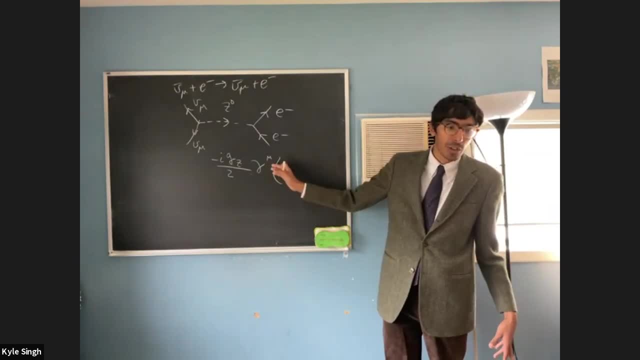 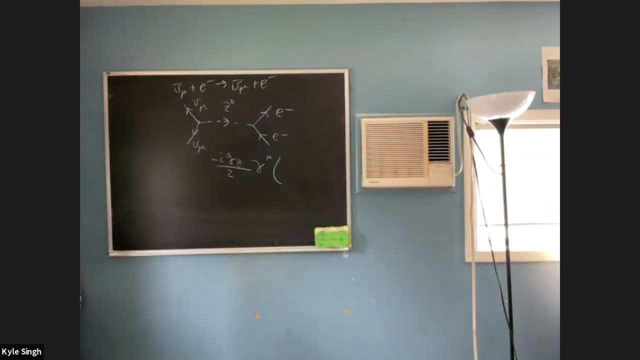 Glashow postulated that you must have neutral interactions, so that was a prediction that was made. okay, we'll call this c v f. I'll tell you what these are. c v- what the heck? what do I want to call this? if I call that c v f? 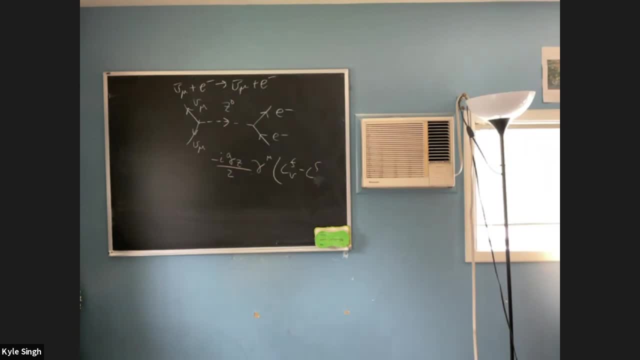 okay, we'll call this c a f. I'll tell you what that means in a second. some factors times gamma, phi. so these two guys depend on the quark and the lepton and quark involved and they're they're constants that are going to depend on what particles you put in. 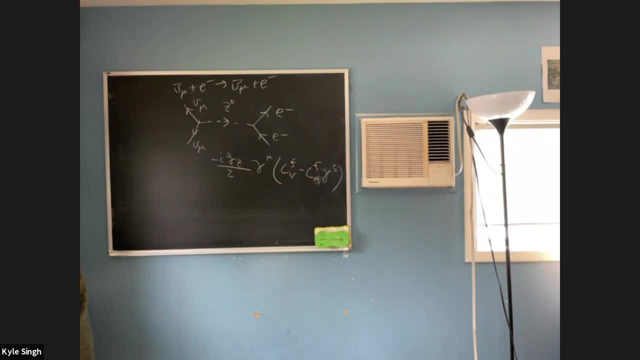 but that's how the vertex factor differs. uh, let's not, let's not worry about that, really, okay, but uh, you get some, some factors. all right, can I erase this? for we're going to see where these come from, but it's going to take us a little bit. 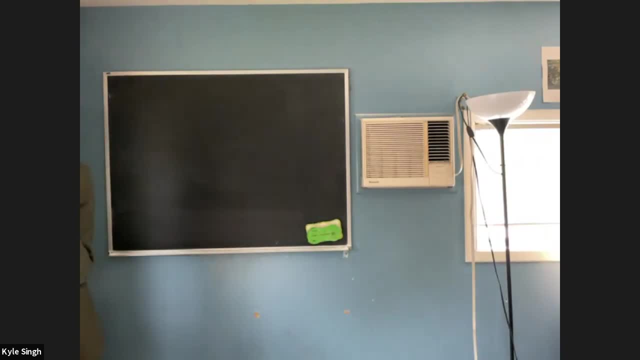 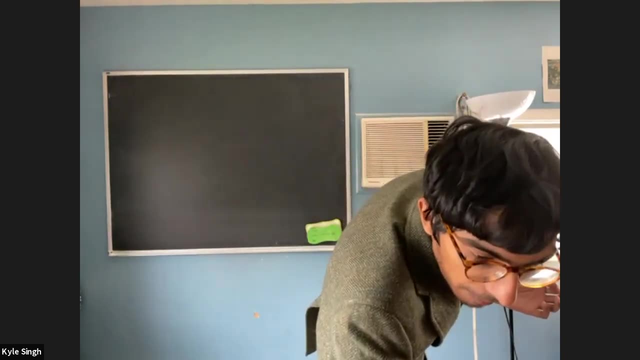 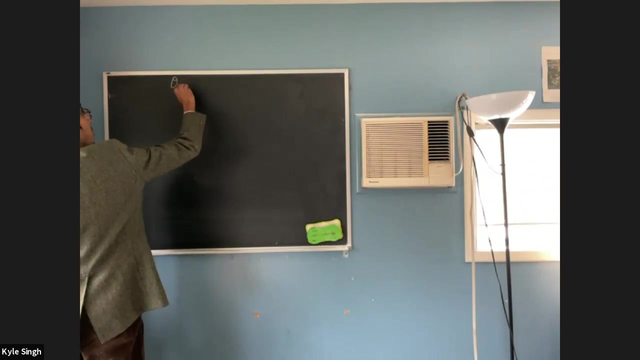 okay, so in the Glashow, Salam and Weinberg model, all of the numbers or all of the parameters that the theory depends on depends on one uh sort of angle. you can call it an- it's not really an angle- theta w. you can derive everything from this one number and this is called the Weinberg angle or the weak mixing angle. 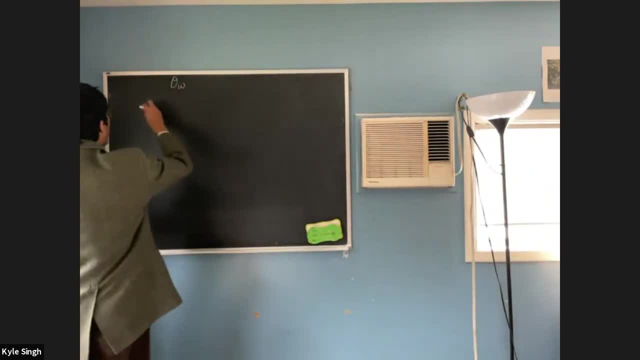 so you have the relationship now between the coupling for the w and z boson to the electric charge. so g w equals g e. over sine theta Weinberg, this stuff's not going to make any sense until next week, because we're going to derive a little bit from: 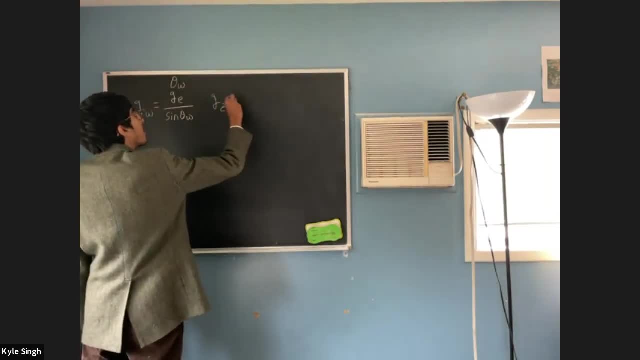 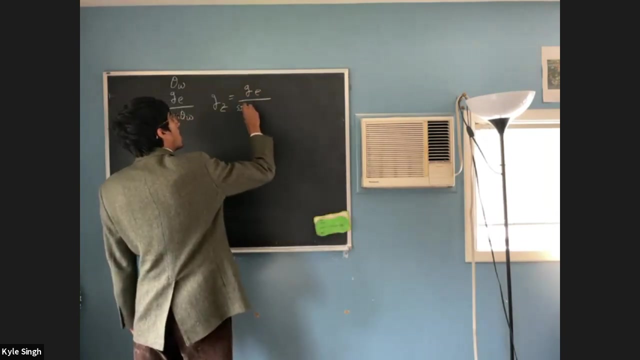 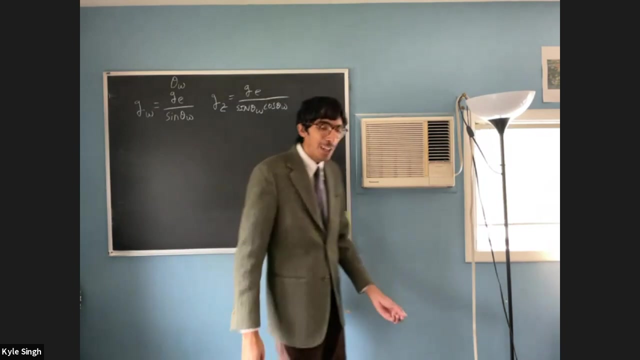 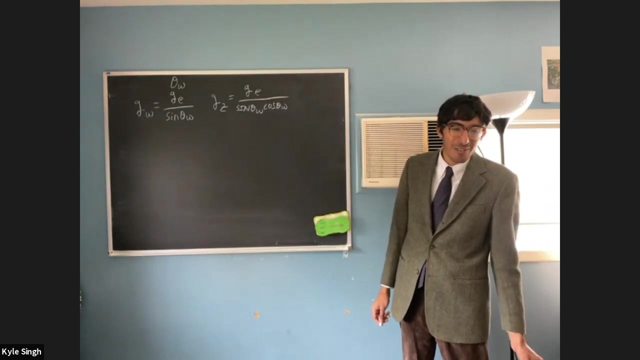 the electroweak unification. then you have this relationship: g z equals g z over cosine theta. sorry, sine theta, cosine theta. okay, so you have electroweak unification by this parameter, theta w. where does it come from? you'll find out when I show you electroweak unification what the model actually looks like. 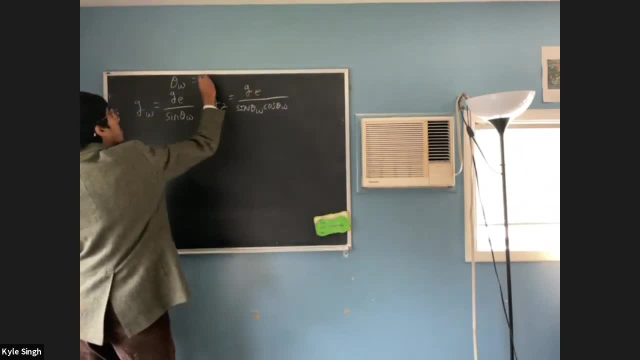 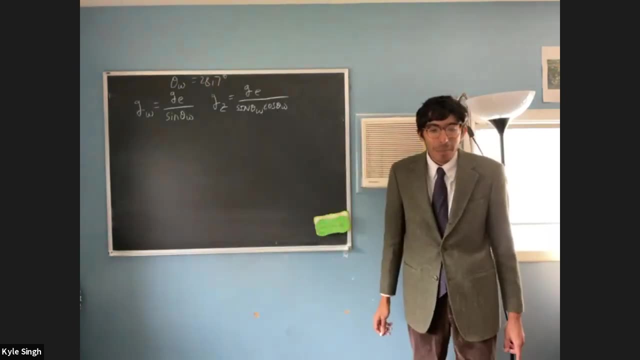 turns out experimentally that this Weinberg angle is equal to 28.7 degrees. why is it that number? nobody knows. this is a big challenge actually for people. you see, the standard model has a lot of parameters. you probably are starting to recognize it, like when you, when you see the standard model on 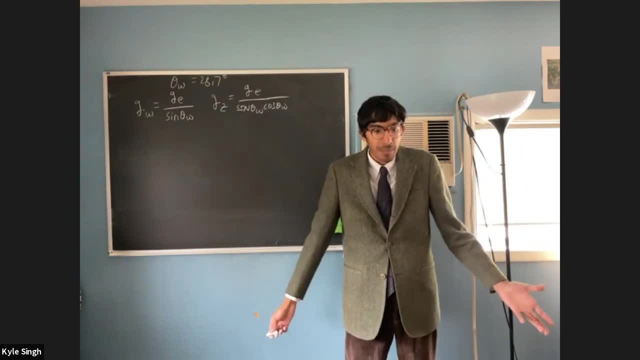 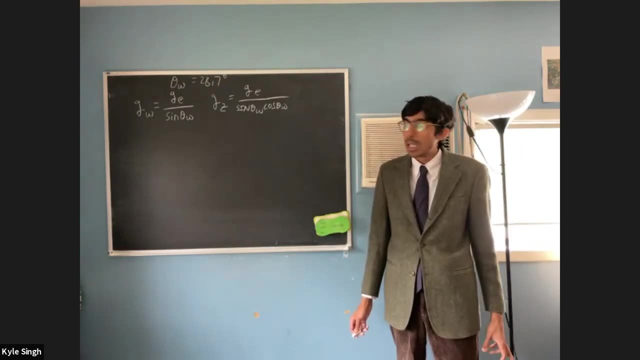 someone's t-shirt. there's tons of parameters that are random, seemingly, and one of the big challenges of people who try to come up with so-called grand unified theories, uh, is to derive these parameters. right, in principle, a grand unified theory should be able to derive these parameters. no one has been able to derive this Weinberg angle. it's a big challenge, uh. 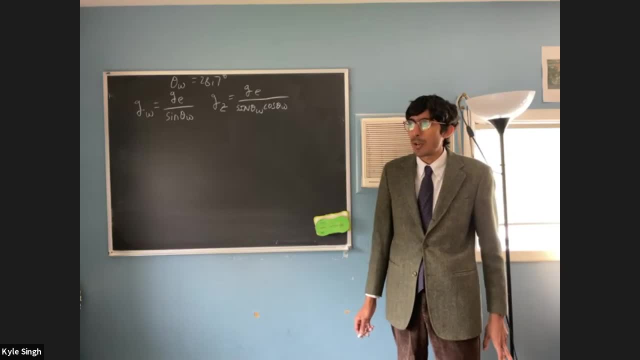 yeah, one of the earliest examples of a grand unified. there was also actually Sheldon Glashow with a guy named Howard Georgi, which was an su5 grand unified theory, and even they couldn't derive this. so it's very interesting actually. okay, let's write down a few more relations. 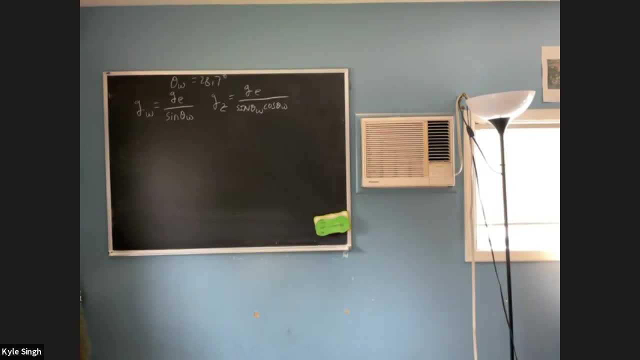 shits. so the the z propagator then is just, we'll just write it down: minus i g nu nu over q nu, q nu. that's just the z propagator over m z squared, which should be oops down, should be a minus. okay, all over q squared, minus m z squared. and right, we work in that limit, so we get minus i. 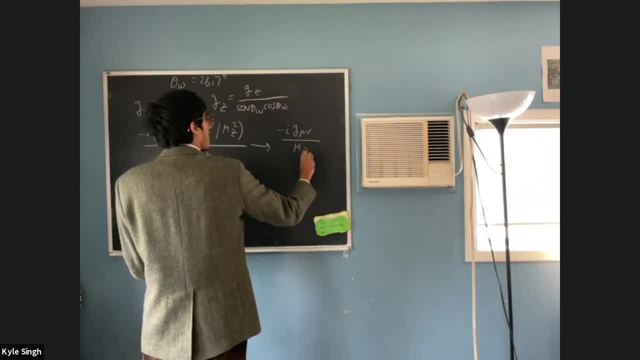 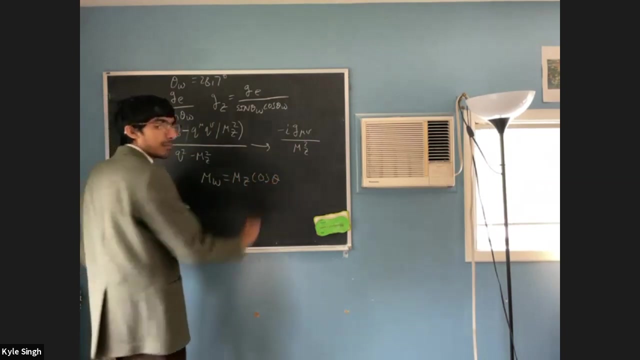 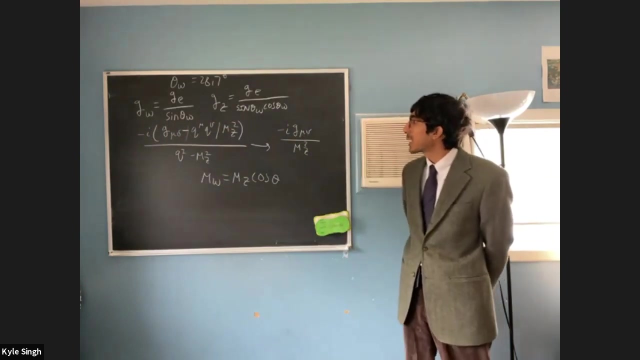 g nu nu over m z squared. okay, and the relationship between the w and z masses is that m w equals m z, cosine theta. that's the relationship between the masses. okay, so these are actually the basic predictions from the unified model gsw. right, this prediction, this should be theta. 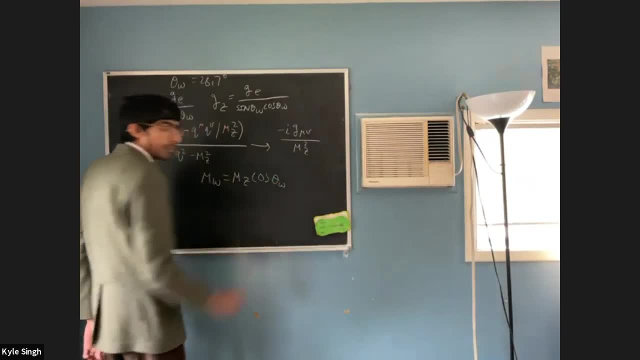 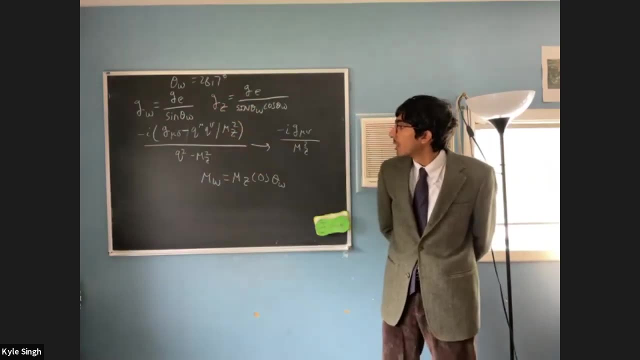 delta, this prediction, these two relationships and this weinberg angle and you can derive all of the relationships of the weak interactions from the gsw model. okay, that's all i have for today. i hope today was relatively simple. we just did some kind of straightforward calculation. i didn't really show. 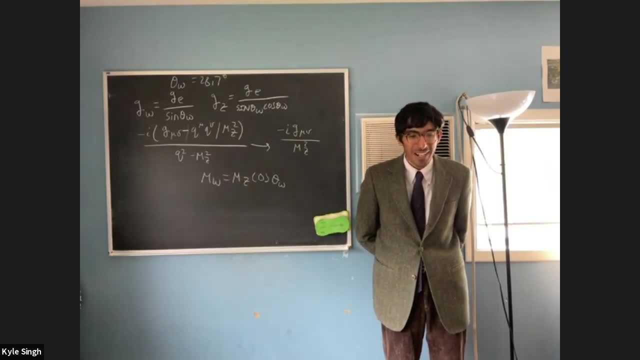 you next week's going to be difficult, i give. i'm giving you fair warning. so if you do some reading, that will help you a lot. and please, please, review spontaneous symmetry, raking uh, or the lecture i gave on it, because that will be important. let me just stop recording.